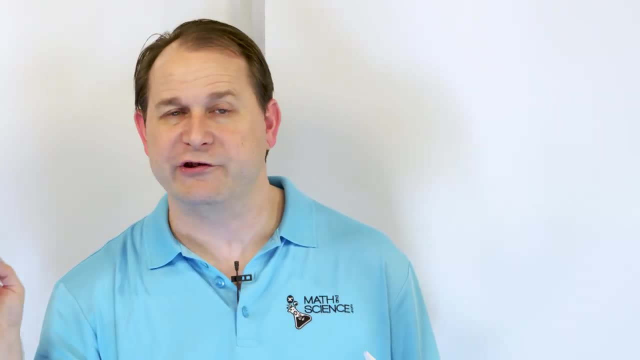 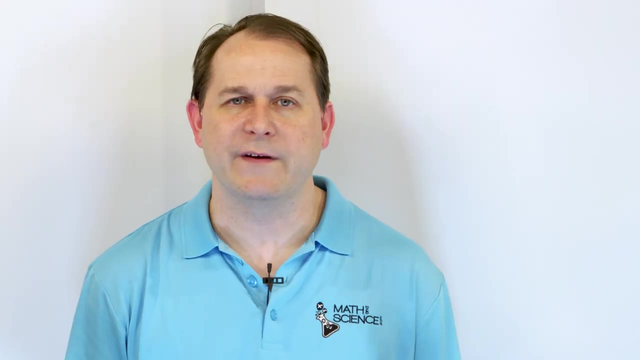 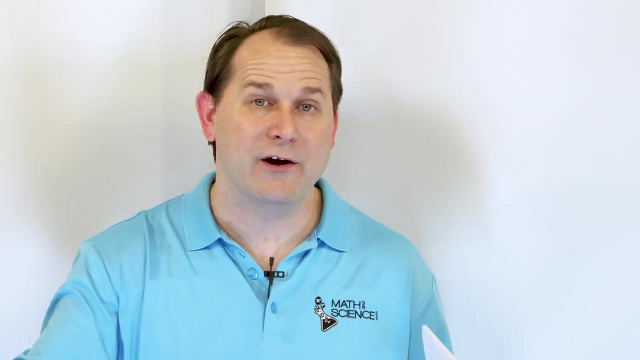 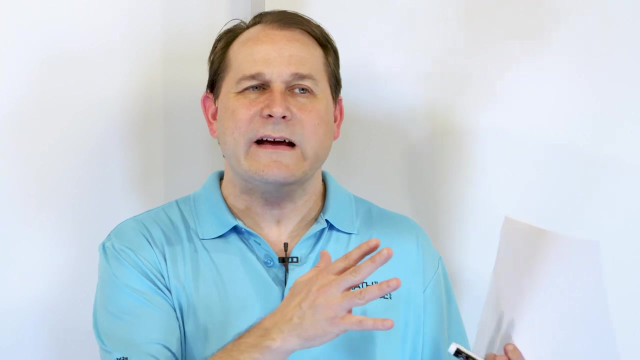 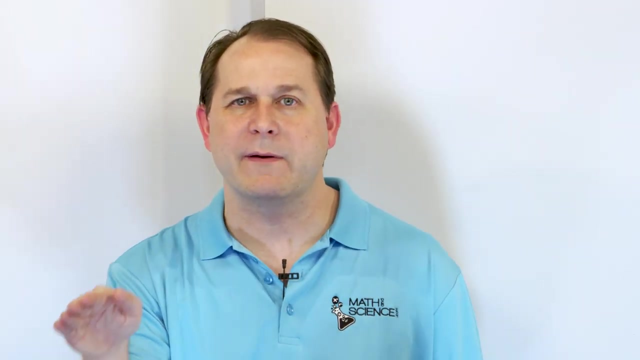 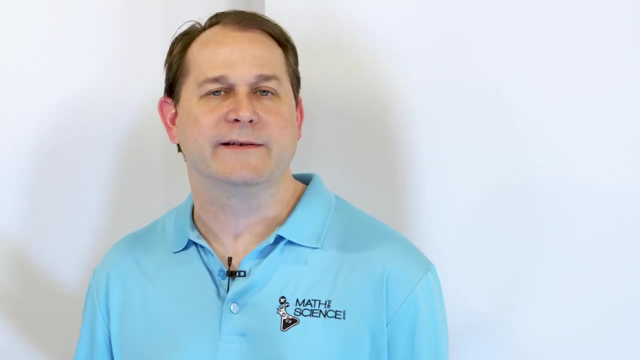 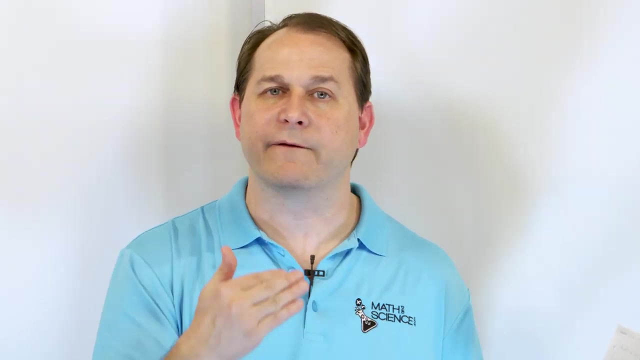 comes back down, that is the shape of a parabola. When you actually go into physics and you study motion and how things move in gravity, it traces out the shape of a parabola. Another example from physics, when you learn about energy, kinetic energy, it's called one half m is the mass of the object, one half mv squared. So anytime you have that square term, it's a parabola kind of shape. In that case, it's energy and velocity. But anyway, these parabolas pop up all over the place. So we're going to spend a lot of time talking about more detail, why is that shape of a parabola so special? Why do we care? Why is it so important? So we're in the beginning, we're going to review what we already know about parabolas. Then I'm going to give you kind of the basic overview of the equations of parabola in terms of other things we're going to learn called the directories and the directorics and the focus of the parabola. 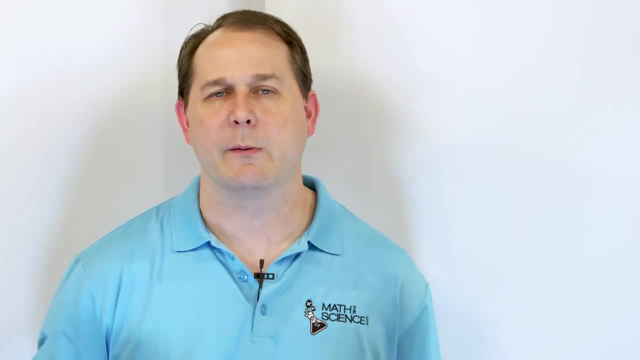 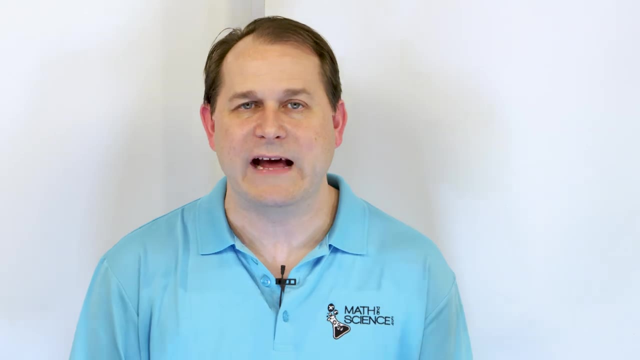 And then we're going to go through some derivations. I'm going to show you where that shape comes from. If I had to boil down this section into one sentence, it would be why is the shape of a parabola so special? And what is that shape? How do we know that it's a parabola? 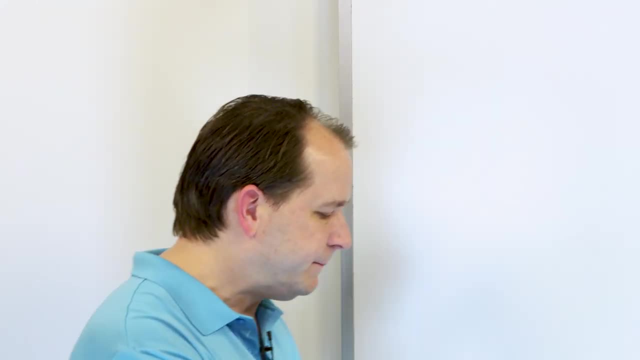 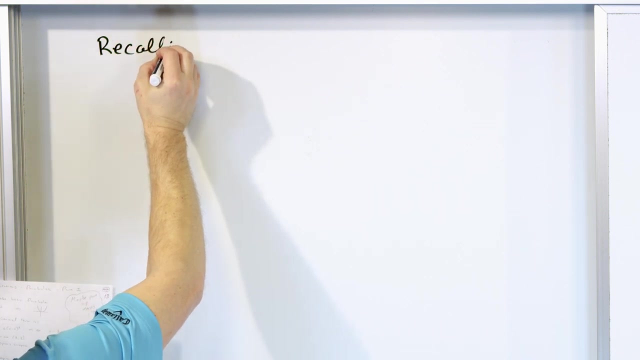 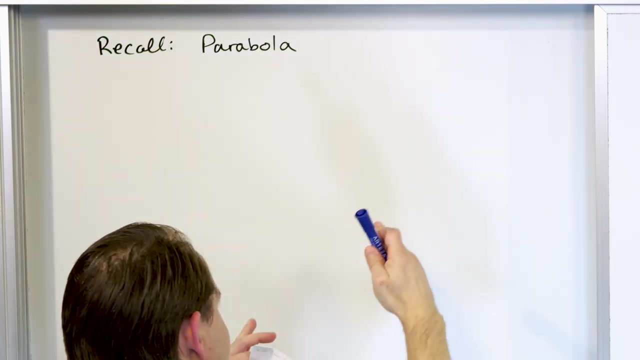 How do we find out what that special shape is? All right, so let's get started. We want to talk about, we want to recall the basic shape of a parabola. We have done this before, but now we are going one or two levels deeper into the concept of a parabola. So we're going to review really quickly what we know. We know the simplest parabola that we can have 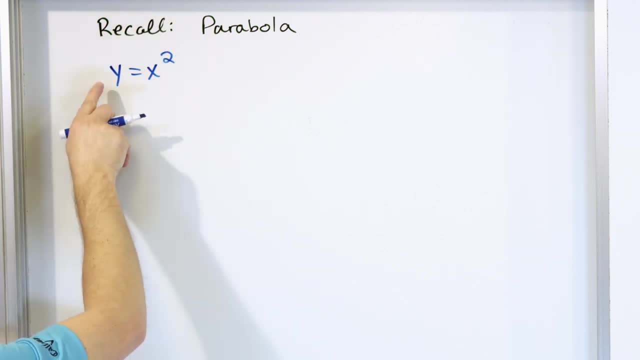 is y is equal to x squared, or you could replace the y with f of x, the function f of x is equal to x squared. 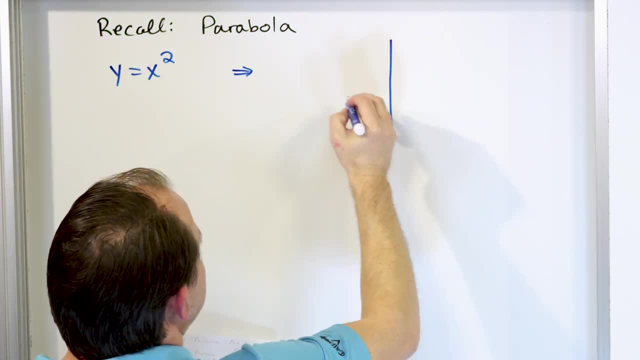 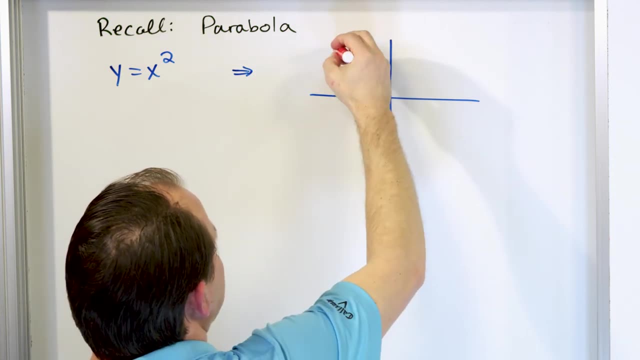 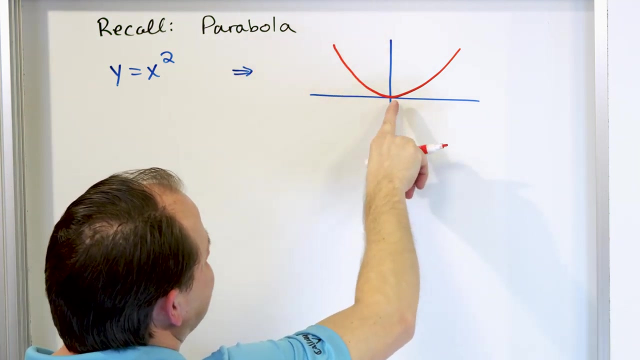 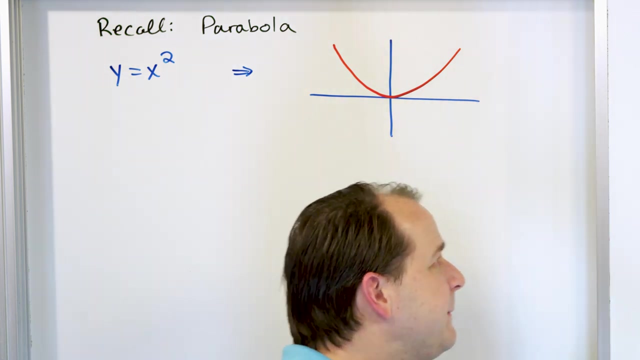 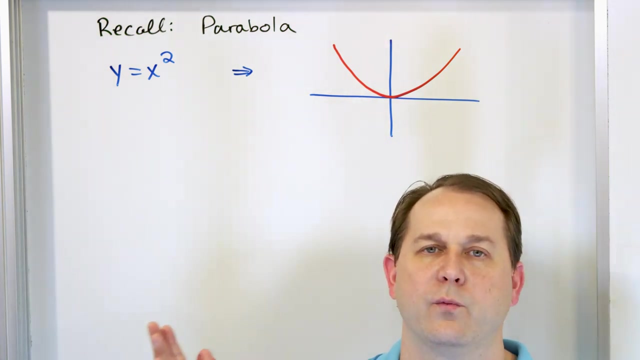 Right? And this parabola is the simplest one that we can have. I'm going to draw a very small little graph here, nothing too big here. But if we wanted to draw the basic shape of a parabola, we know this parabola touches the x-axis. It goes down something like this and goes up something like this. It's kind of a smiley face. Notice now this is not a perfect drawing. It's got a little kink here in the bottom. You got to imagine a smooth drawing there. The shape of a parabola is not a semicircle. A semicircle would be something that would go more down like this and more straight up. This is much more a gradual opening is what a parabola is. Now, of course, that's the basic parabola. But you know we can change the shape of that parabola, make it close up narrow or open up wider. 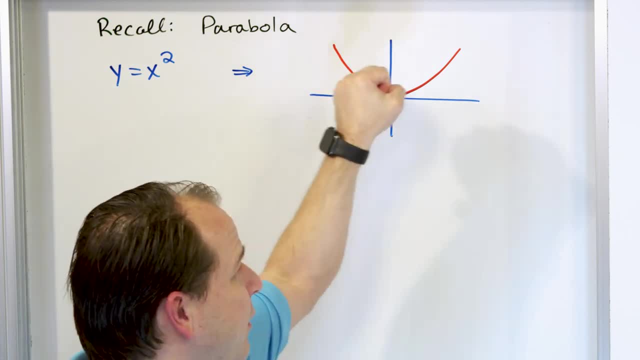 We can flip it upside down so it opens up down. And we can also take this parabola and we can move it anywhere we want in the xy plane just by changing the equation of the parabola. 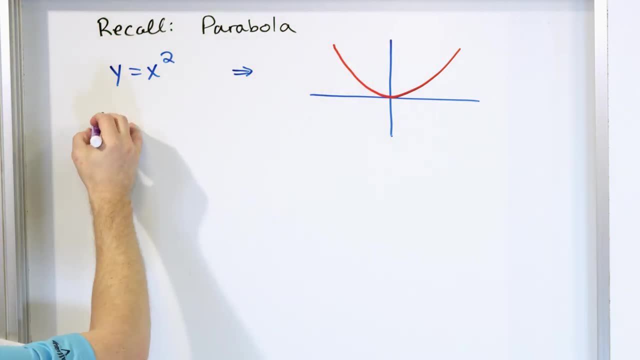 So we learned in the past that the more general form, the general form of the parabola is something like this. It's y minus k is equal to a x minus h quantity squared. Now, if this looks unfamiliar to you or totally you're lost already and you've never seen it before, then it just means you need to go back to my lessons on parabolas. We talked about that at great length. I did probably 10 lessons on it. We talked about what every little part of that equation means, how to sketch parabolas and all of that. But we never talked about why the shape of it is so special and why it's so important and what the shape of a parabola really is. We learned how to sketch it. 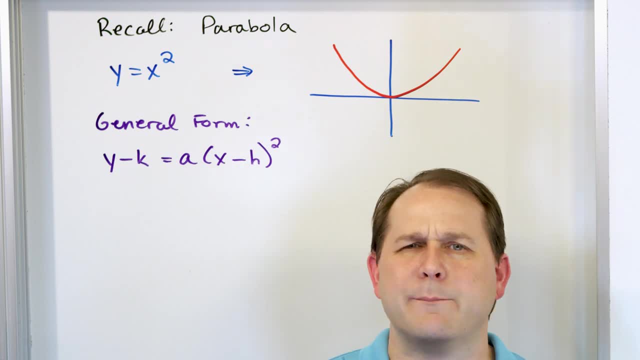 We talked about why geometrically it works or why it pops up in nature so much and what's so special about it. 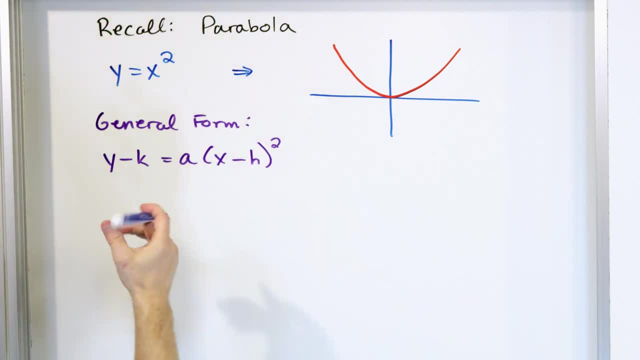 So this is the general form. And an example of that for an example of a practical parabola in this form would be something like this. Just one example off the top of my head. Y minus 3 is equal to 2 times x minus 1 quantity squared. So notice you do have this x minus 1, but this x term in general is squared. That means it's a parabola. The 3 and the 1 tell you that this parabola is shifted in the xy plane. And the 2 in front of the parentheses tells you that it's actually closed up on itself a little more than this one right here. 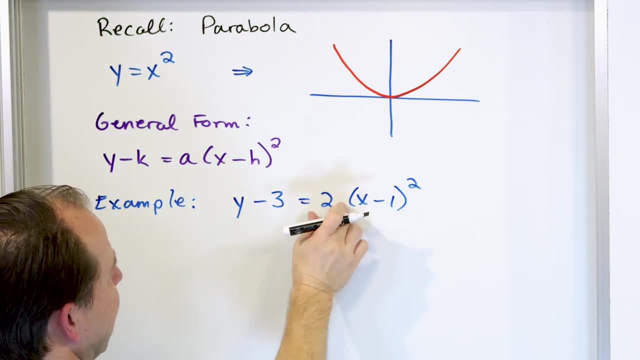 So if I were going to, and also because this is a positive number out in front, the parabola 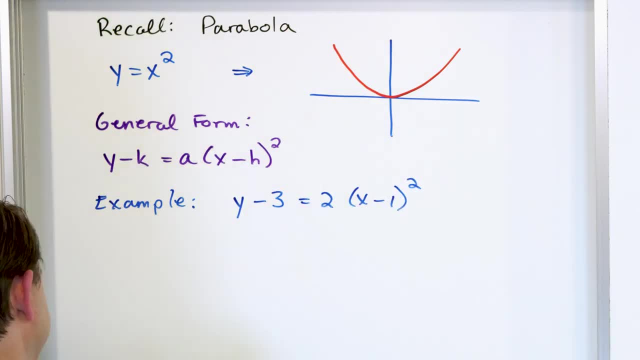 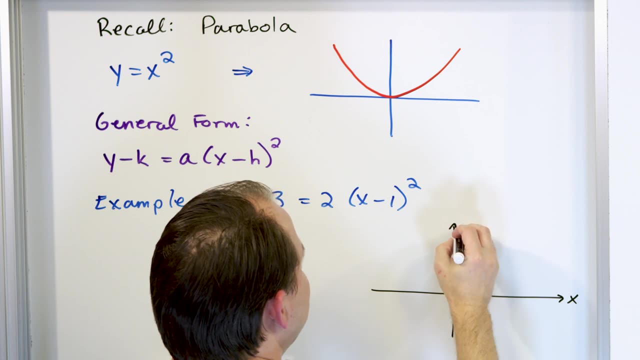 opens up. If it were a negative 2, it would open down like a frowny face. So the general idea or the general shape of this parabola, this is not going to be a detailed graph, but just this is all review. 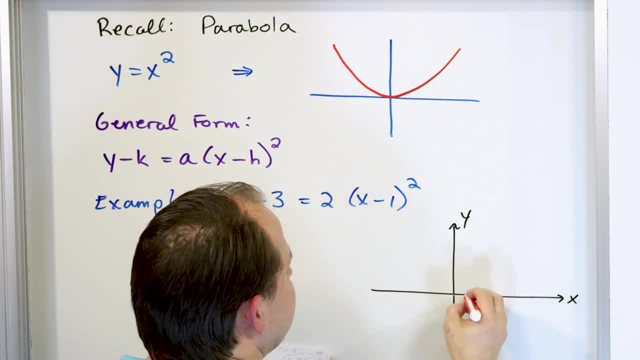 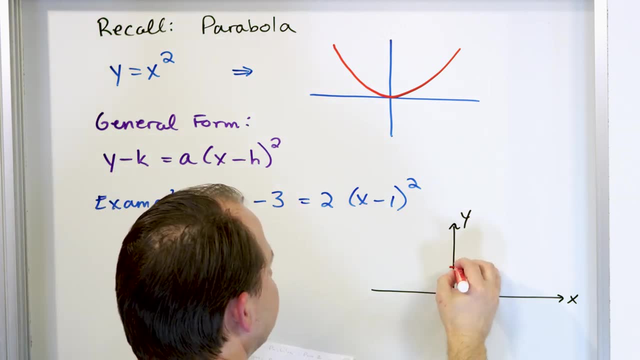 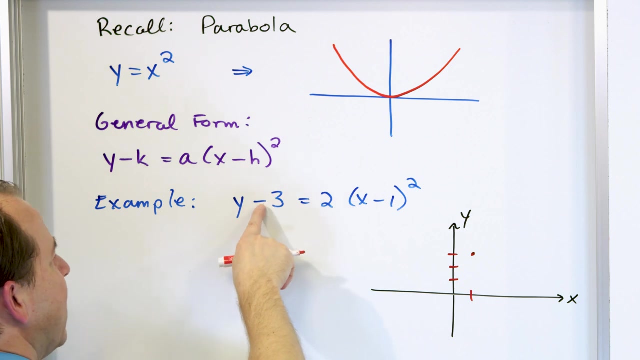 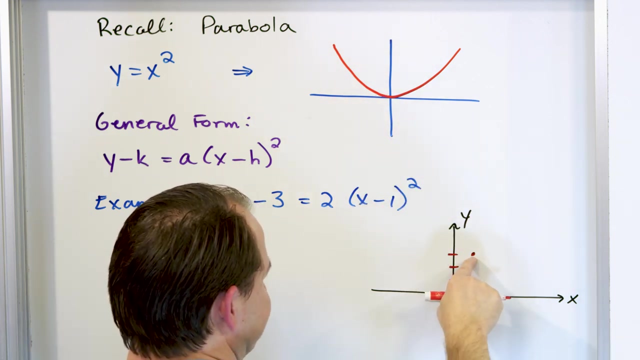 This is stuff we've done before. The x coordinate is shifted one tick mark over in the positive 1 direction and then in the positive 3 here and for y, 1, 2, 3. So that means the bottom of this parabola is at x is equal to 1, y is equal to 3. We talked a long time ago about these minus signs and why it shifts it in the positive direction. So we know that the vertex, the bottom of the parabola is now here. And this parabola has a positive 2. 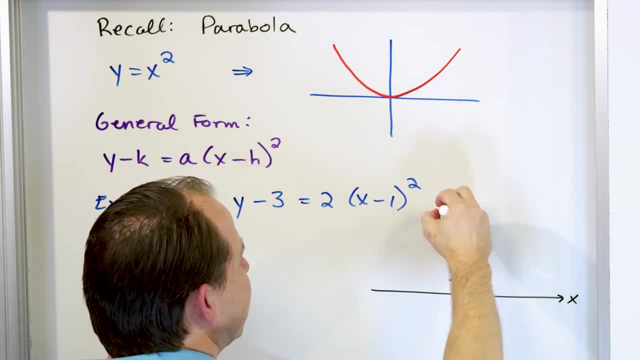 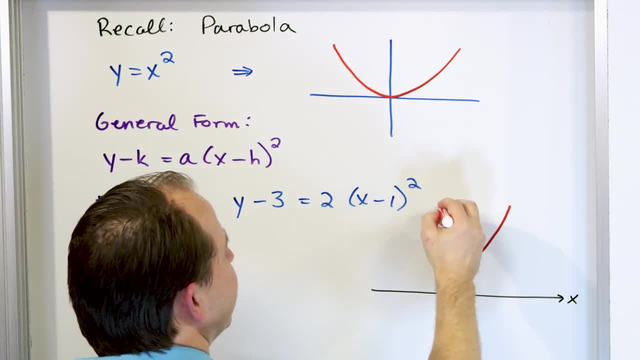 I'm just going to guess here. This is probably going to open up a little bit more steeply. So you see, the higher the number in the front of the parentheses closes the thing up more. 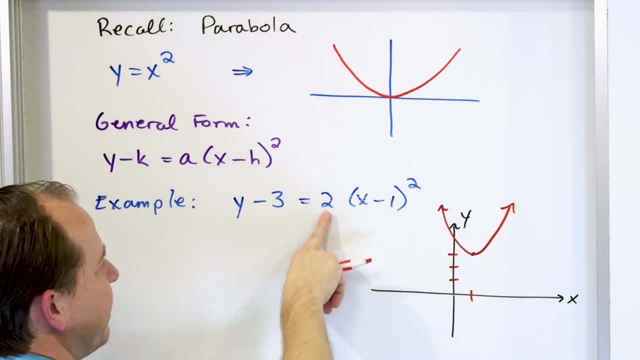 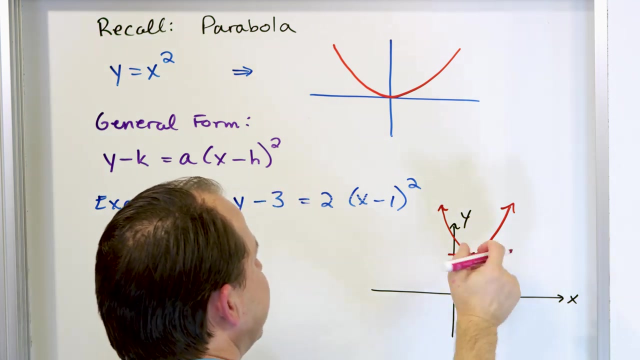 If you had 10 or 20 up here, it would be really, really narrow. And of course, if it were negative, the whole thing would flip upside down and go like a frowny face, like this. So when this number in front is positive, it opens up. When this number in front is negative, it opens down. Everything that we have just discussed, including the vertex, 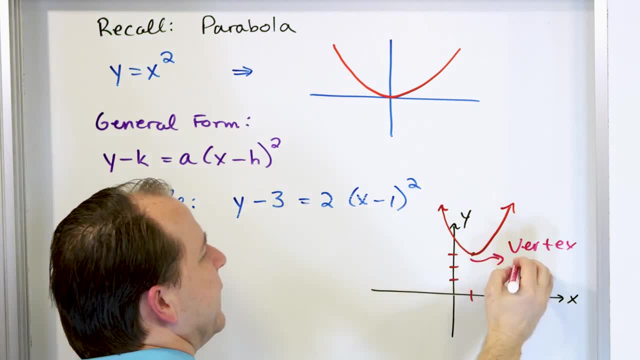 vertex, notice you can read the vertex directly out of the equation, is 1,3. Everything, 1,3. 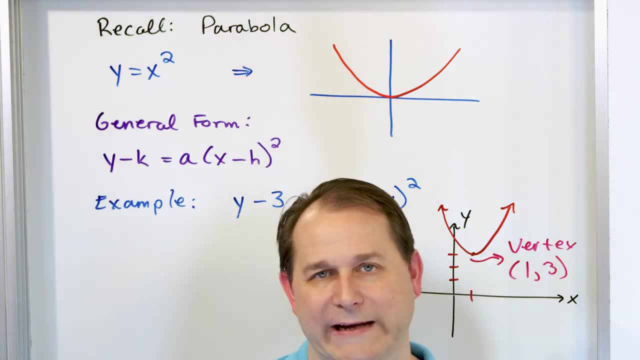 Everything that I've just talked about, we've covered at great length already. If you don't have any idea what I'm talking about already, then please go back to those lessons on parabolas. 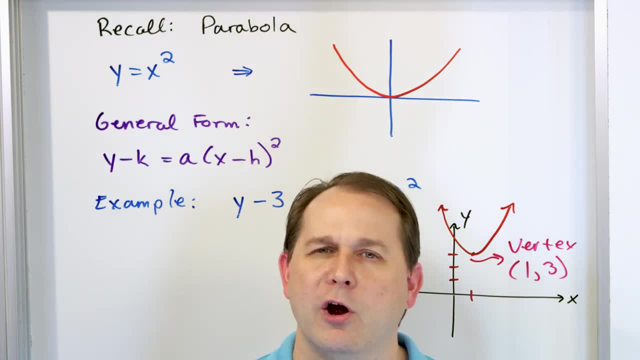 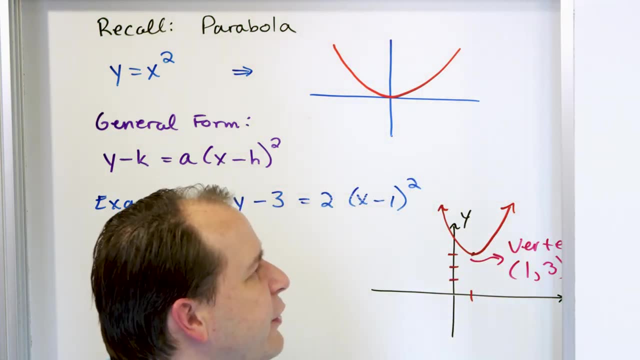 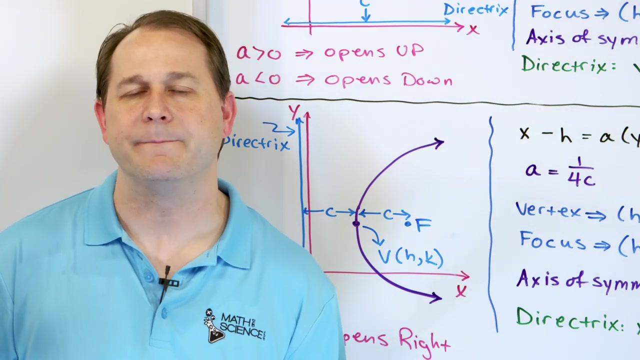 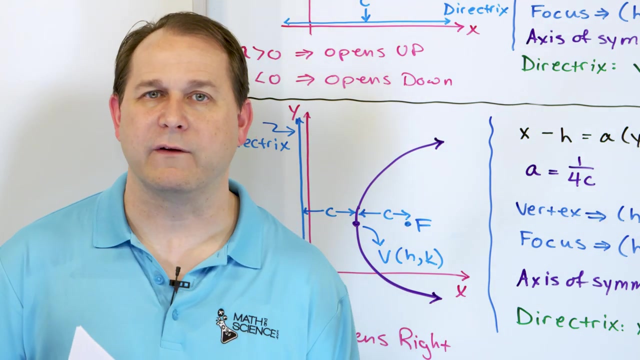 Our goal now is to go a little deeper. That's what we know so far, but we want to go a little bit deeper. And so to do that, I have a bunch of things that I have to cover kind of in sequence. And the first thing I want to do is I want to give you a taste. We're going to revisit this board. I almost never ever just put things on the board and have you read them. I don't like doing that. But in this case, I have to because there's so much information I have to get across. So I have to make sure it's all done correctly, right? So here we have the general equations of a 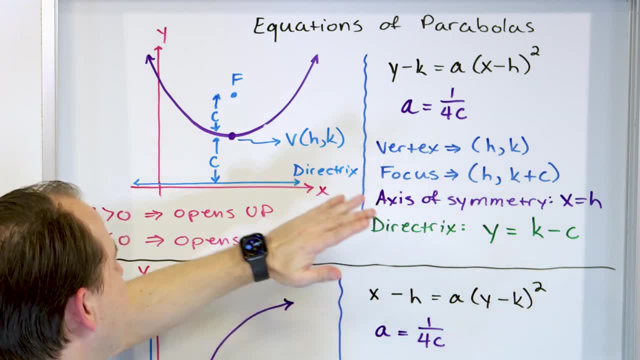 parabola. I want you to ignore everything on the bottom side here right now and just focus on the top. Basically, this is the general form of a parabola equation. This purple curve is a parabola. 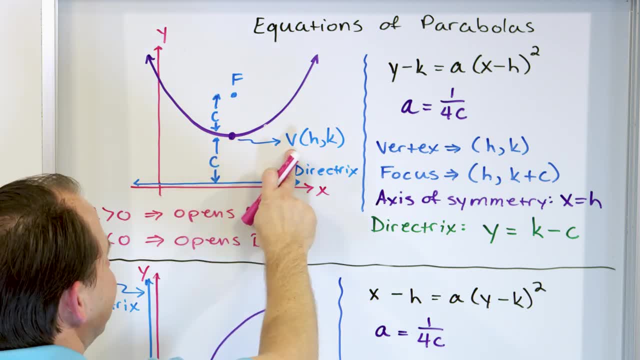 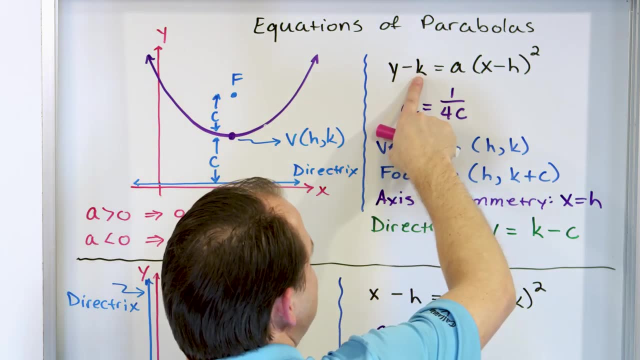 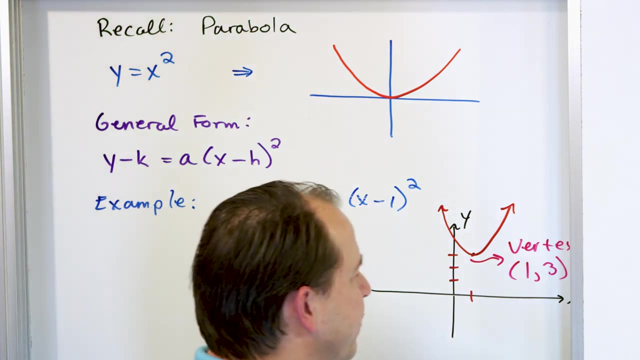 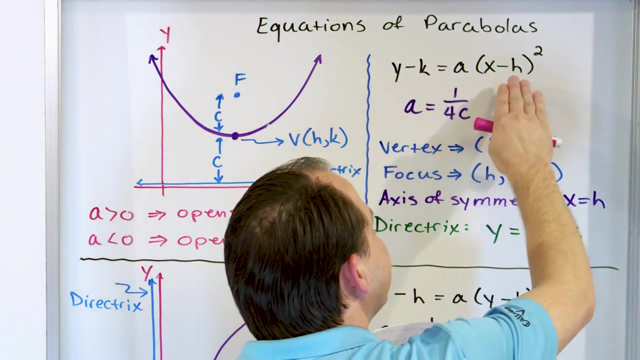 Right? The vertex is the lowest point right here. That's why it has a v. And the v is at h, k, which is exactly, this is the same form of the equation we wrote on the other board. So we had y minus k and x minus h. y minus k, x minus h. This is exactly what I've written on the previous board. So this is all stuff we've learned. But I guess I just want to put it all in one place and tell you this is the general form of the equation. This whole relation between a and 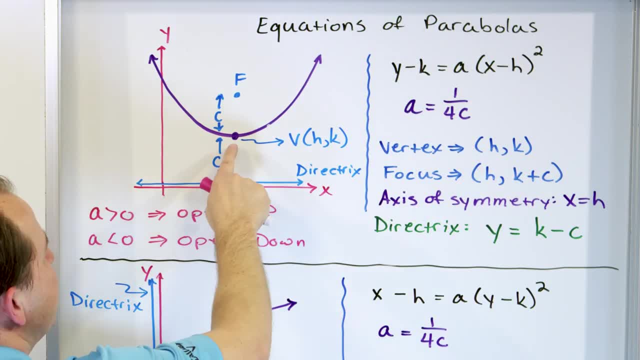 c, I'm going to come back to a little bit later. Because this is the general form of the equation. Because notice, when you get over here on the graph, you're going to notice there's a couple of additional things that we never learned about in the past. We do have the parabola. But now we have a special point above the parabola called the focus. We're going to talk about the focus of the parabola in just a minute. So you can think of the beams of light, if you want to think of them 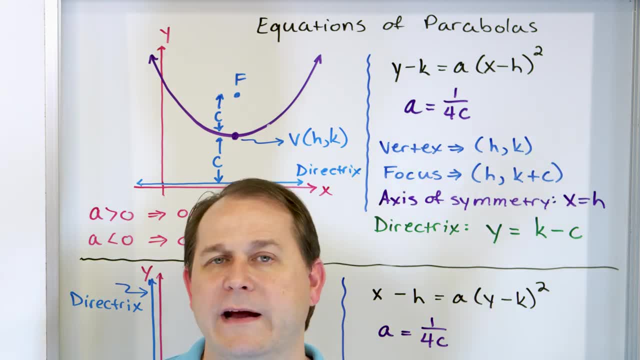 as reflected from that parabola, are focused at a point. That's why it's called the focus. 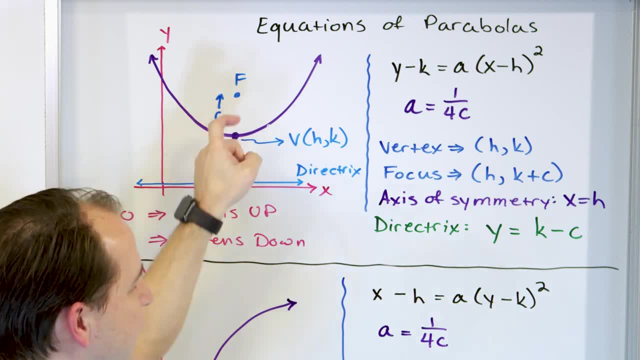 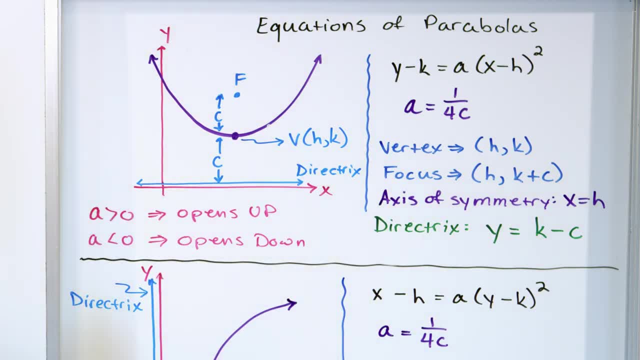 Perfect spot, right? Just think of a focusing light or something. And then on the other side of the vertex, we have a blue line, which we call the directorics. I don't expect you to know what that is, but you just need to know that every parabola, we never discussed it before, but every parabola has associated with it something called the focus and also a line called the directorics. 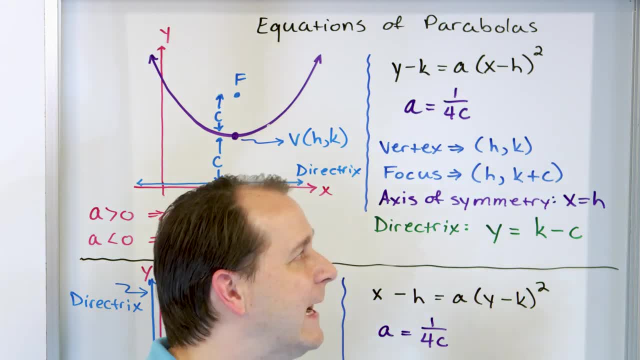 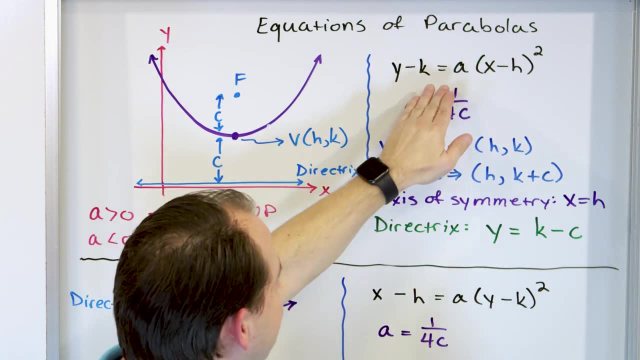 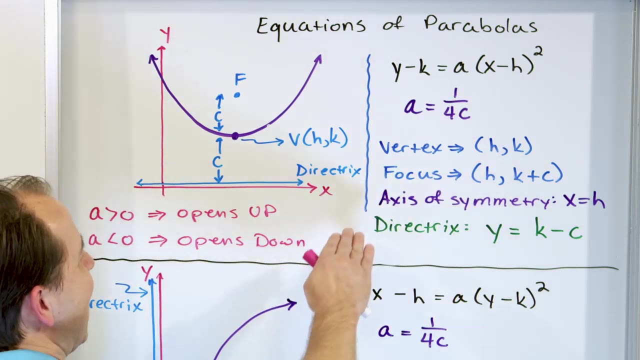 And we're going to talk at great length what the directorics is. Don't stress out about it right now. But here you have a purple parabola. It's shifted some distance in x and y, and it's shifted some distance in y. So we have the equation of the thing. This is the same equation we learned before. The vertex is given. The focus is given. We're going to talk about all of this later. The axis of symmetry is given. That's where you can cut the thing in half. We're going to talk 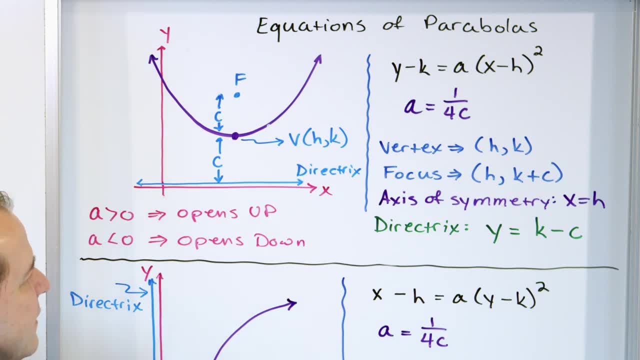 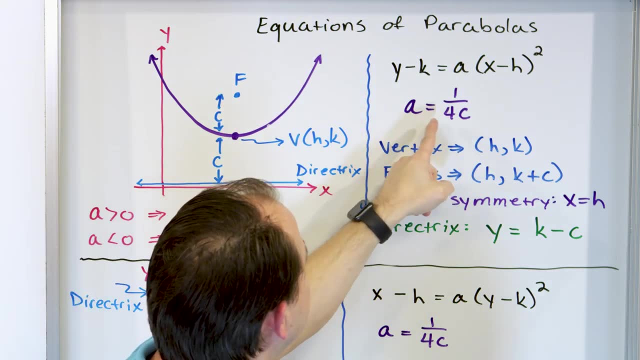 about that later. And then the directorics I've given here as well. Don't worry about what these things mean. I'm going to get to it later. And then this c relates to the focus of the parabola related to the number that's in front of the parentheses there. Remember, when a is greater than zero, when this number is greater than zero, it's going to be the axis of symmetry. 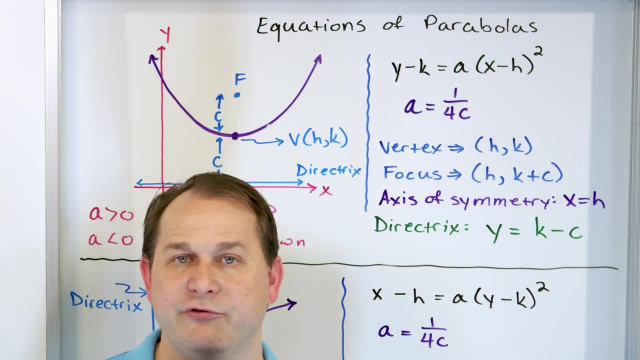 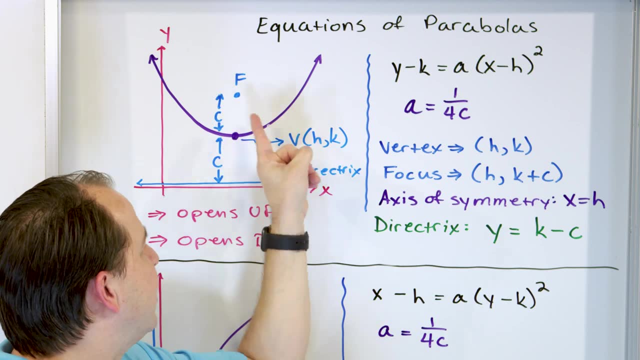 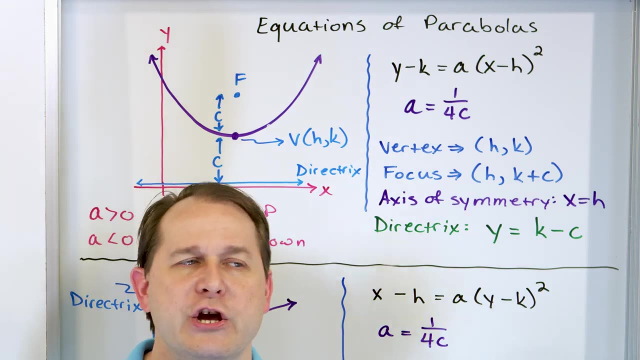 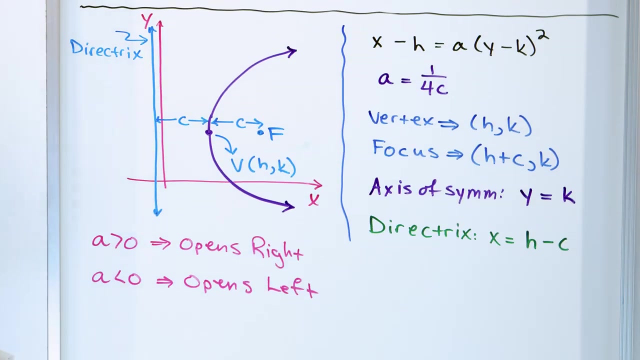 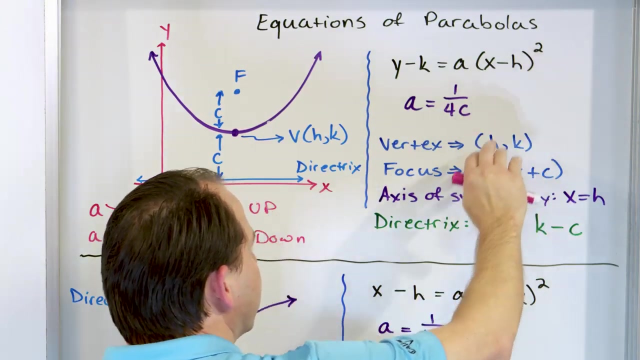 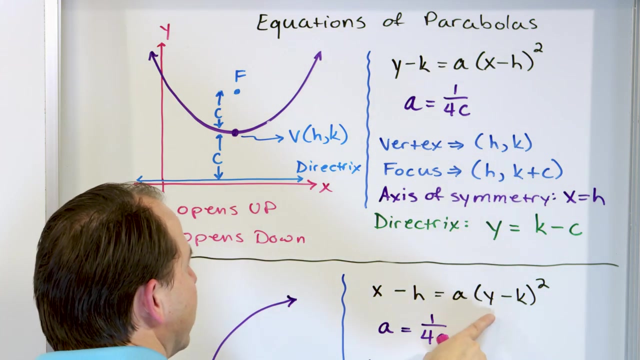 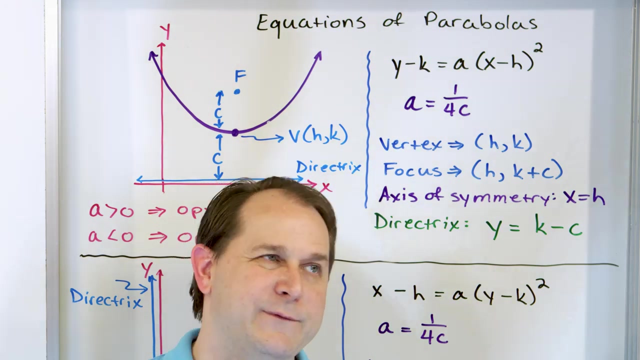 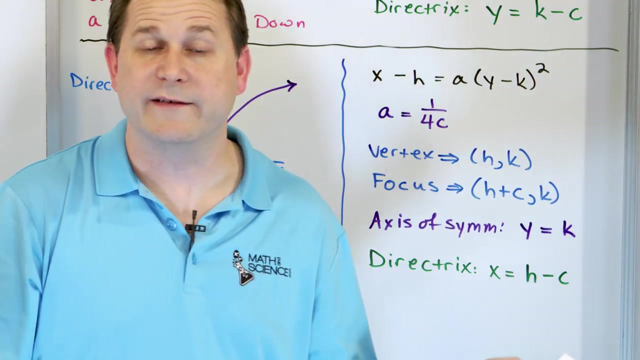 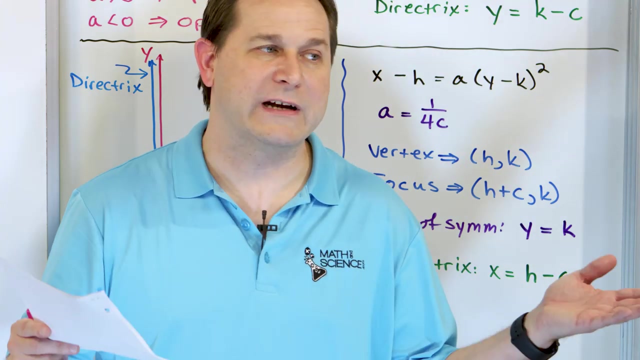 The parabola opens up, like in our example just a second ago. But if the number in front of the parabola is negative, that's what this means, then this parabola goes upside down, which we've done in the past before. So in general, you can have two kinds of parabolas. You can have parabolas that open up or down, which is really the only kind we've discussed so far in this class. But you can also have parabolas that can open left and open right. And we haven't talked about that before. So that's why I say we're going a level deeper. So here we have a sketch of a parabola that, in this case, opens to the right, right? So you can see the equation of this parabola is very similar to this one. Really, the only difference between these equations is the y has been replaced with x, and the x here has been replaced with y. So when you flip something on its side like that, what you're doing is you're interchanging the x and y variables. And because if you tilt your head sideways, really, and kind of just pretend that this is the x-axis and this is the y-axis, then it looks the same as the other one. So flip your head to the right, and then you're tilting the variables around, does the job of tilting the thing on its side. When you do your problems in algebra with parabolas, you're going to have some parabolas tilted to the side and some parabolas that are going up or down. 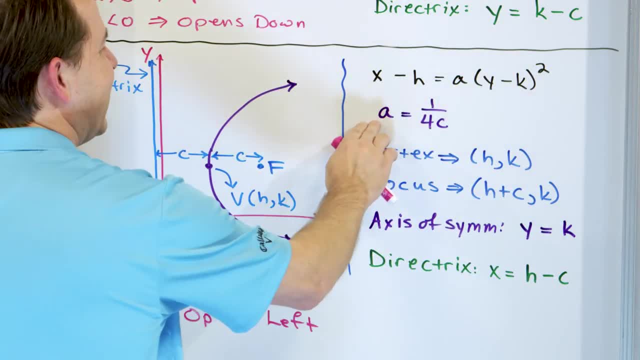 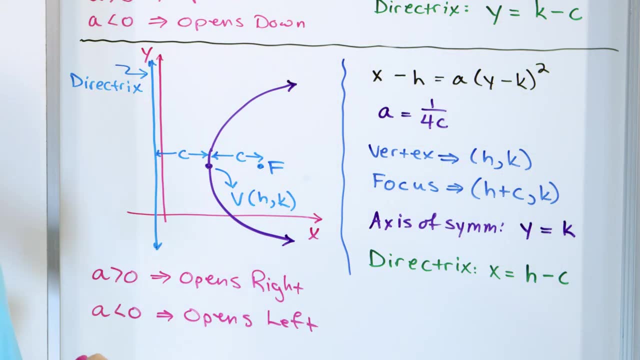 But anyhow, this is the equation of a sideways parabola. You have a same relation between the number in front and the focus. We're going to talk about that later. We talk about the vertex and the focus of the parabola. I'll discuss it later. The axis of symmetry cuts this thing in half. I'll talk about that later. And then there's an equation for the directorics, which is the blue line here. 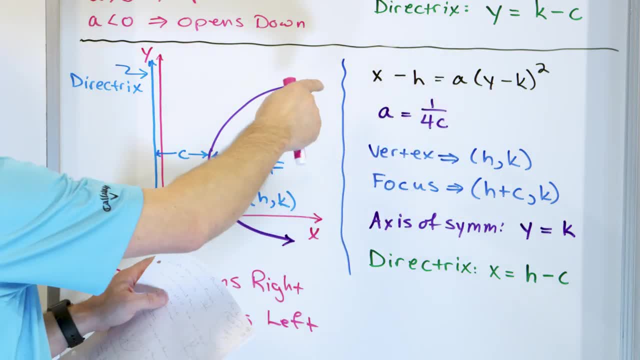 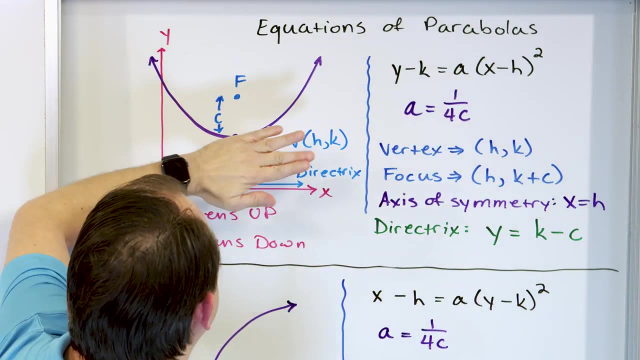 Okay. Now when a is greater than zero, when this number is greater than zero, the parabola opens to the right because these are the positive values of x. And when it opens with a negative a, then it's flipped around the other way, and it opens to the left toward the negative values. This is the same thing up here. When a is positive, the thing opens upwards towards the positive y. 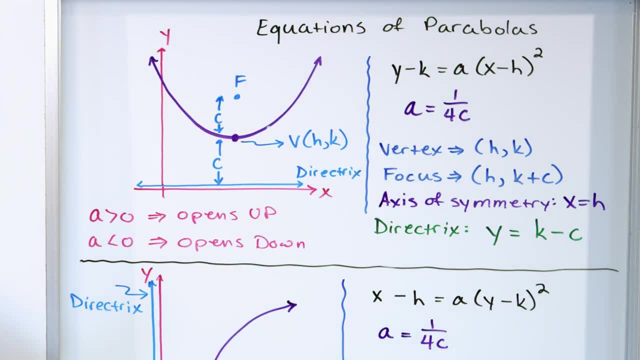 When a is negative, it opens upside down to the negative, towards the negative y values. 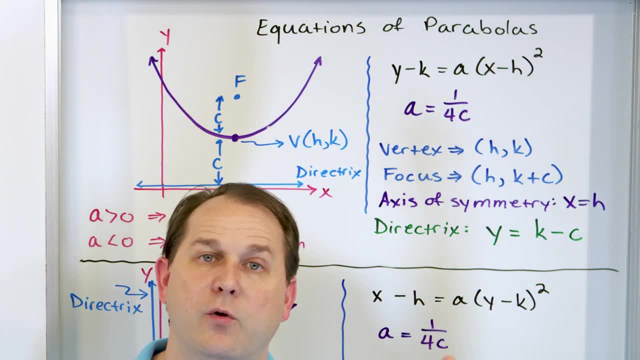 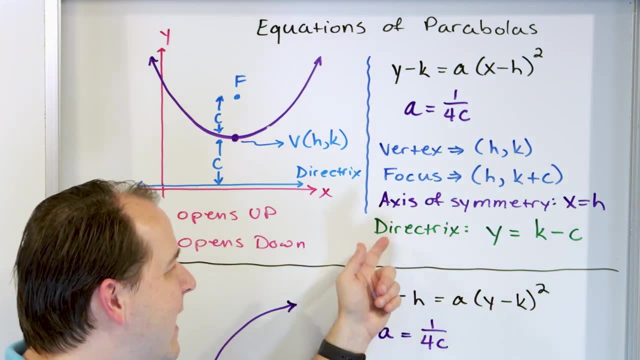 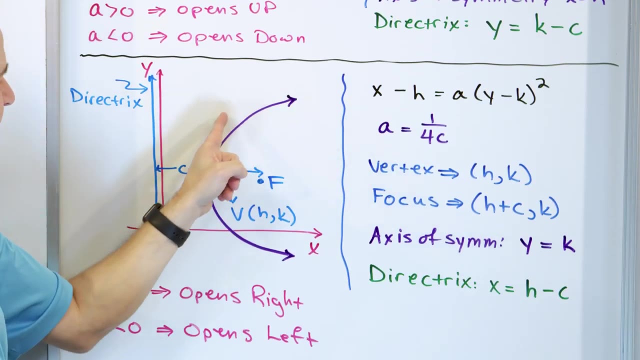 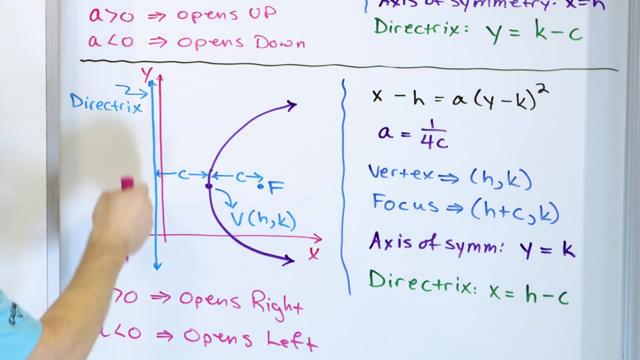 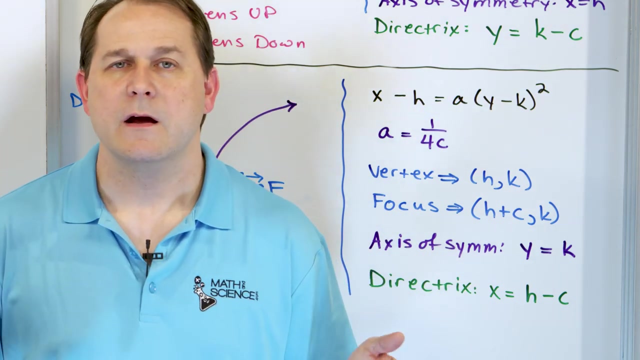 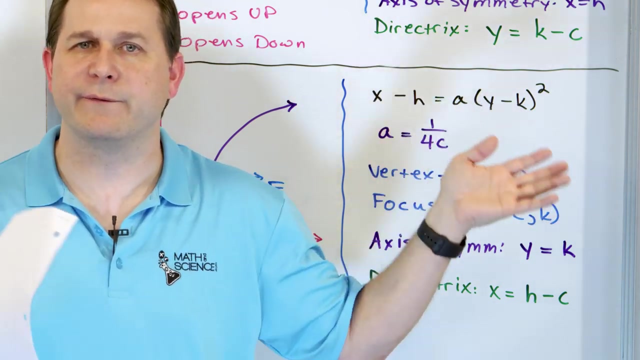 So I'm putting all this on the board to put it all in one place. You have the equation of the parabola. You have the vertex coordinates. You have the focus coordinates. You have the axis of symmetry equation. And you have the equation for the directorics. Notice that this parabola goes up and you have a directorics that goes horizontally. This equation has a parabola going to the right with a focus right here. And you have a directorics behind it. So really, if you tilt your head, it's exactly the same picture as what's above. You have focus, vertex, directorics, focus, vertex, directorics. I have to put it all there because you're going to have to do problems with both kind of situations. But what I want you to do now is kind of forget about this for now. Just in the back of your mind, remember, okay, we're going to have to talk about horizontal and 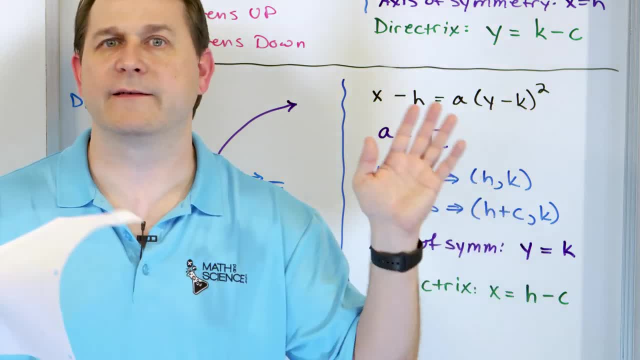 vertical parabolas. We're going to have to talk about focus, vertex, directorics, axis of symmetry. 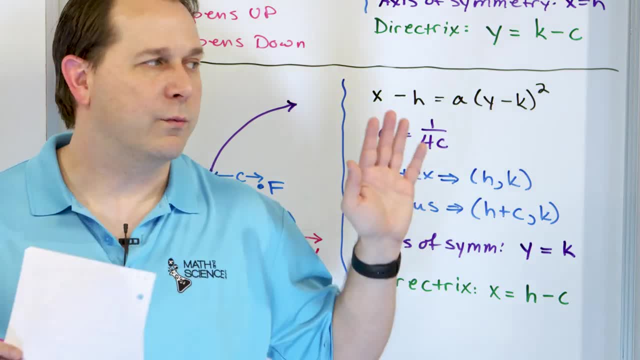 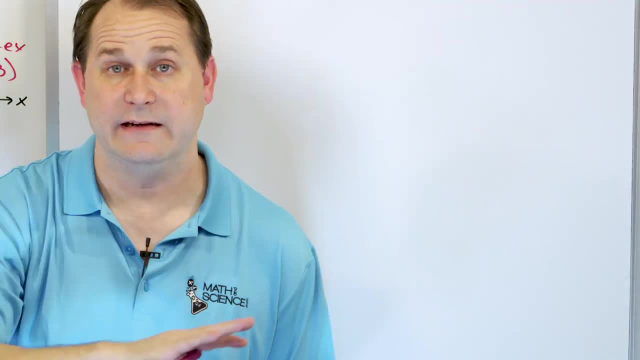 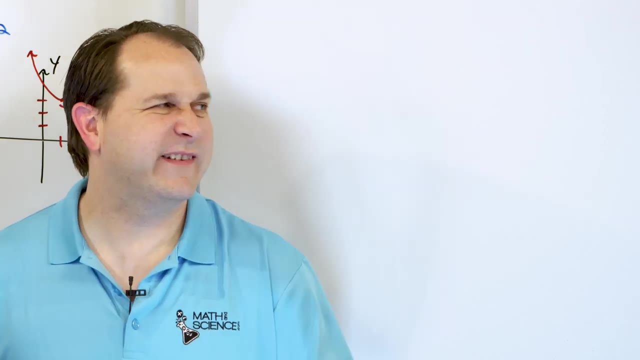 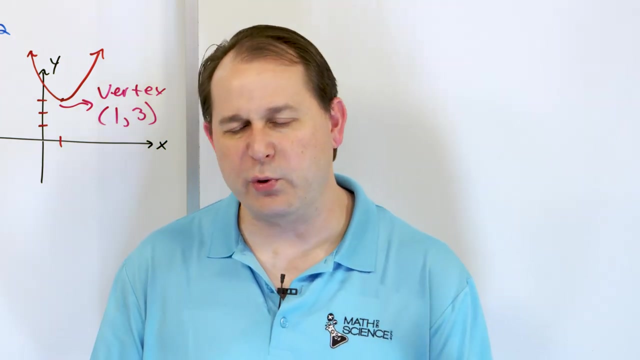 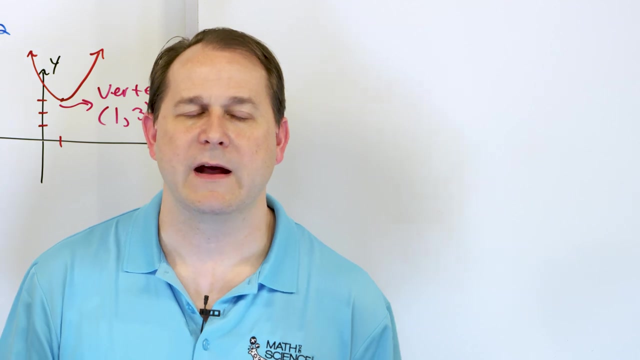 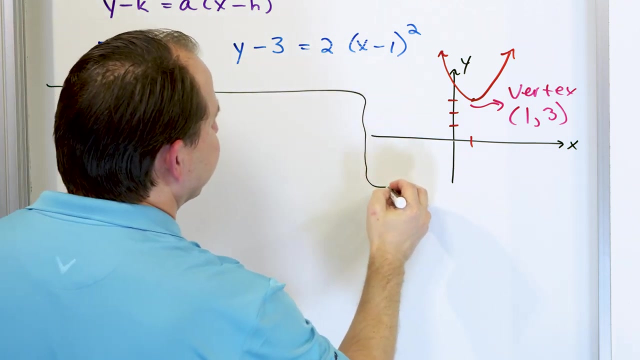 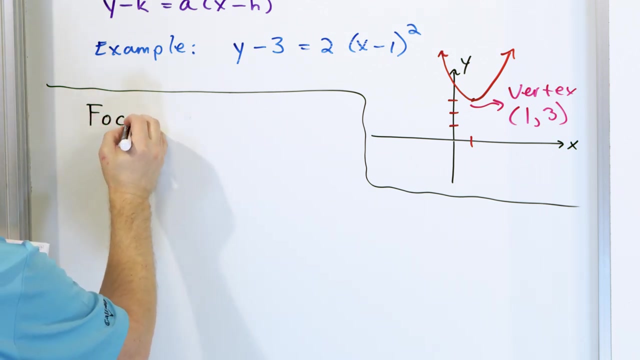 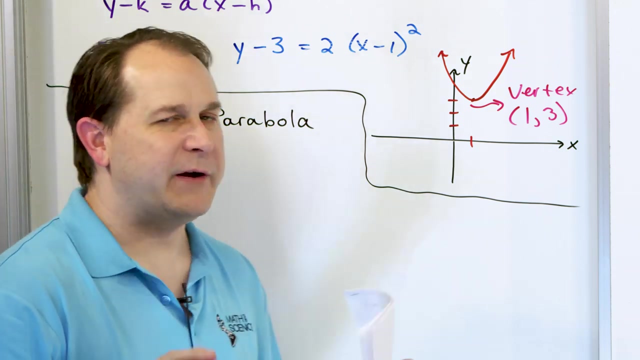 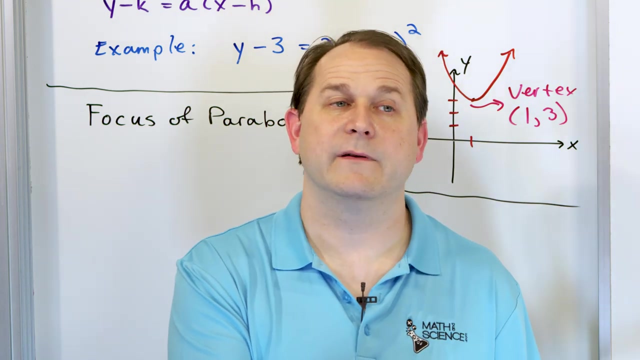 Those are all the things you're going to have to do in all of your homework problems. So keep that in the back of your mind that we're going to get back to you. We're going to circle back at the end of this lesson, and you will understand everything on that board in exquisite detail. But I have to guide you there, okay? If I just throw it at you and say, hey, good luck, you'll never know what you're doing. So go on a journey with me. It's going to be a little bit of a long lesson, but we will get there. So the next thing I want to talk about going down that road is why is the shape of a parabola so important? It's important for lots of reasons. But one of the biggest reasons, honestly, that parabolas are so important is that every parabola has what we call the focus of the parabola. Now, a focus of a parabola is very easy to understand. But in the back of your mind, I want you to remember that when we get down to ellipses later on, ellipses have foci, two focuses as well. And also hyperbola have focuses as well. 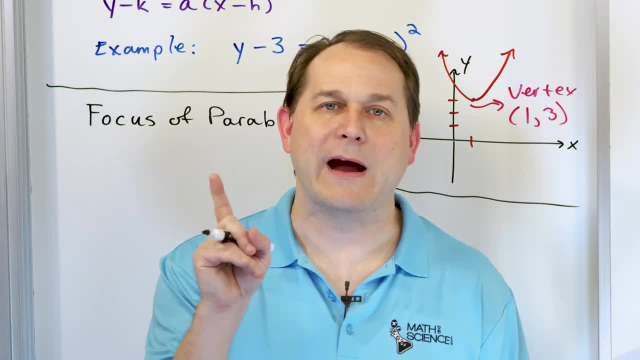 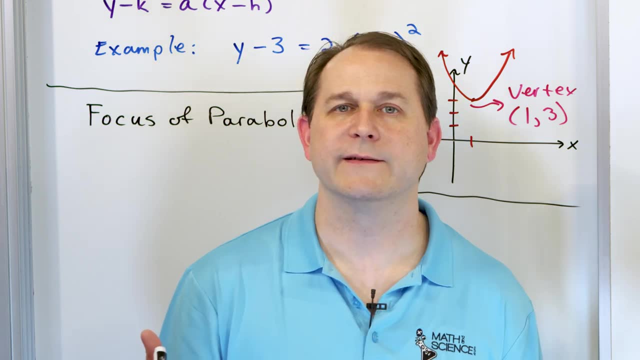 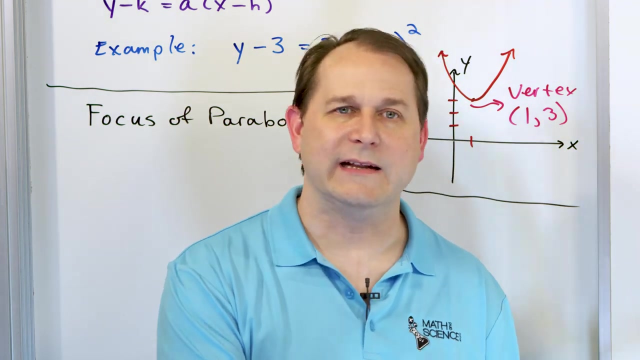 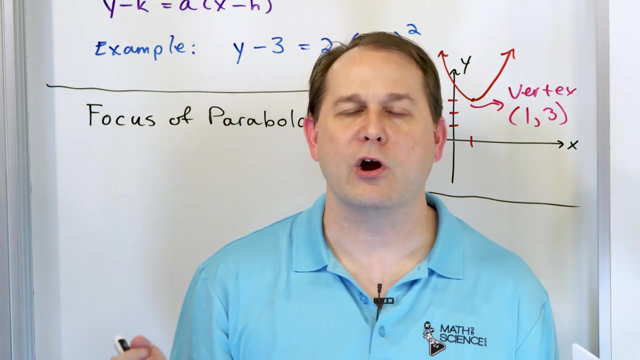 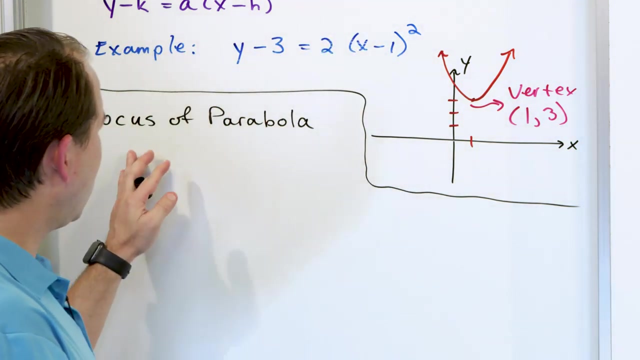 So it's not like parabolas are so important. They're not so important. They're not so important. Parabolas are the only thing that has a focus. A parabola has one focus, one dot. And ellipse actually has two of those focuses. We call them foci. That's the plural of focus. And then hyperbola also have two foci. So the concept of a focus, it's going to stick with us as we talk about ellipses and also hyperbolas down the road. And actually, the circle that we've been talking about forever also has a focus as well. It's just the center of the circles. We don't call it the focus. We just call it the center, right? So all of the focus is going to stick with us. And so these conic sections have something called a focus, right? But the parabola's focus is super, 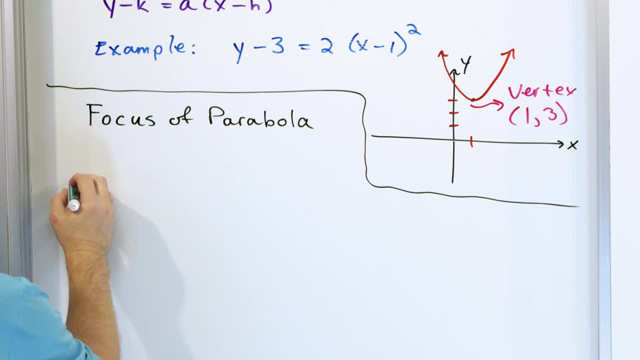 super important. Now, let me try to draw this. It's not going to be perfect, but I'm going to try to draw a good shape parabola. Is this a perfect parabola? No, it's not. I can almost guarantee you because the bottom here is too flat. But it's my best shot at a freehand parabola. 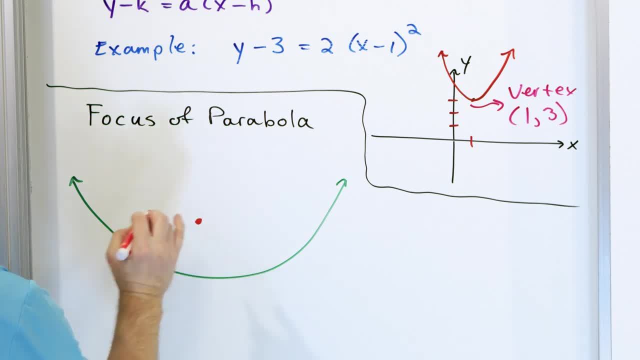 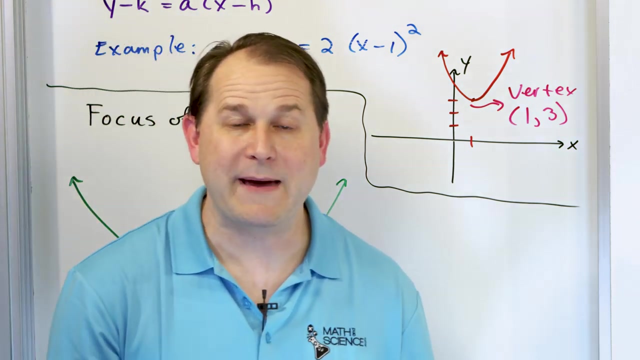 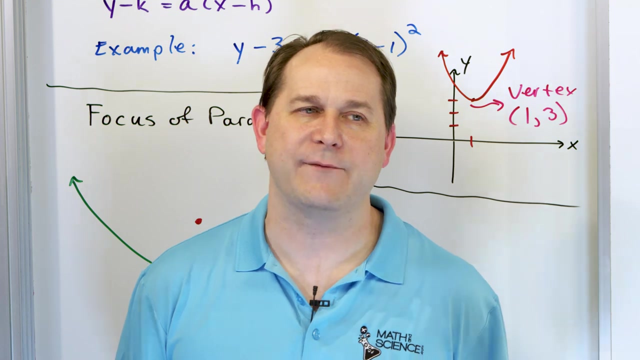 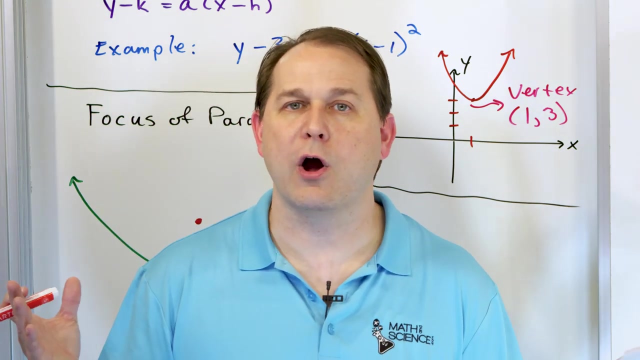 So if this were a parabola, the focus would probably be somewhere right around here. I'm just guessing because I don't have graph paper and all that. But let's just say the focus is right here somewhere. Every parabola shape, whether it's really wide open or really, really steep, is going to have one focus at one location, right? The focus is called the focus because it takes, if you can imagine this thing being a radio dish, which is really one of the main reasons we use parabolas in real world, all of your satellite dishes from the gigantic radio telescopes we have all the way down to the small satellite dishes for your television or for your whatever dishes you see on a tower somewhere. They're all parabolas. They're all parabolas. They're all parabolas. 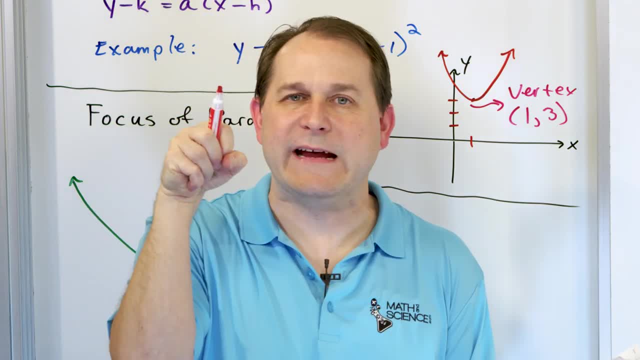 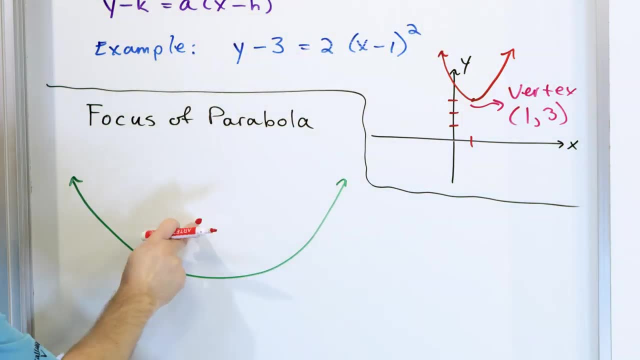 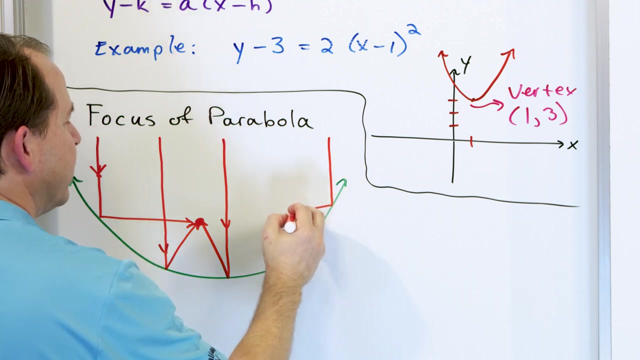 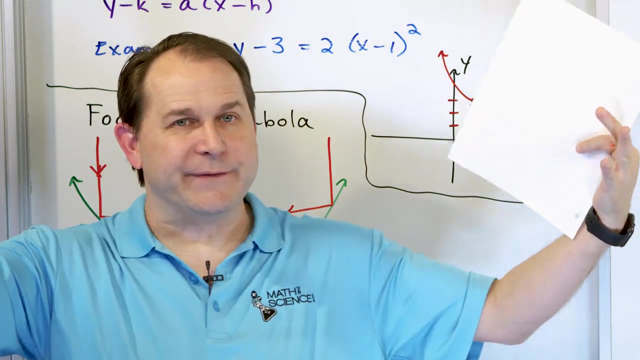 And the receiver that's in there or the transmitter is at the focus of that parabola. It's the thing that's kind of suspended in the center, right? So this thing would be the transmitter or the receiver. And that means that any light waves or radio waves that come in are going to bounce off of this curved surface and they're going to go this direction towards the focus. But I also have a light beam, not just right here, but I have light beams everywhere. I have a light ray coming in here like this, and it's going to bounce off that bottom. And hit the focus as well. Notice it's curved differently than it is right here. If I take another one to the other side, it's going to bounce off and hit this right here. And I know that it's a little hard to see because my parabola is not perfect, but you can see because it's constantly curving, no matter where I stick a light beam, it's going to bounce and it's going to hit this focus point right here. I can take one way over here, in fact, and it's still going to come off and bounce and hit into this guy. So that means that if I create a parabola in a special way, and I put the transmitter or the receiver, like when you look at the big radio telescopes, there's always like the scaffolding with the thing hanging in the middle, like above. That's because that's the focus of the parabola. Because if I'm going to receive light or radio waves from space, 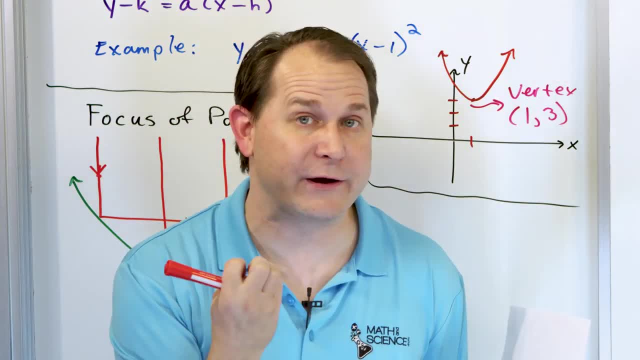 it's going to concentrate them at the focus so I can hear them better because I'm concentrating it like a magnifying glass would concentrate light, right? Or if I want to broadcast something, 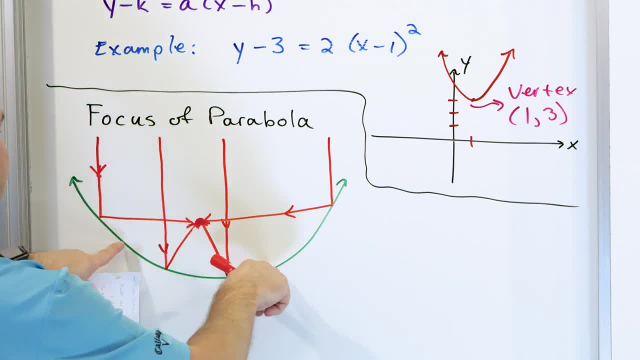 this whole thing works in reverse. If I'm going to shoot energy out of here, no matter which way I'm going to shoot energy out of here, no matter which way I'm going to shoot energy out of here, no matter which way I'm going to shoot energy out of here, no matter which direction I shoot it toward the dish is going to bounce it this direction. So you can 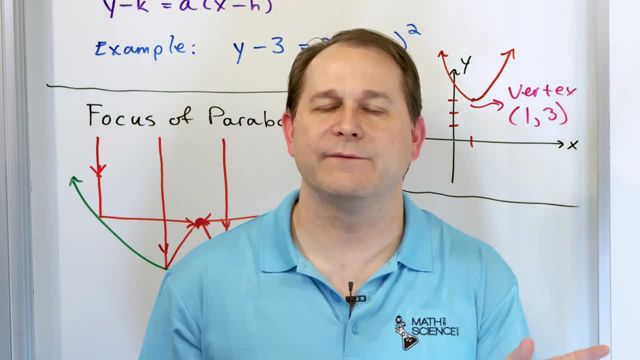 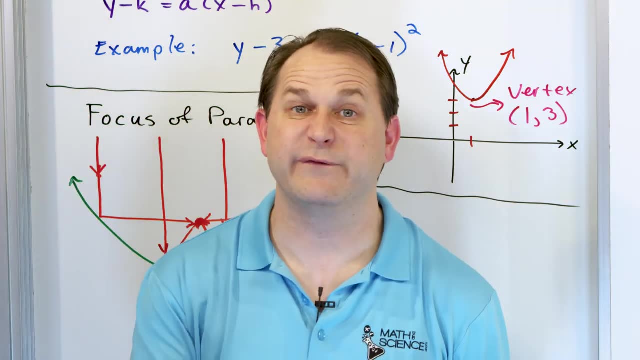 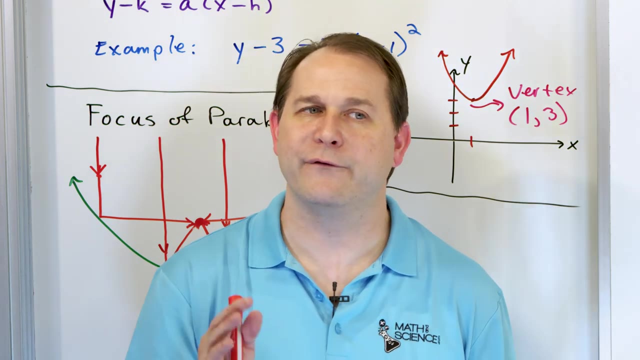 think of, you know, like the Death Star in Star Wars is not a great example, but that's kind of like the focus of the parabola. You can see it kind of bouncing in and going out or coming in and bouncing up to the receiver. That's the focus. And as I said, parabolas have a focus, ellipses have foci, two focuses, hyperbola also have two foci. So focus is a central thing for conic sections. Circles have a single focus also, it's just at the center, right, of the thing. 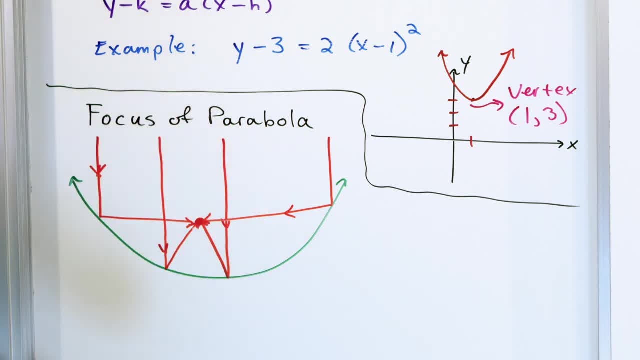 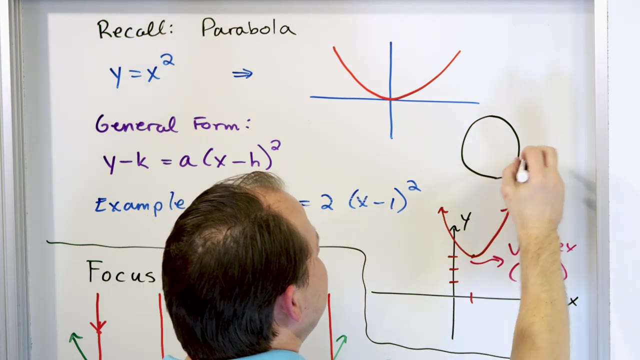 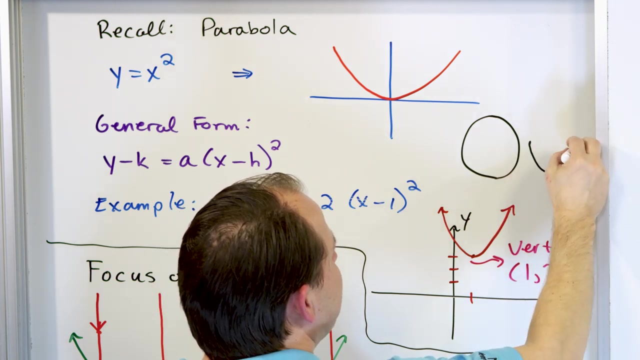 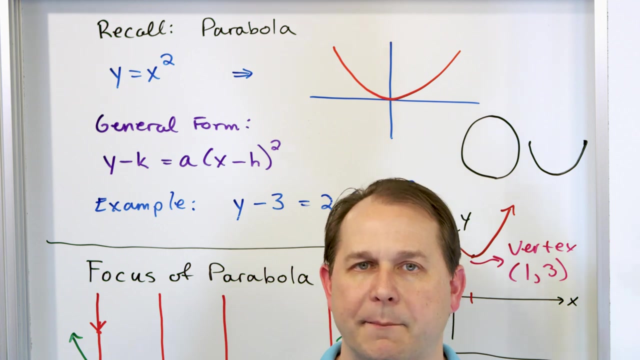 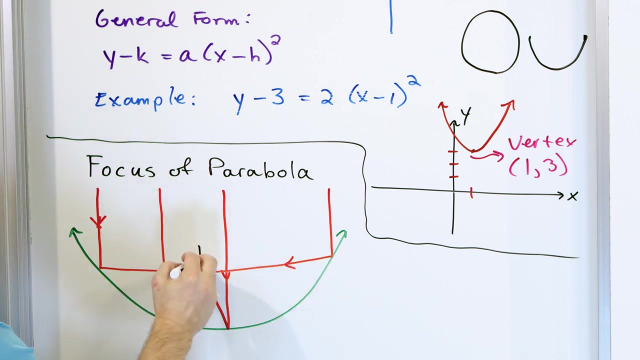 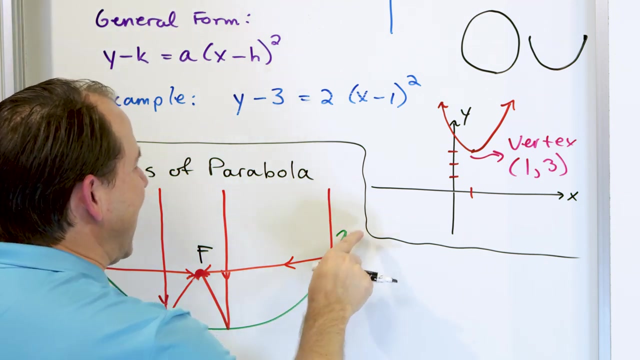 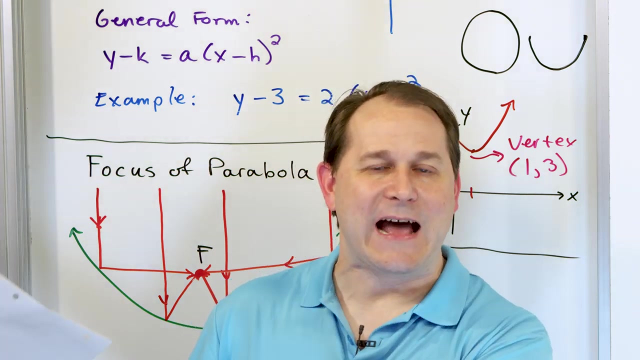 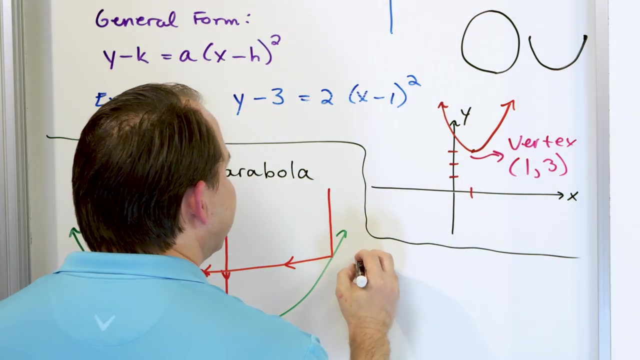 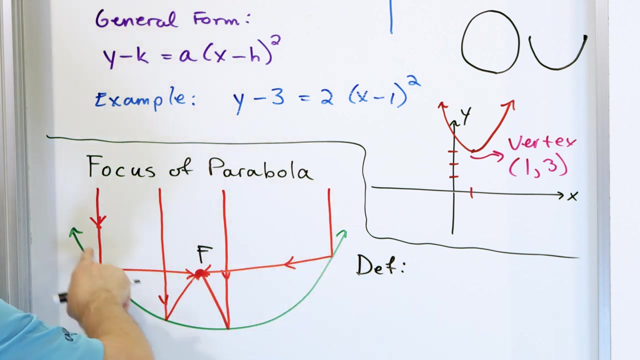 All right. So this is a useful feature of a parabola, but what is this special shape? Clearly this special shape is not a circle. This does not look like a semicircle. If you could think about a circular shape, what does a circle look like to you? A circle looks something kind of like this. So this means a semicircle is the bottom of this thing. A semicircle would be something kind of like this. Actually, that's not even a semicircle, a perfect semicircle. It should be going more up and down right there. This shape will not reflect those rays in the proper way towards a focus like a parabola does. It has to be opened up more into the shape of a parabola in order to bounce everything into the focus right here. That's called F, the focus point right there. But the question remains, what is the special shape? What is so special about it? How do we define what the special shape is and how do we know that Y is equal to X squared is that shape that is the special shape that focuses things? That's what we really want to know. Okay. So here I'm going to write the definition of the parabola. I'm going to write it right here and then I'm going to draw one more picture to set up how we're going to derive this green curve. We're going to actually derive the green curve and show that it's equal to this equation or to this form of an equation. So 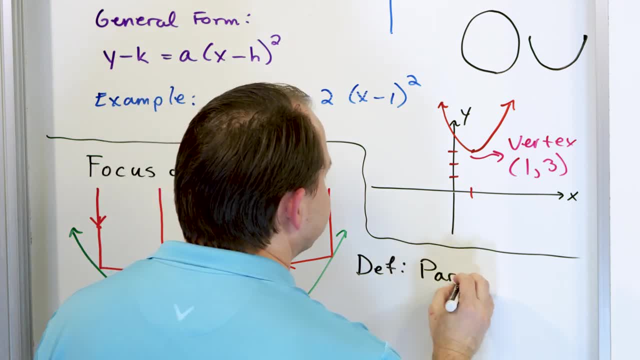 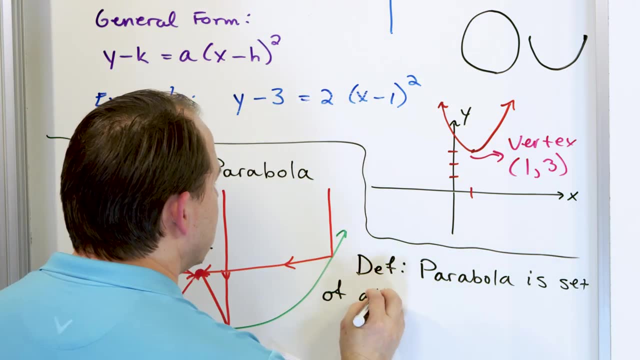 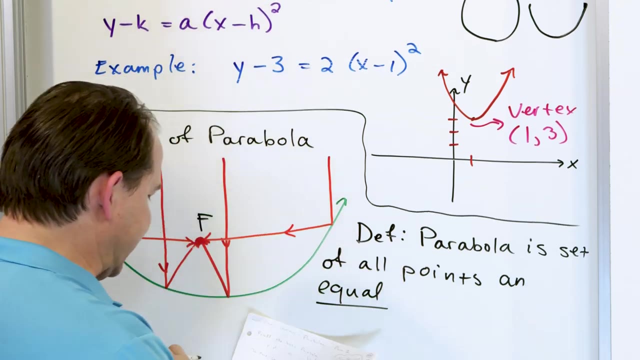 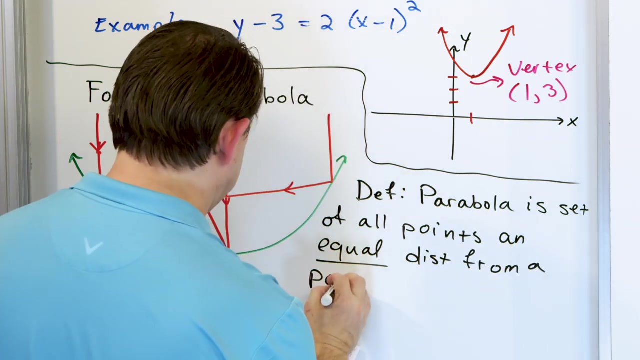 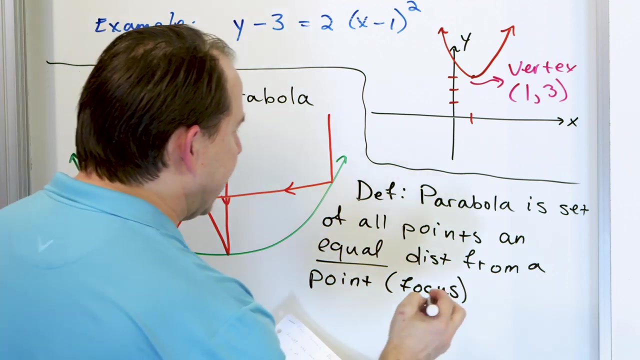 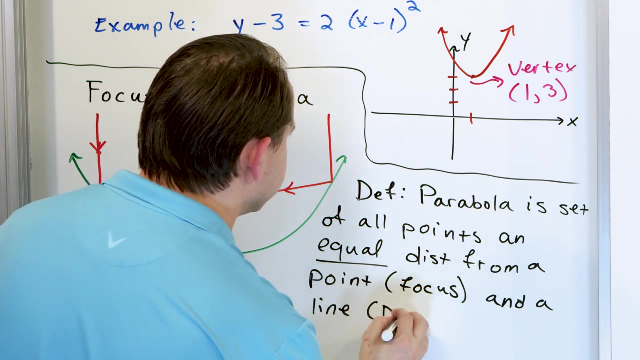 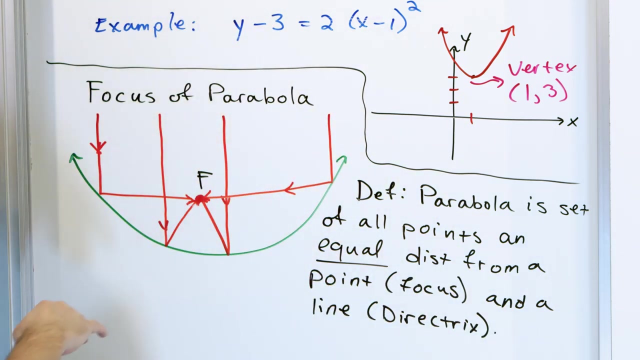 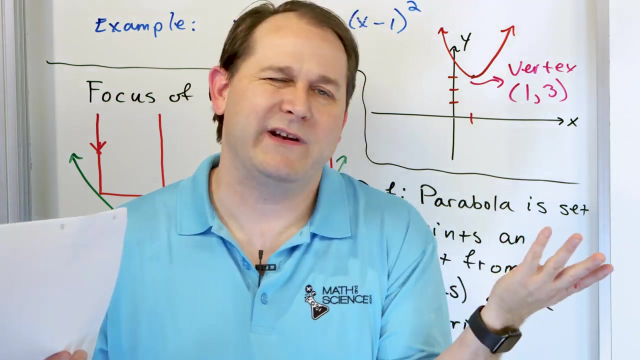 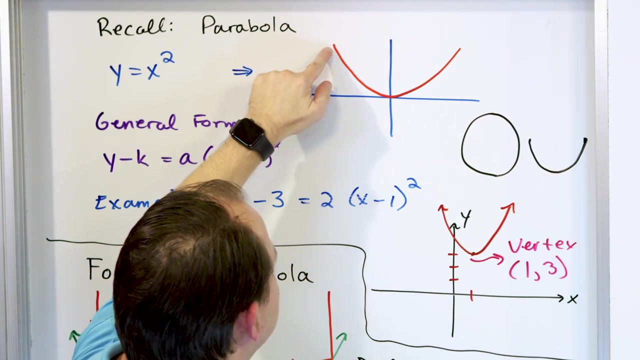 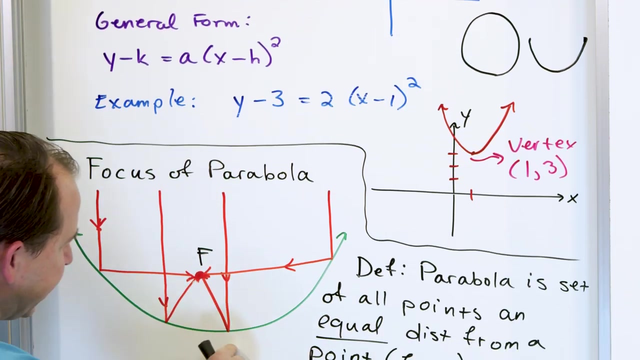 the definition of a parabola says parabola is the set of all points and equal distance. So I'm going to underline that and equal distance from a point. I'm going to call that point the focus. Focus is central to the concept of a parabola. And a line. And this special line is called the directrix. We're going to read this a couple of times. We're going to let it sink in one more picture to kind of set it up. A parabola is just a shape. It's the set of all points that define that shape. What does that mean? If this is a circle, all of the points along this black curve define what the circle is. If this is a parabola, all of the points inside the red curve define what the curve is. If this is a parabola, all of the points that define the green curve define the set of points that we call this thing a parabola. So we're saying a parabola is the set of all points. 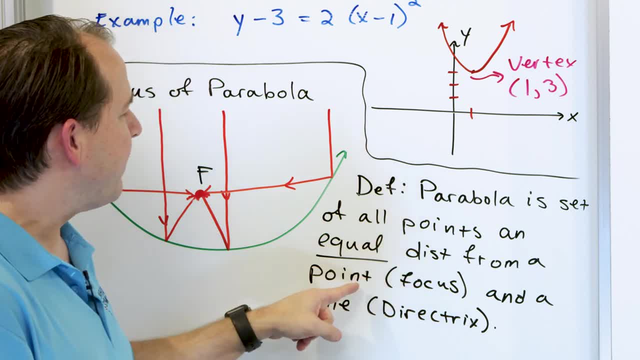 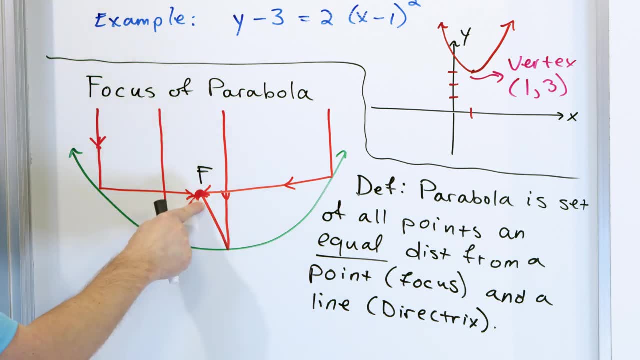 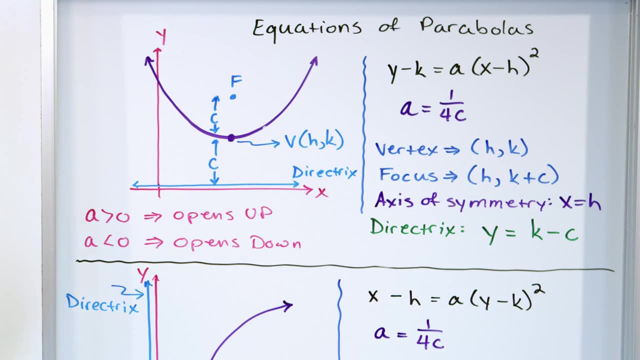 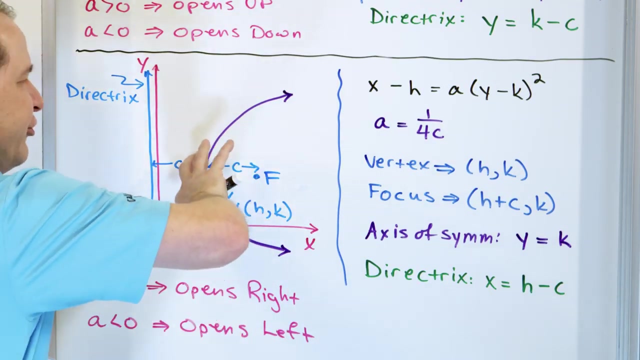 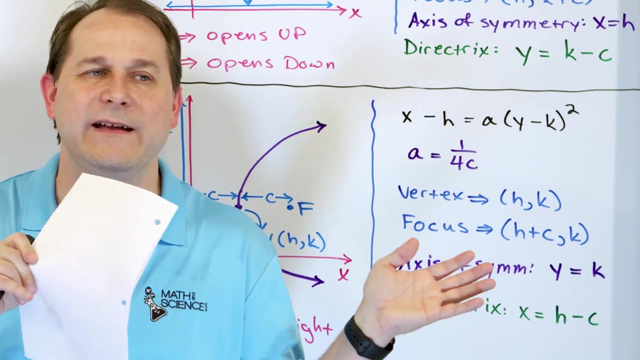 That means the green curve. That are in equal distance from a point called the focus and a line called the directrix. Now I haven't drawn the directrix here, but you can see the focus is here. The directrix is always somewhere behind the parabola. In fact, when you look, I know I told you to forget about this, but if you see every parabola you have, you always have a focus up above. And then on the other side of the rear end of the parabola, you have this blue line called the directrix. So you can kind of think of the directrix as this kind of like this black, glass shield that's kind of behind. If you think about this thing as like a death ray or something, like a gun trying to shoot energy off like a death star or something into space or something, then it's going to shoot everything this way. And back behind it is this thing called the directrix. If you tilt it off to its side, you have a focus here. You're shooting your energy out this way and you have a directrix that's kind of behind it. That's the line that defines the other. It's in the definition of a parabola to define what the shape of a parabola is. 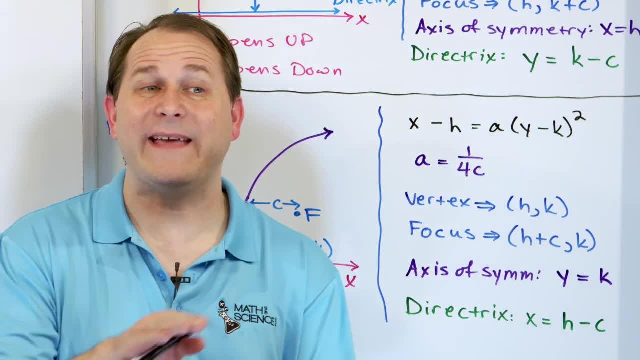 In other words, if I take any line I want and any point I want, which I'll call the focus, then given any line 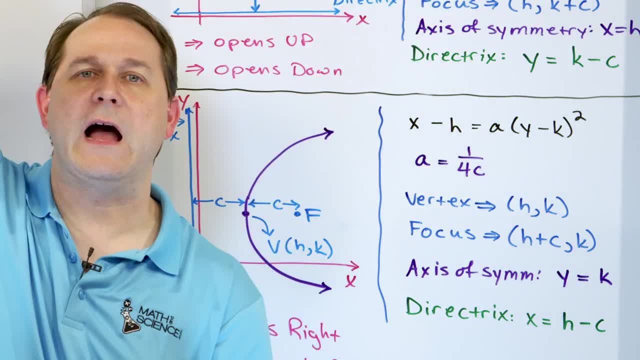 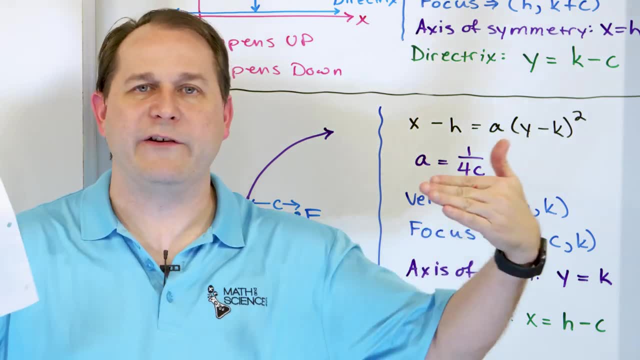 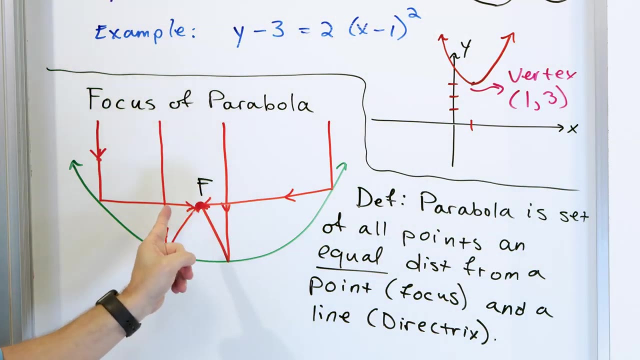 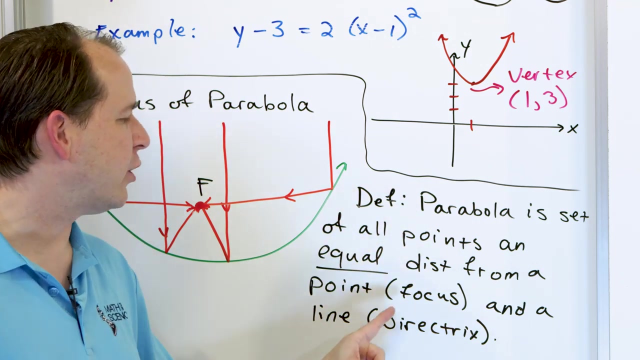 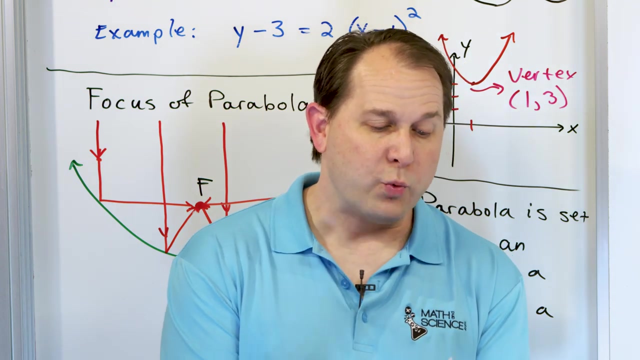 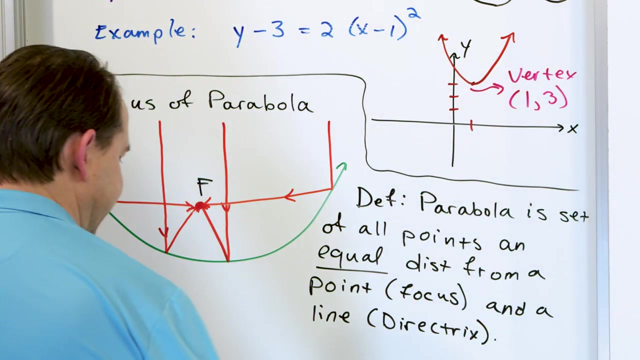 and any point, I can always choose or I can find that beautiful parabolic curve that fits between them like these do. That is the perfect shape of a parabola, meaning it will always reflect incoming rays to the focus, just like in my diagram right here. All right. So let's take this definition. Parabola is the set of all points in equal distance from a point called the focus and a line called the directrix. So let's take those words and let's translate them into a picture. And then once we translate them into a picture, we will have what we need to derive and figure out what the shape of this curve actually looks like, which is what I'm trying 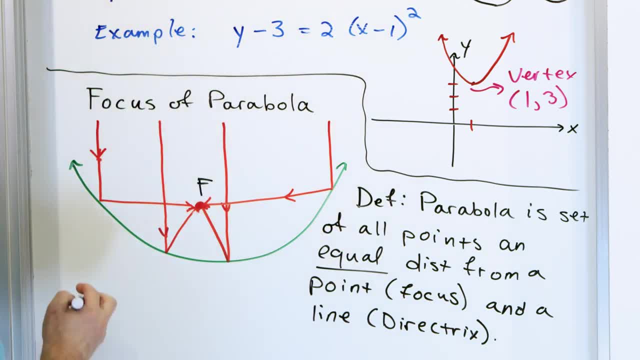 to get to. Before we get to that, let's draw one more picture of this whole situation. 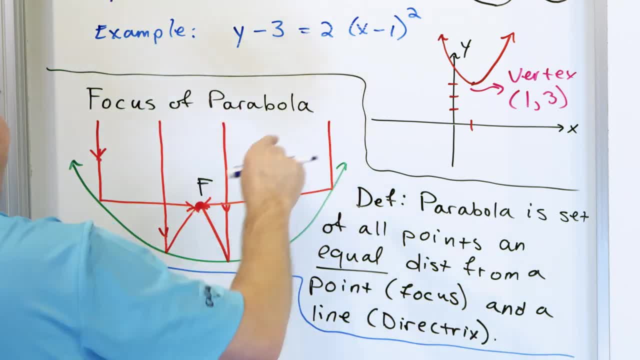 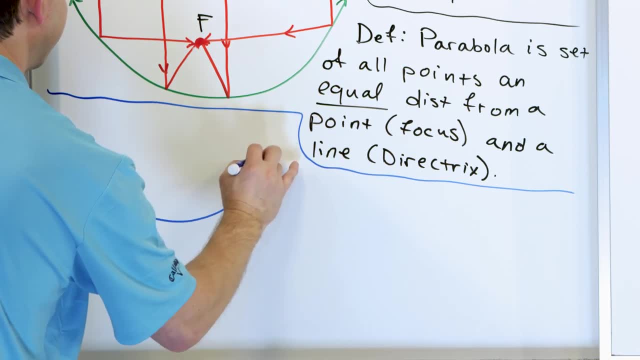 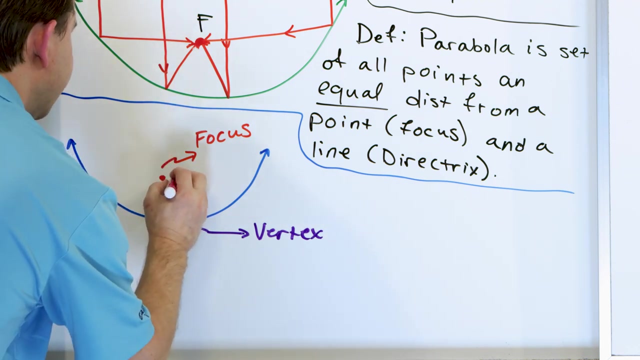 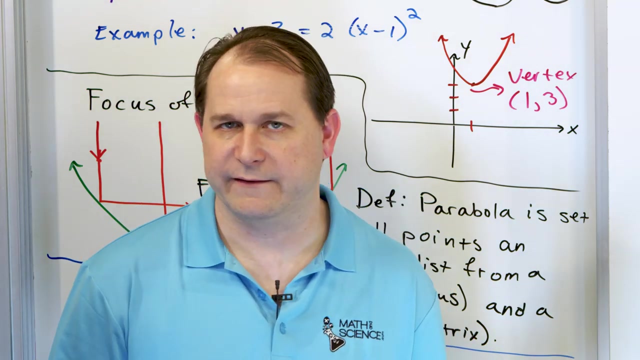 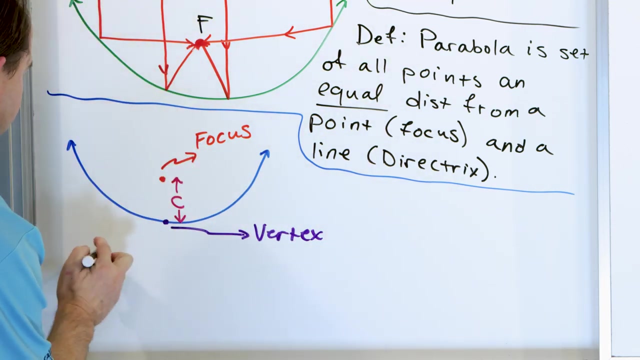 That'll make it a little more clear. So I'm going to redraw what I have above with the green curve, right? I'm going to draw a parabola and it's not going to be perfect. Forgive me because I'm not good at drawing things. I cannot draw perfect parabolas by hand. So this shape I'm going to call some kind of parabola. Okay. Some distance above and kind of inside the bowl is some point, a special point called the focus that's going to accept all of the incoming rays. It's going to focus it at that point. So this point is called the focus, which we discussed before, right? Now the distance between the focus and the vertex, which I haven't, really talked about yet, but there's the point, the lowest point of the parabola here is called the vertex, which we've discussed when we did parabolas before. So the focus is always some distance above the, the, uh, vertex, some distance C. So I'm calling it C because depending on the shape of the parabola, the focus will be in different locations, but it's got to be some distance above it. So we just call that distance C, but whatever distance this is right here, there's always a special line on the backside underneath the rear end, which we call the directrix. It's always a line that goes horizontal. If 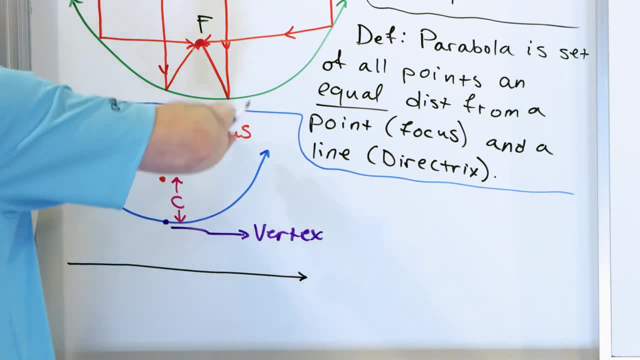 it's a horizontal parabola, vertical, if it, you understand what I mean, if it opens upwards, it's a horizontal line. 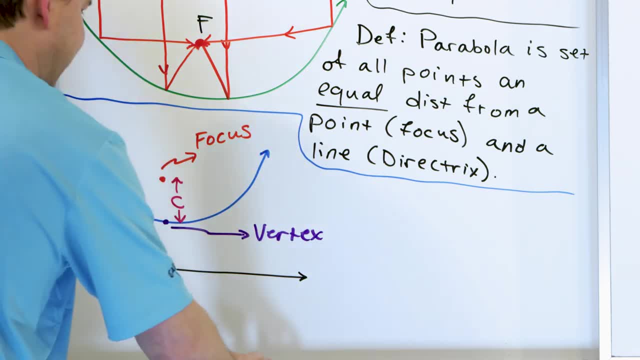 If it opens sideways, it's a vertical line. But the interesting thing and the special thing is that the distance between the vertex is also a distance C to the directrix. So this thing is called the directrix. 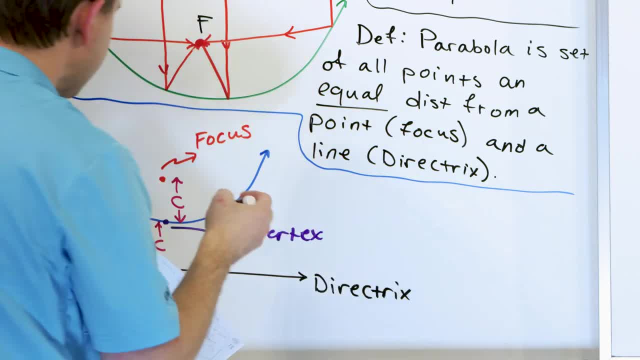 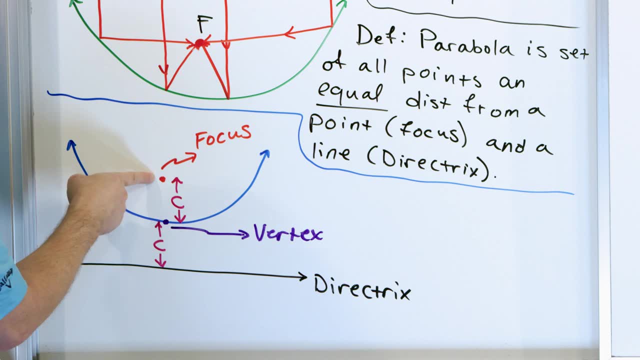 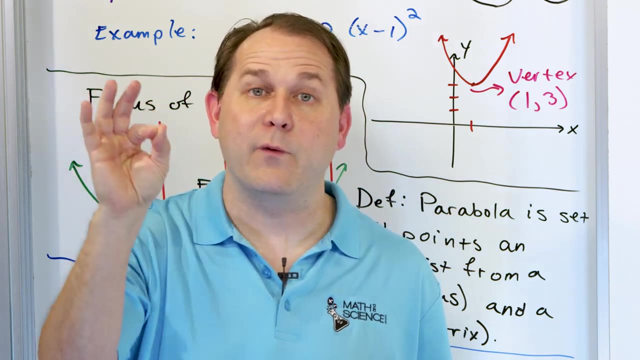 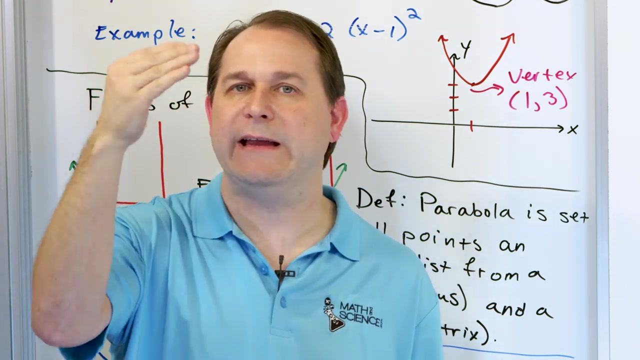 Okay. So it's crucially important for you to understand that the vertex is always halfway between the focus and the directrix. I'm going to say that again. The vertex, the lowest point of the problem is always halfway between the focus and the directrix. I'm going to say it a third time. The vertex is always halfway between the focus and the director. 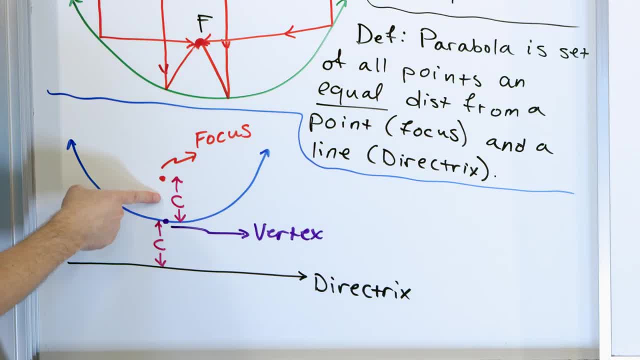 So here's the focus. Here's the directrix. This is a distance C. This is a distance C. So the vertex has to be in the middle, right? It's always halfway between like this. So 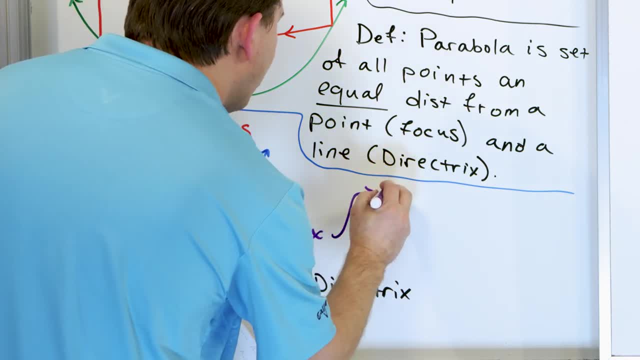 I can even write that down and I can say the vertex is always one half the way, the between, focus and directrix. 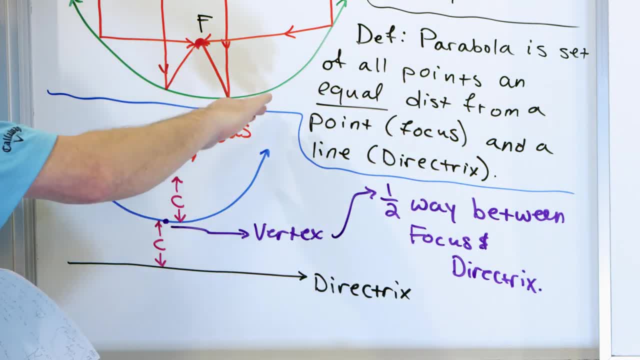 So now we have a pretty complete picture. We have a parabola drawn on the board. We have a focus of the parabola, which is going to focus all the incoming light beams or radio waves. 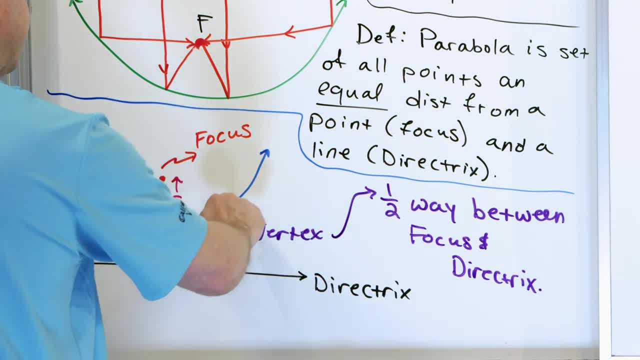 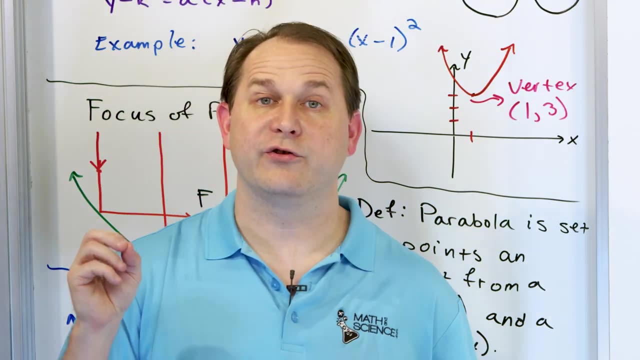 We have a directrix, which sits on the backside. And we're saying that there's a special shape, which is the blue curve, which we call a parabola. And we're saying the definition of a parabola is the set of all points, that's the blue line, an equal distance from the focus and the directrix. An equal distance from the focus and the directrix. 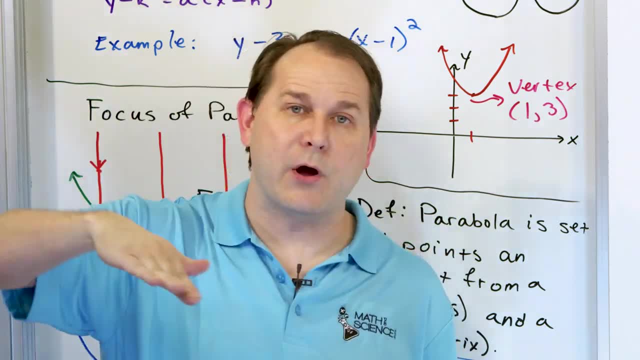 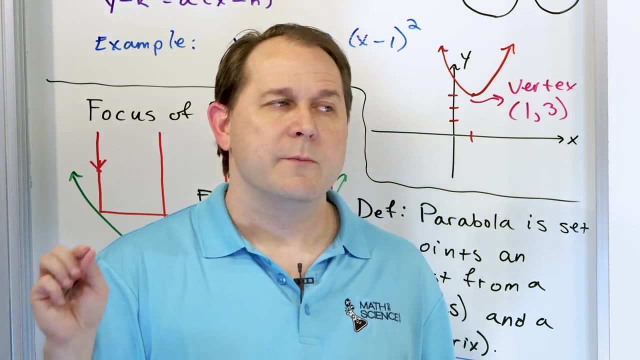 I'm saying it again to get it into your head. A parabola is the set of all points for that blue curve. That is always every point on that curve is always an equal distance between the focus and the directrix. 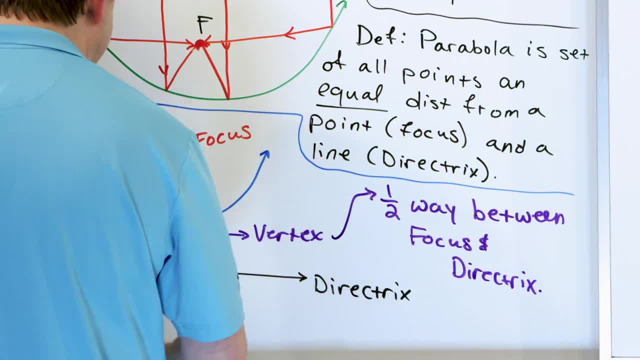 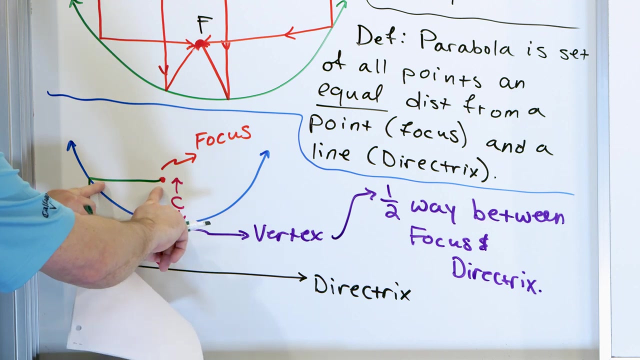 And that line that we call the directrix. So let's talk about how we make that happen. What this thing is saying is that this blue curve is the set of all points we're calling a parabola. The distance between this focus to this point on the parabola is the same as the distance between this and this. Now if you, my drawing is not perfect. So it looks to me like this line is a little bit shorter than this one. But if I had opened up my parabola, or maybe moved my focus. 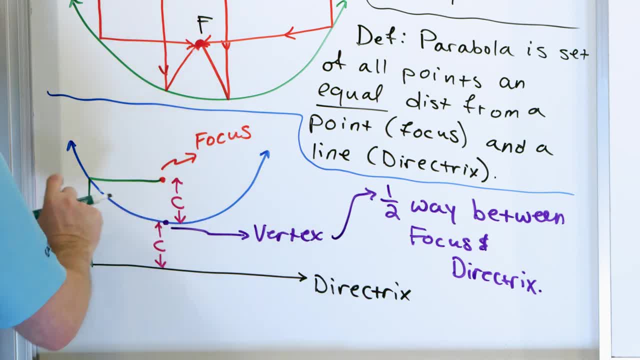 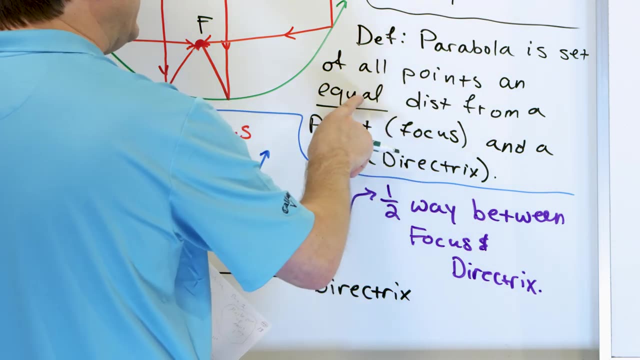 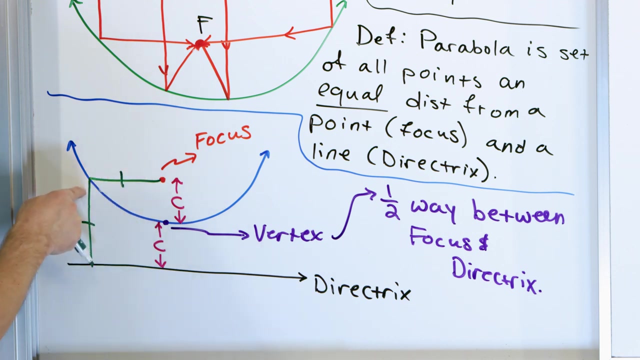 A little bit more exactly, this line should be exactly the same as this one. Now in geometry, the way you denote two lines being congruent is what we call it in geometry. We're going to put a little line through there and a line through there. That means this distance is the same as this one. That means that the parabola is the set of points that's an equal distance from the focus and the directrix. So this is an equal distance. This point here is an equal distance to the focus and also to the directrix. What if I pick a different point on this parabola? 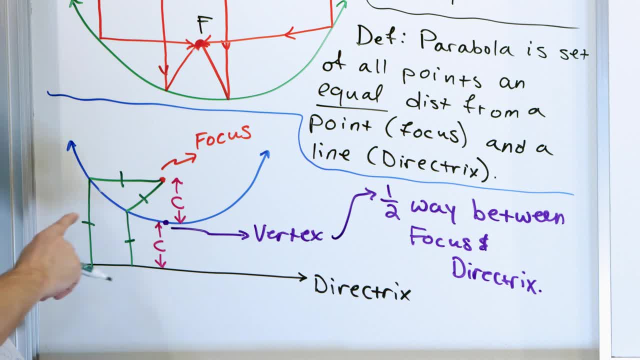 Here and then straight down here are equal distances. This point on the curve we're calling the parabola is an equal distance to the focus as it is to the directrix. What if we go crazy and we pick a point way over here? Well that's okay. This is farther away. Sure it is. But so is this one. This one's farther away to the black line. So this is an equal distance from there and there. Now of course it doesn't just happen on the left hand side. It happens on the right hand side too. So I'll go ahead and draw one going way over here and then one going way over here. This distance is the same as this one. 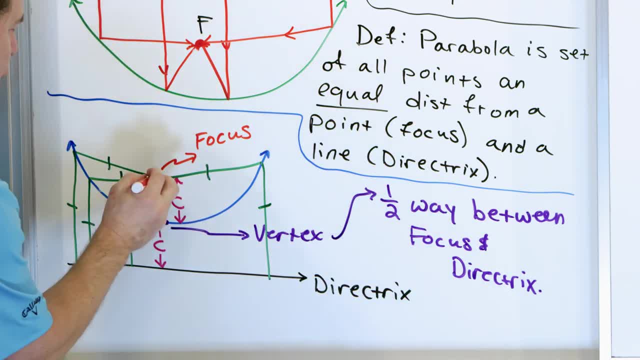 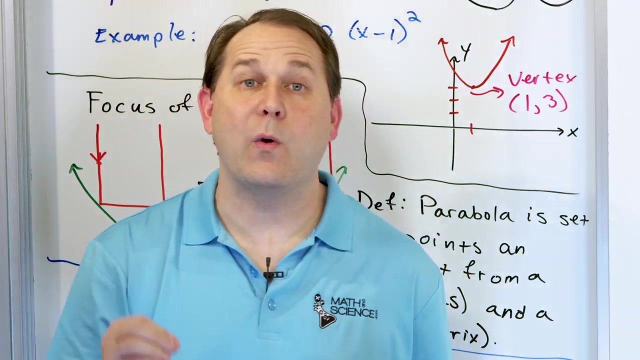 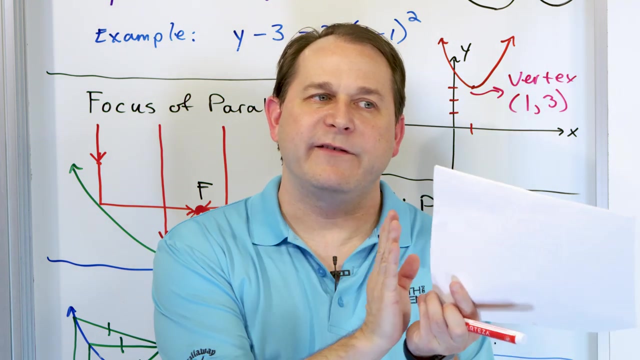 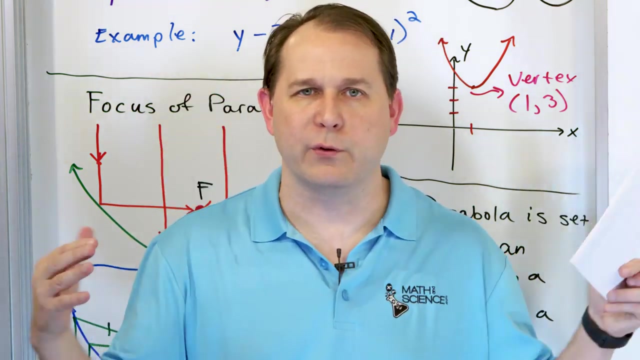 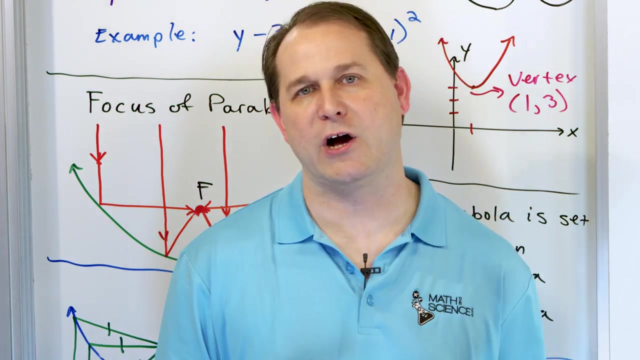 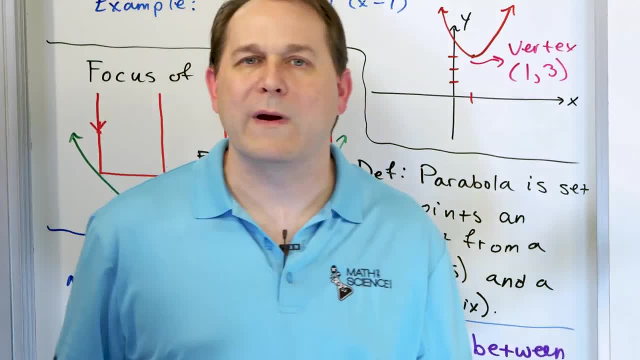 This kind of thing is not what you learn when you first learn about what a parabola is. We talk about a parabola y is equal to x squared. You just say, oh, it's a parabola. Great. 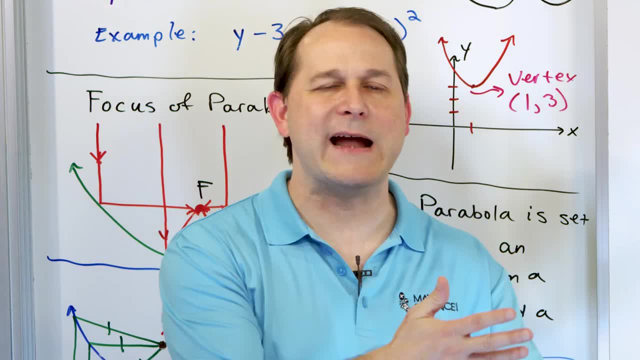 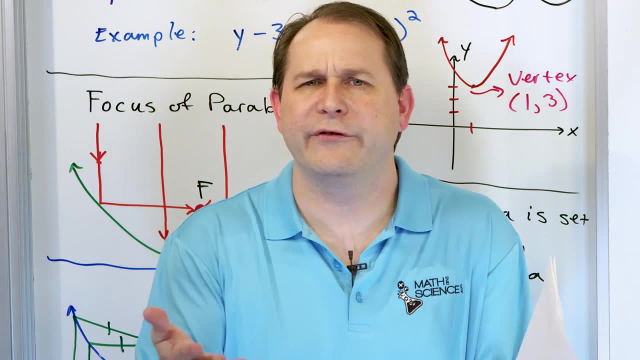 We graph it. We talk about it. Even in calculus you learn how to do things with parabolas. But until you get to a lesson like this, you don't understand why we care about parabolas, why they're so special. A circle is another special shape. It's the set of all points 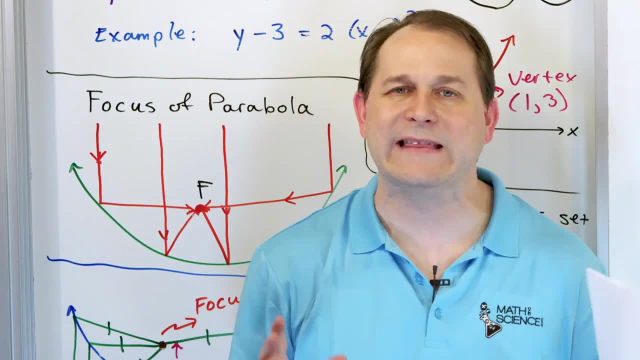 equal distance from the center, an equal distance from a single point. That's what we call the special shape, called a circle. A parabola is a special shape where every 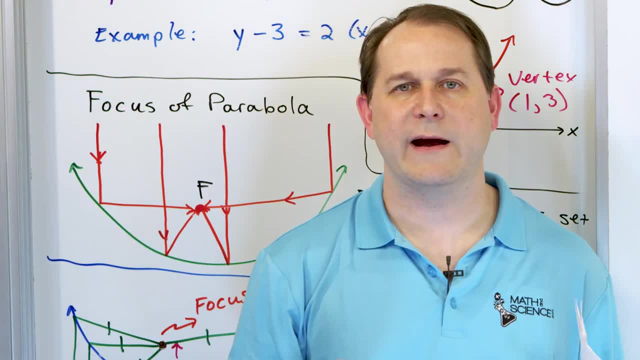 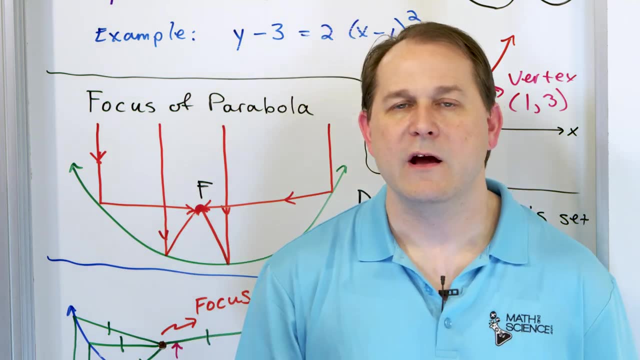 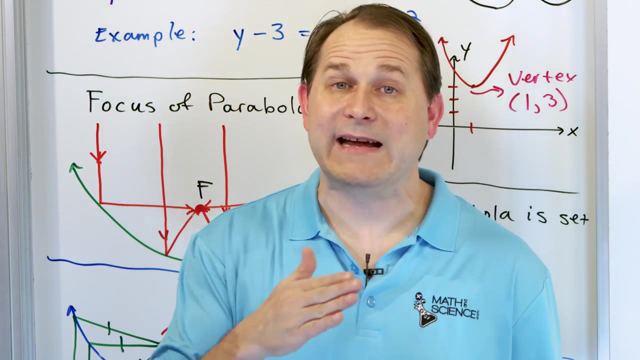 point on that curve is an equal distance to the focus as it is to the directrix. So every parabola has a directrix. Every parabola has a focus. And that's something you have to get in your head. When we first learn about parabolas, we don't talk about the focus or the directrix. So it kind of seems like we're adding it on. But in fact, every parabola 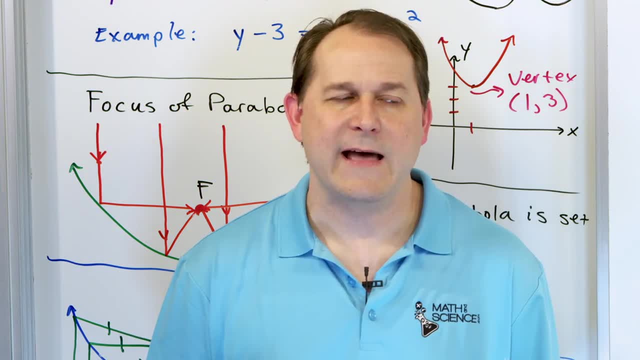 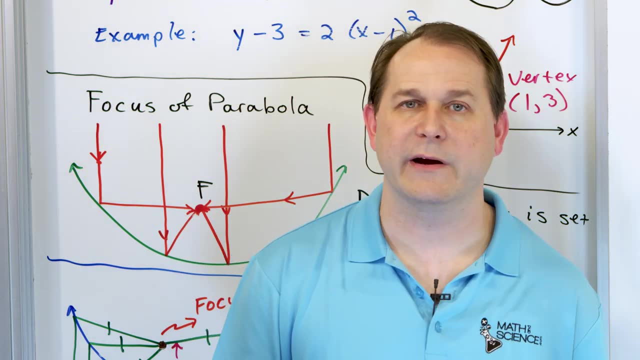 you've ever graphed always had a directrix. Even if you didn't know how to graph it, you can graph it. And they always had a focus, even if you didn't graph it. But here in these problems moving forward, we're always going to talk about the focus and the directrix as we graph and sketch all of these parabolas. So we have reviewed basically what we knew 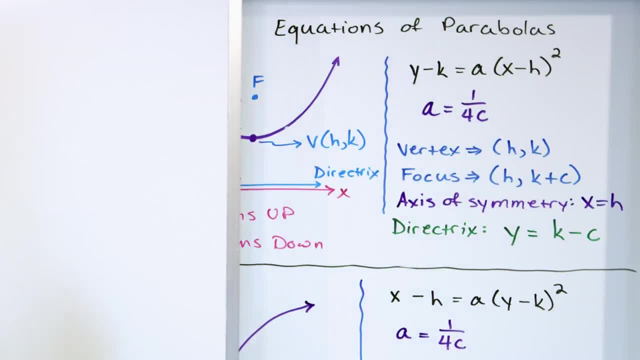 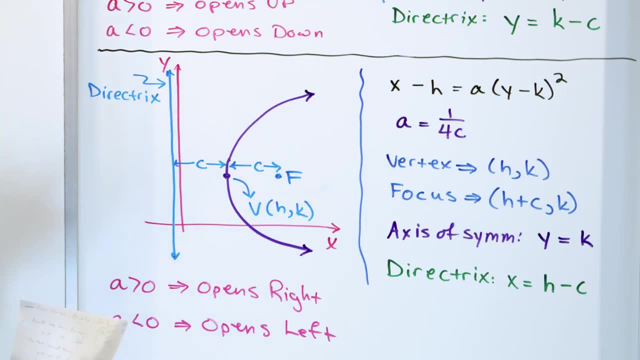 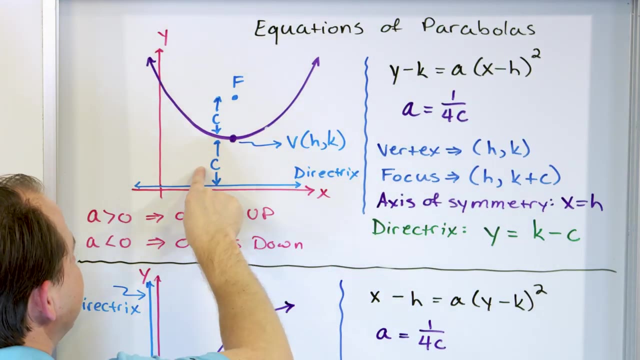 about parabolas. We have introduced the equations of a parabola, but I haven't really explained a lot about this because I need to talk about a few more things before I go into crazy detail here. But now at least you understand a little bit more that every parabola has a focus, it has a directrix, the distance c is here, the distance c is here. So the vertex is halfway 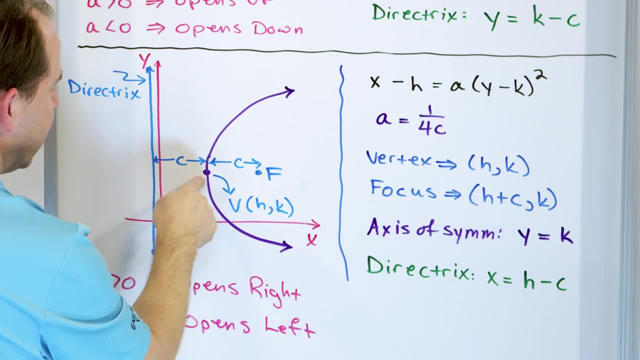 between the focus and the directrix. Same here. The vertex is halfway between the directrix and the focus for every parabola that we have. And so we've learned all of these things. 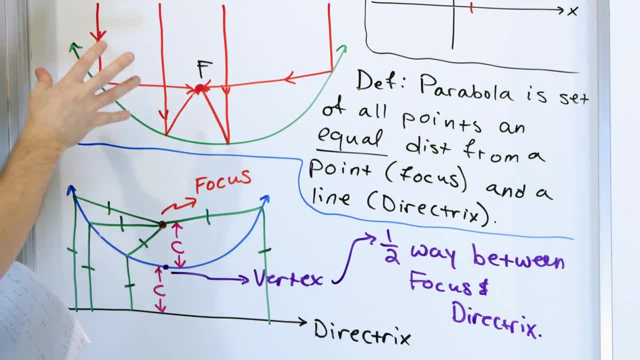 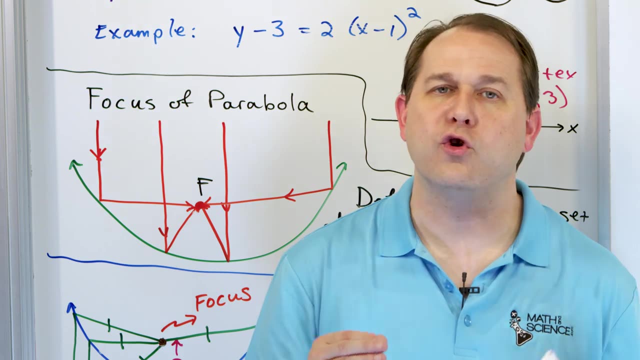 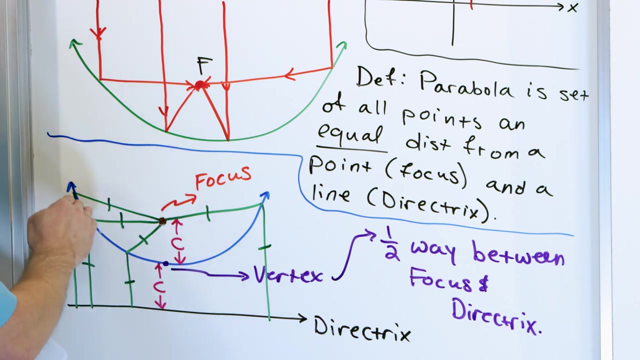 And then finally, we talk about this special property of a parabola, which allows it to focus incoming parallel rays to a point. And then we talked about the definition of a parabola, which we've discussed a lot so that you can get your brain wrapped around it. Now what we need to do is we need to derive the shape, the equation of a parabola. See, here's the geometric description. Here's a point we call the focus. Here's a line called the directrix. 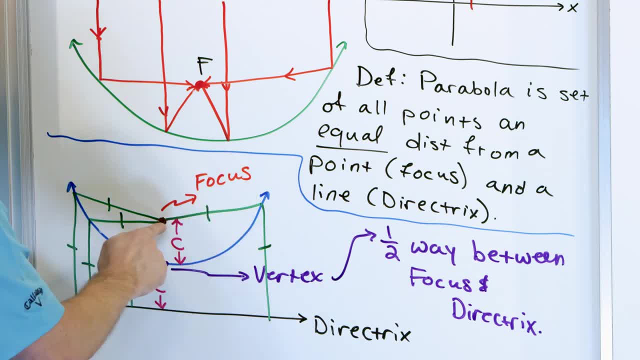 There has to be some blue curve called the parabola that every point on this curve is an equal distance from the point here to the focus and the point here to the directrix. 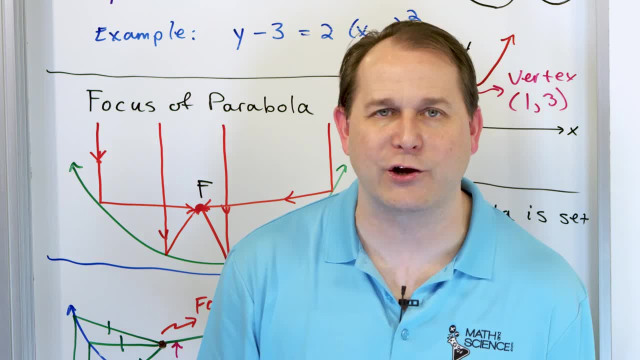 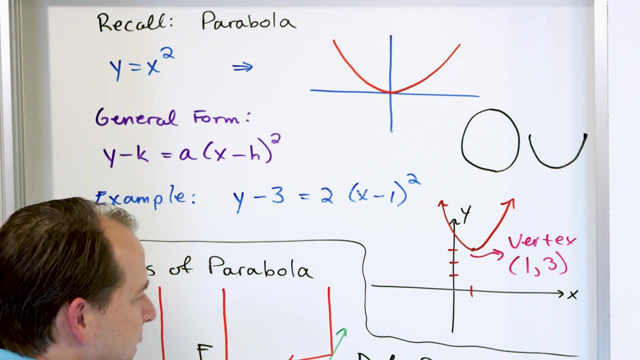 There has to be some special curve we call a parabola. What is the equation of that curve? Now you already know the answer. The equations of a parabola always look like this. But how do we go from the definition of the parabola to the definition of a parabola? Well, first, we have to derive the shape. So what we're going to do is we're going to derive the shape. parabola, which is all about geometry, to showing that really this thing is and does describe all 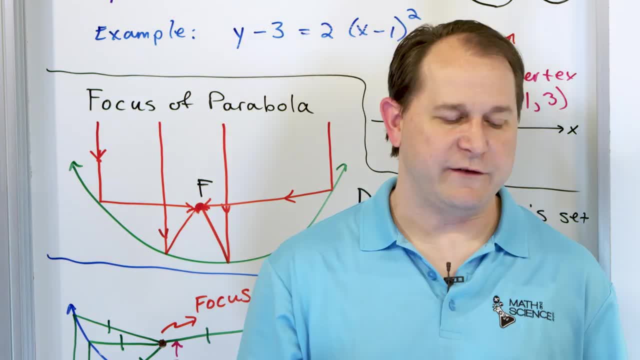 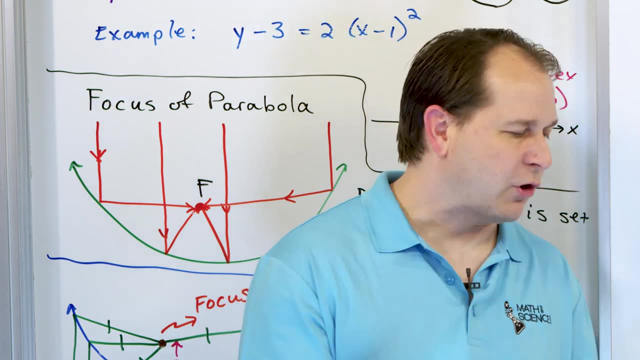 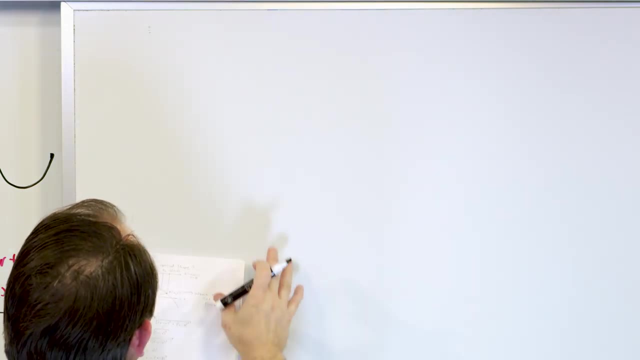 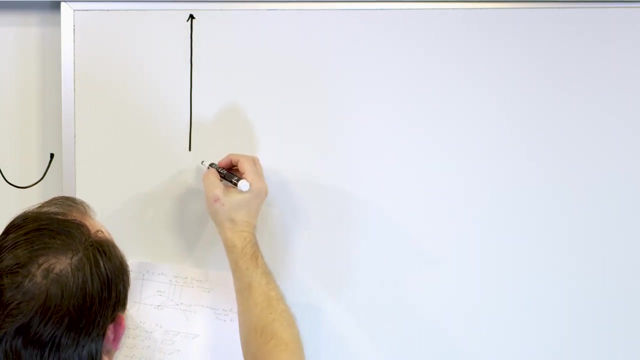 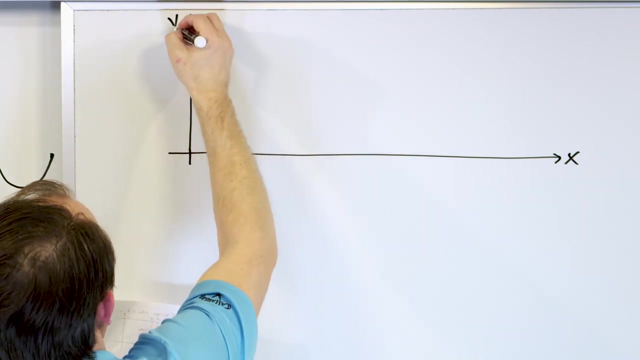 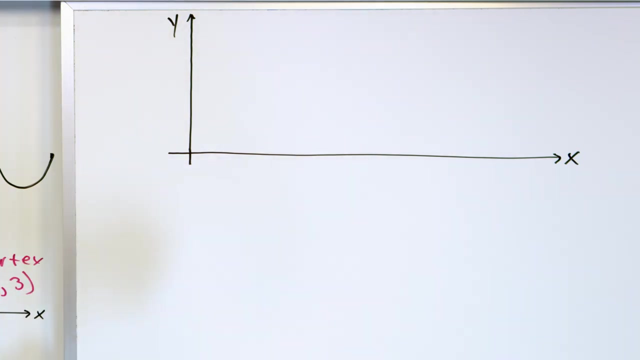 parabolas that you can graph. How do we know that? And so what we're going to do is we're going to go through a derivation of that. It's not hard. It's actually really easy to understand, but I do have to do some drawings here in the beginning. So we're just going to jump right into it. So what we have is we have to draw another sketch before we can derive the equation of a parabola. And this sketch I'm going to draw right at the top of the board. It's not going to be very long here, but I do need to get it on the board. So here we have the xy plane. I'm trying to give myself a lot of space down here to do the rest of the work. So here we have the xy plane. Now I have to pick some actual numbers. So what I'm going to do is I'm going to put the focus of this parabola at one, 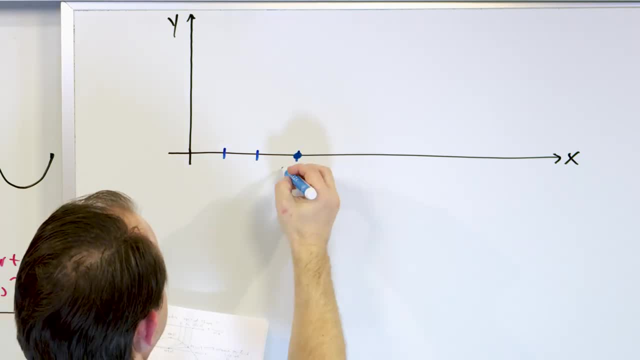 two, three units along the x-axis. So this thing is called the focus. It's at three. 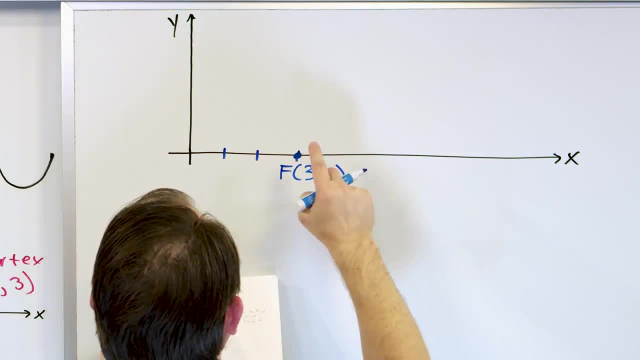 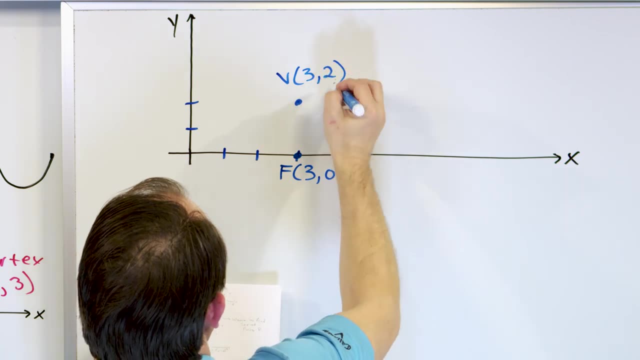 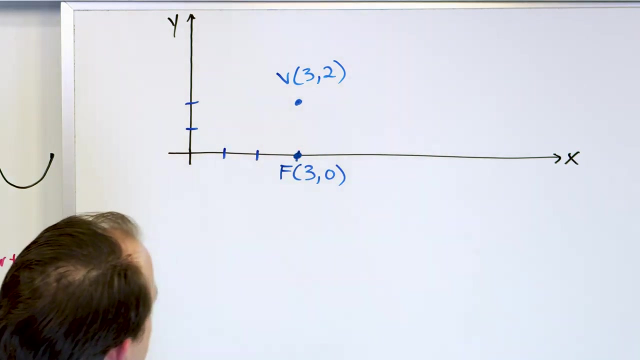 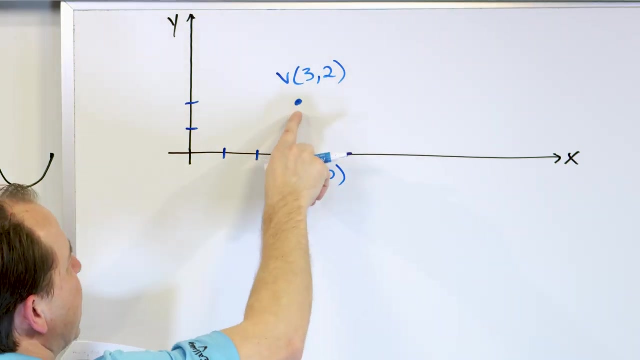 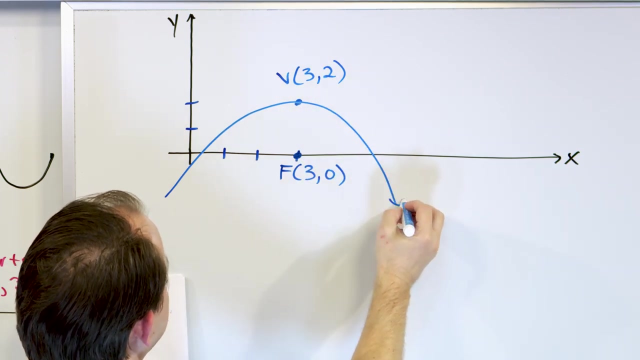 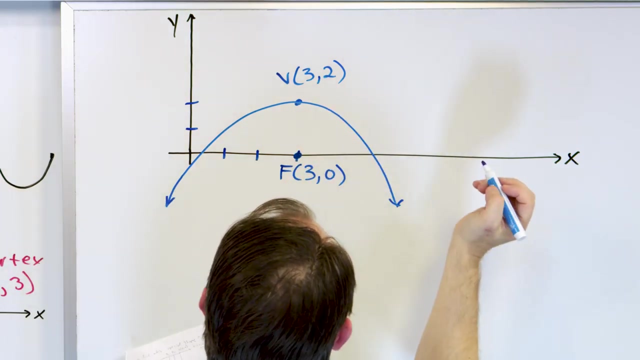 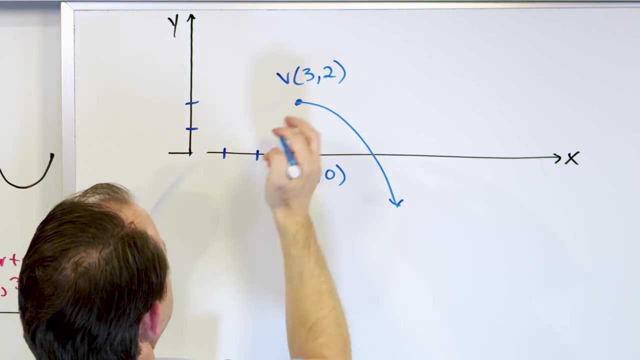 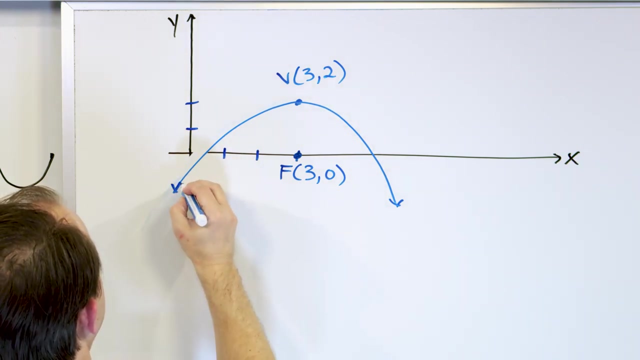 comma zero, right? And then I'm going to put the vertex at three comma two. So this is the vertex at three comma two. Now, because this is the vertex and because this is the focus, you know that the parabola has to be opening upside down because the focus is always kind of inside the parabola. The focus is always inside the bowl. So if the vertex is here and the focus is here, the only way the thing works is if it goes something like this. And I'm going to try to draw it upside down the best I can. Is this perfect? No, it's not. I can already tell this kind of opened up a little bit weird. But anyway, that's the basic parabola. This is the highest point of the... Actually, I'm looking at it again. It's completely lopsided. Sorry about that. Actually, let's try to fix it just a little bit. So it's going to go off something like this. Still not great. Sorry about that. Anyway, it's an upside down parabola that goes something like this. 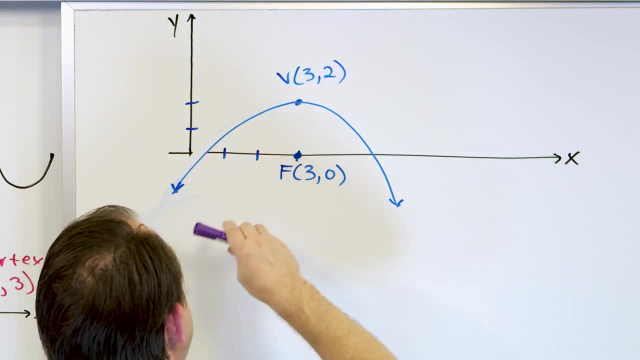 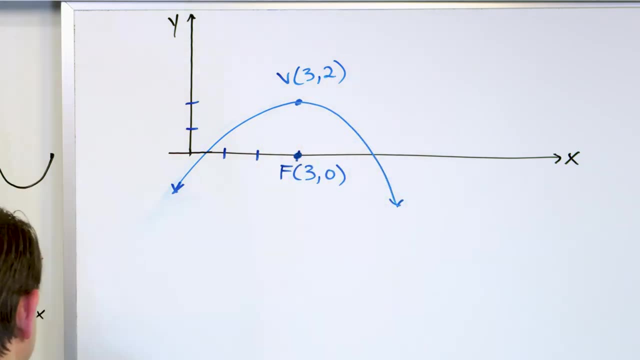 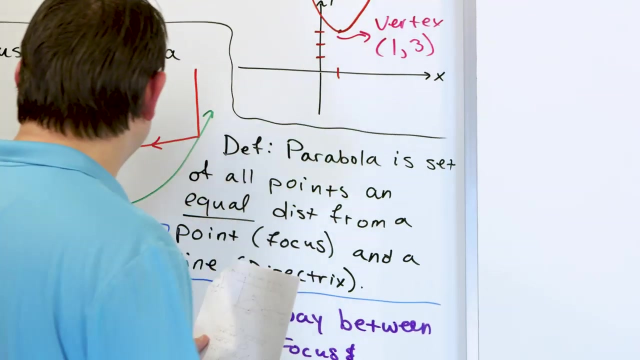 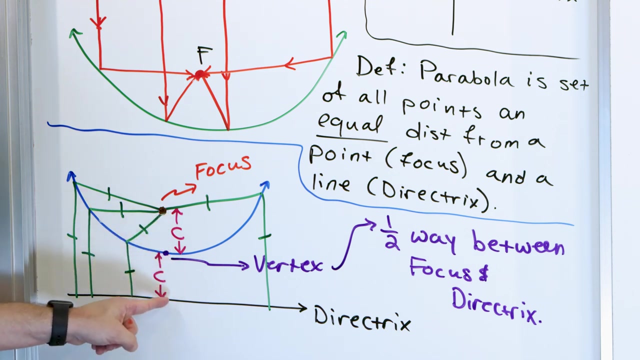 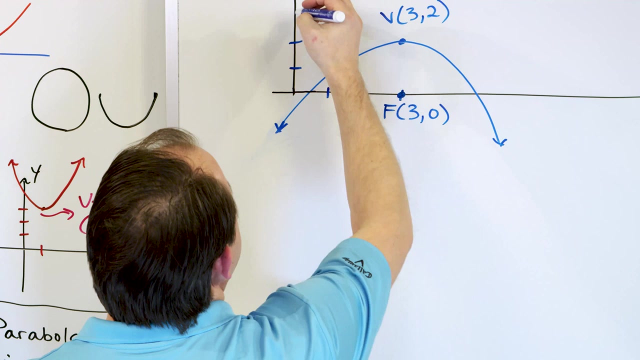 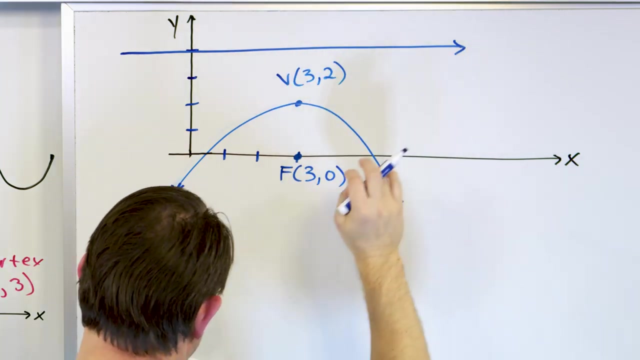 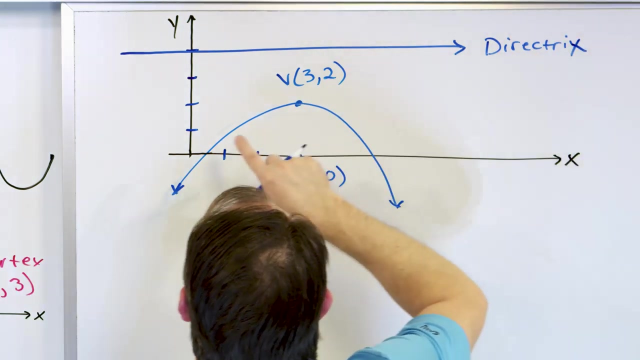 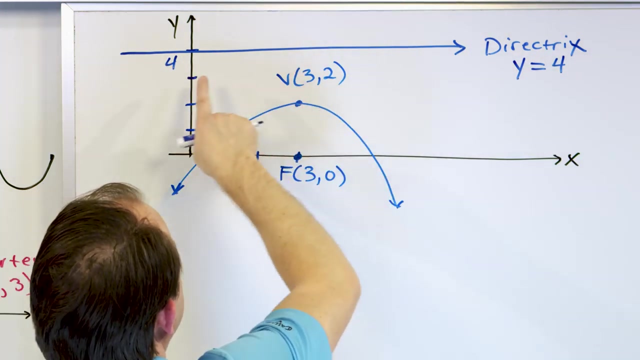 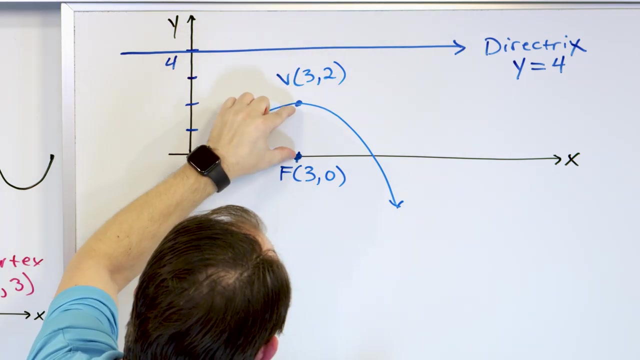 All right. Now, every parabola... It has a focus and every parabola also has a directrix. So let me ask you, if the focus is here and the vertex is here, where is the directrix of this parabola? The directrix of the parabola has to be on the other side, has to be on the backside. And also, we said that the vertex is always halfway between the focus and the directrix. So if the focus is here, the vertex is here, the directrix has to be the same distance away on the other side. So that means that we have... We have one, two. So this is three, this is four. So that means there needs to be a horizontal line up here. This is going to be the directrix. I'm going to write this directrix. And what is the equation of this directrix? Well, this is one, two, three, four. So this equation of the directrix is y is equal to four. It's a horizontal line, four units up like this. How do we know the directrix is actually there? It's because the vertex always has to be in the middle. So if this is two units, then this has to be two units. 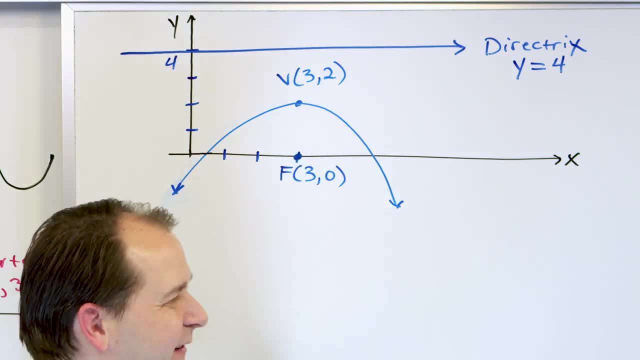 And so when we lock down the vertex, we know where the directrix is. A lot of these problems in algebra are always going to be like, tell me where the vertex is. And you'll just have to know 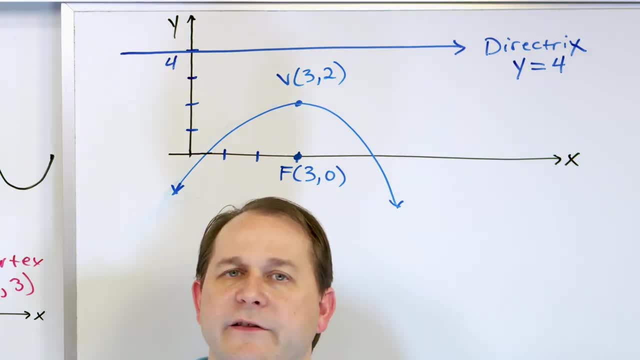 how things are set up. They're at equal distance on either side of the vertex or whatever to write the equation of the directrix down, which is what we did right here. All right. So what we need to 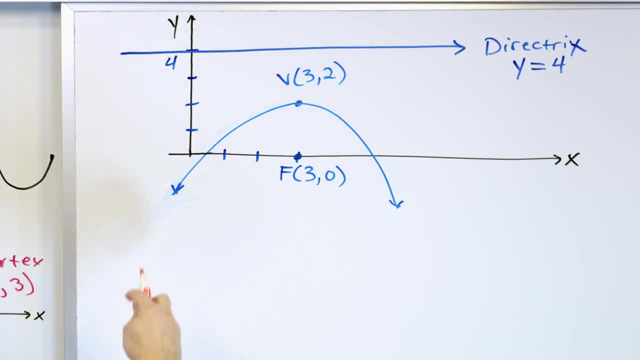 do is we need to realize that this blue curve is a bunch of points, right? It's a bunch of points. 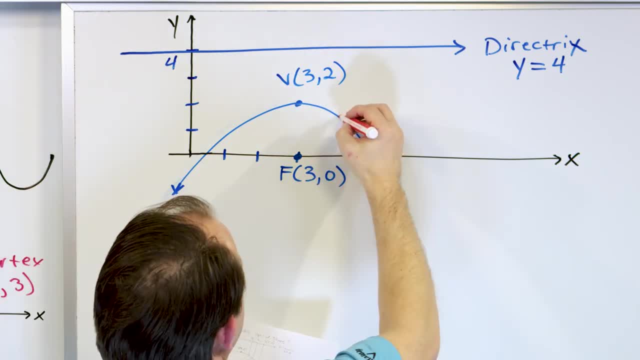 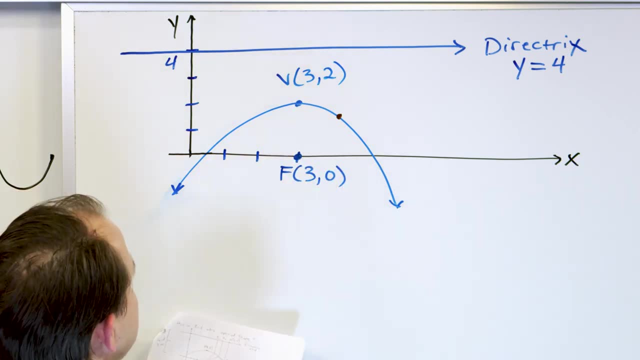 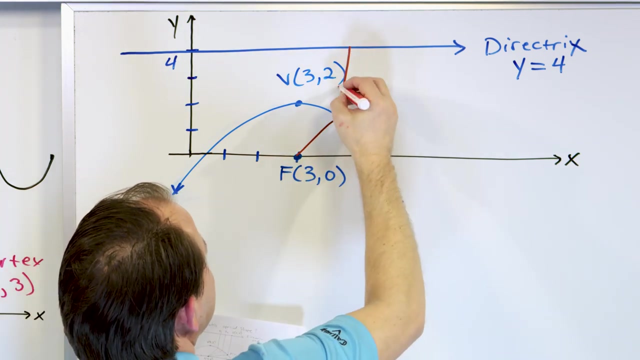 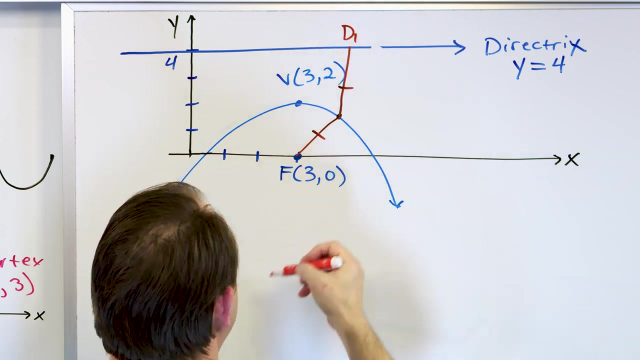 What we're saying is that this point, for instance, right, whatever this point is right here, I don't know exactly where it is. It's over here and it's up here. But there's some point right there in the curve of the parabola, right? But I do know one thing, and that is the distance from here to here to the focus is the same as the distance up like this. And I'm going to put little lines to show me this. So this line here, d1, is the point on the directrix right there. And what I'm saying is 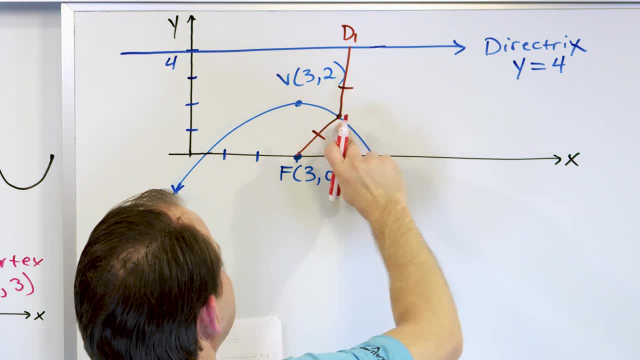 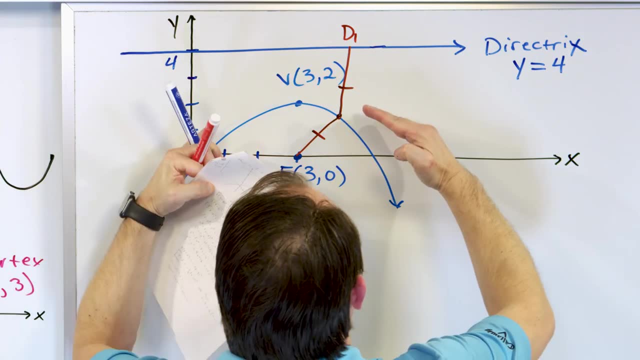 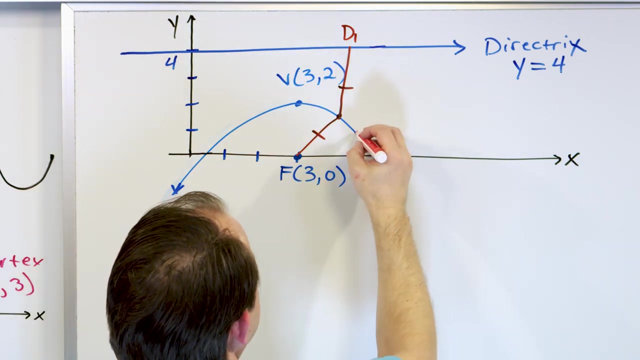 between this point and the line directrix is the same as the distance here to here. Now, I can tell you that they don't look the same because I'm drawing it freehand. But if you could imagine that I opened my parabola up a little bit more and it was an exact shape, then it would exactly be correct, right? And then if you want to pick another point, let's say this point right here. 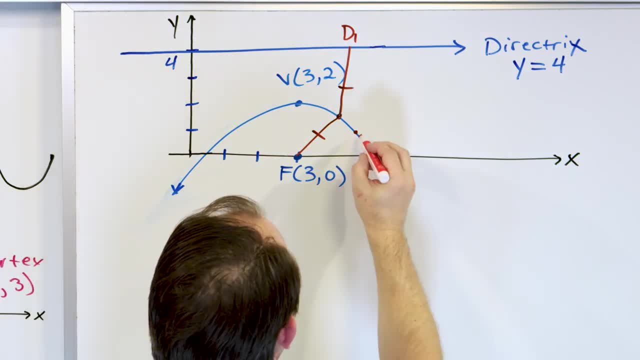 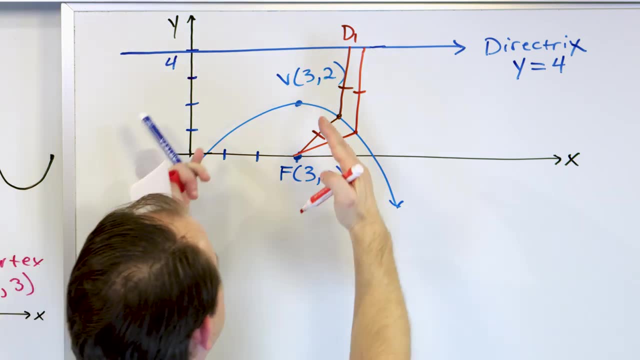 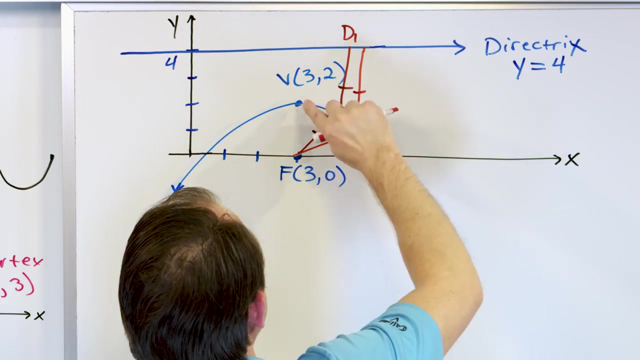 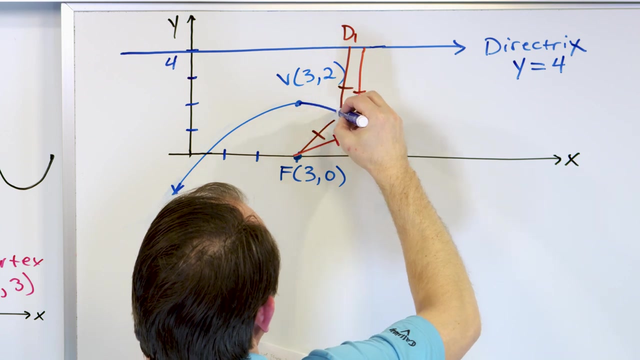 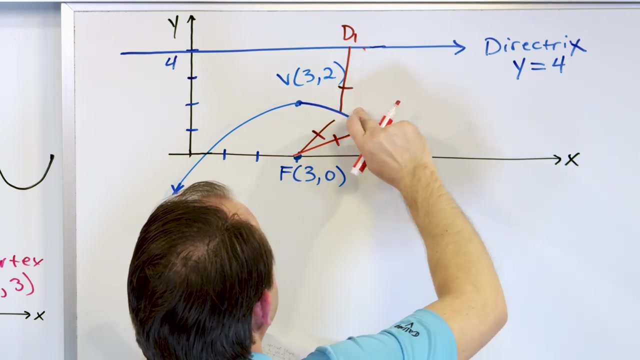 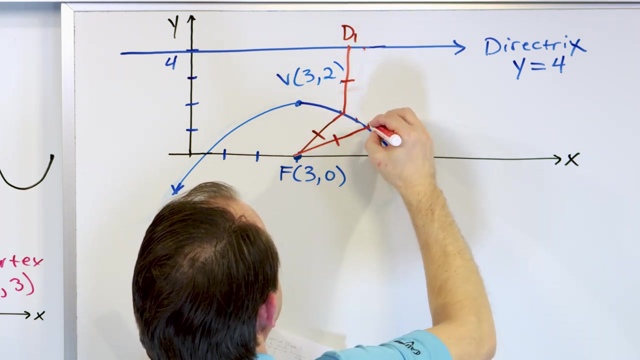 And this one even looks even worse, actually. You can see because this one here, what I'm saying is the same as the distance up there as well. It doesn't look the same, and that is just because parabola is really just too, it's too crunched in. It's not a real parabola shape. So if I wanted to fix it, I could erase this, and you know, we could do that if you want. Does it really matter too much? No, but you know, why not? Let's just open it up just a little bit more, something like this. That's probably a little bit closer. Is it still exact? No, it's not exact, but it's pretty close. So let's go and do something like, let's try to erase this a little bit. So the distance here to here is the same as the distance here to here. The distance here to here is the same as distance here to here. That's pretty close. 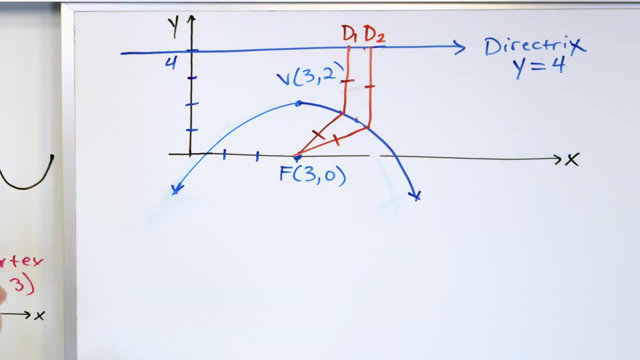 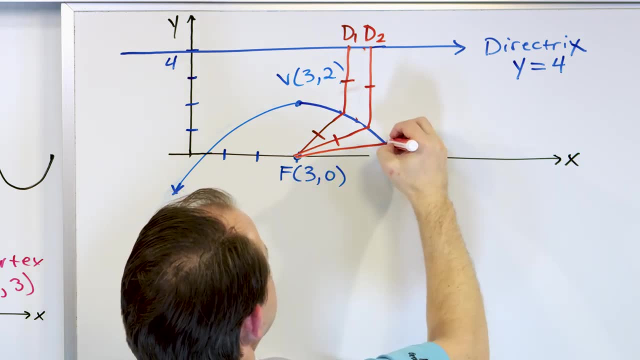 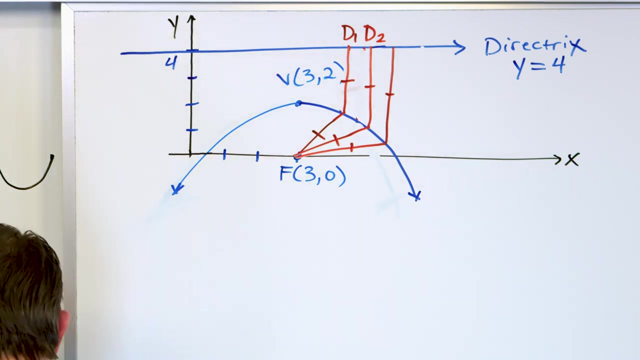 And we'll call this point D sub 2, because that's where it hits that line. And we'll call, we'll do one more point, this point here. The distance between here and the focus is the same as the distance up there to the directrix. So those lines are there. And then this one I'm going to label as an actual point. I'm going to label this one right here. I'm going to call it 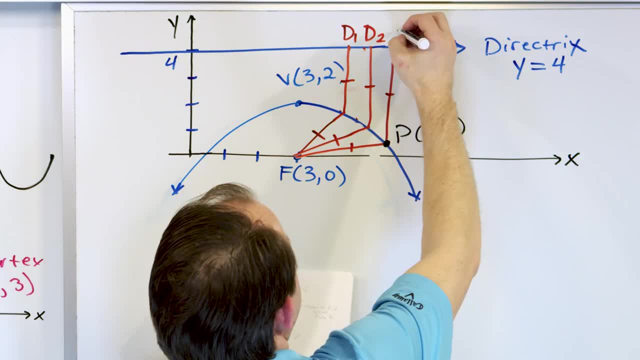 PX comma Y. And then up here, this D that's going to be the point on the directrix is at X comma 4. 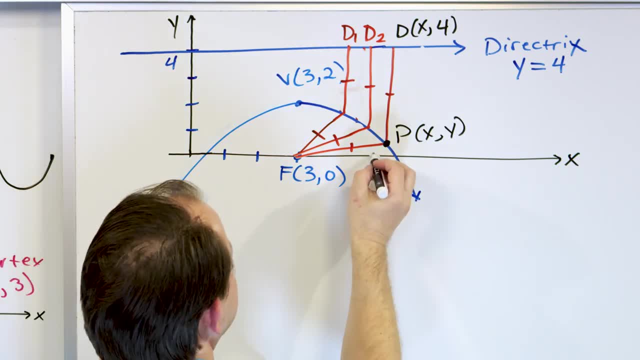 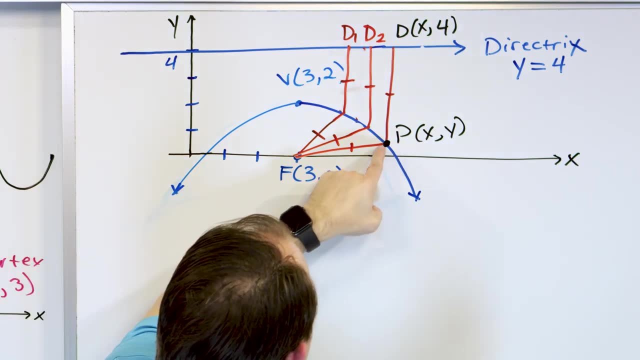 Now, I need to explain what I'm talking about here because pretty soon I'm going to use this in an equation. What I'm saying is the focus is a lockdown point at 3,0. The point on the parabola is just some xy location. 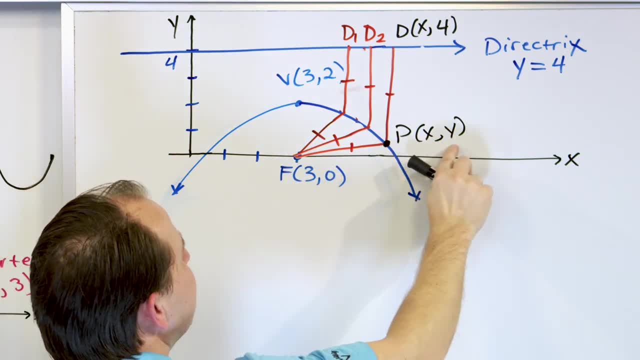 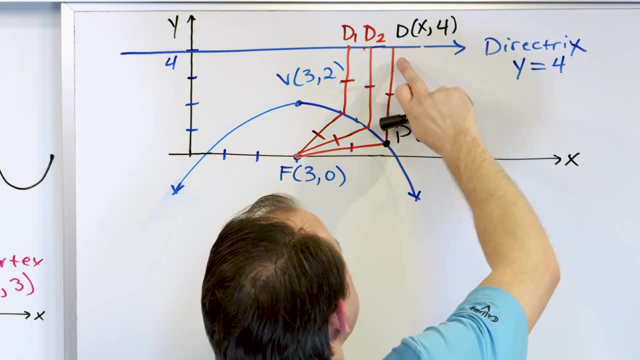 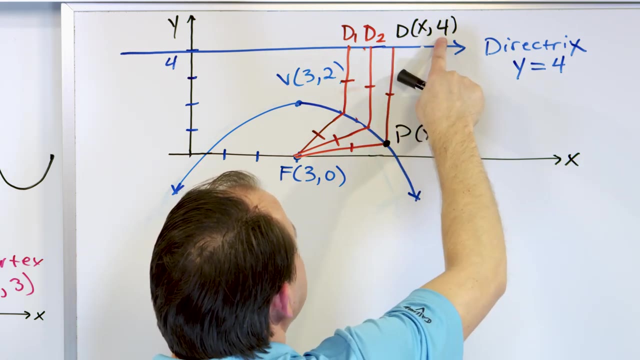 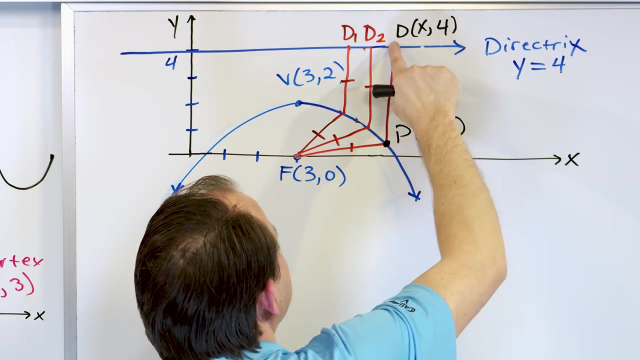 If I look at all these points here, they're all at different xy locations. I don't know what this point P is because I don't know the shape of the curve yet, but it's at some xy location. This point here is the same x value as the point because it's straight up. That's why x is the same here, but it's 4 units in y. That's why I had to put the number 4 here. So it's at x, 4. In other words, the point where I intersect here is at whatever the point is here, x, 4 units up. 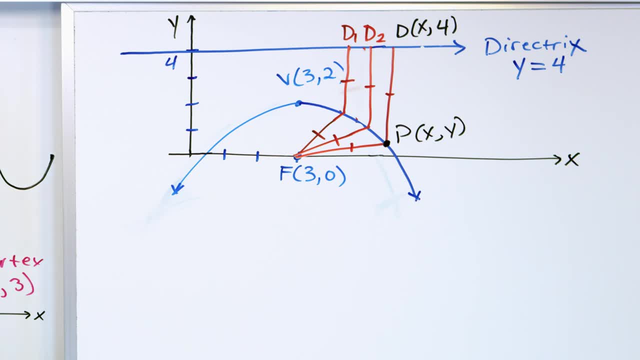 Now, why do I spend all of this time writing this stuff down? And that is because what we need to do is figure out the equation of this parabola. 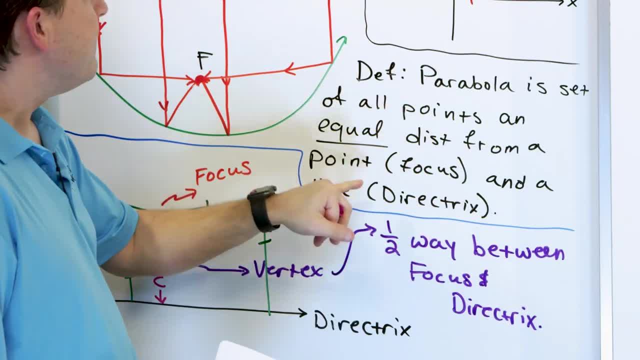 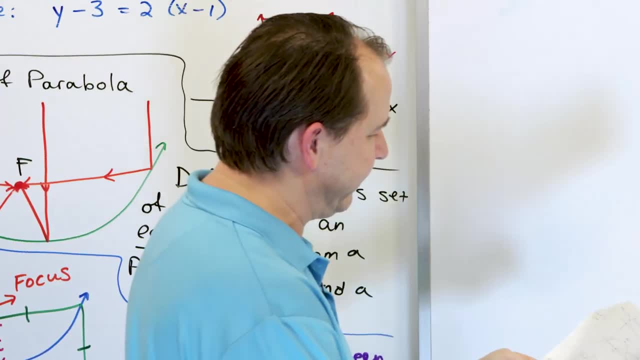 We want to derive this thing. And we know that the definition means that the distance from every point on this parabola to the focus, and also to the directrix, is the same distance. 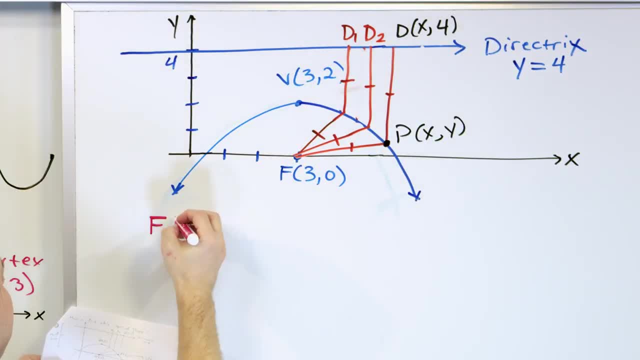 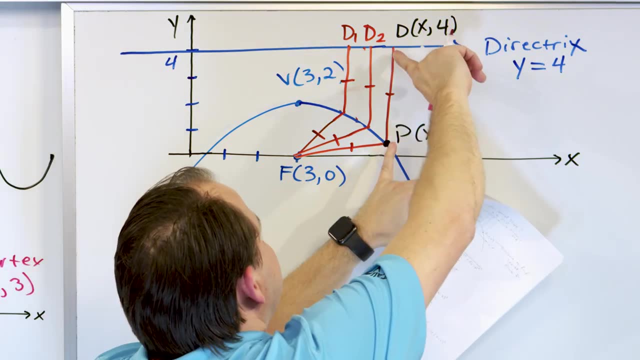 So that means if this is point F, the distance between F and P is the same thing as the distance between P and D. This distance is the same as this distance. This distance is the same as this distance. This one is the same as this one. This one is the same as this one. This one is the same as this one. 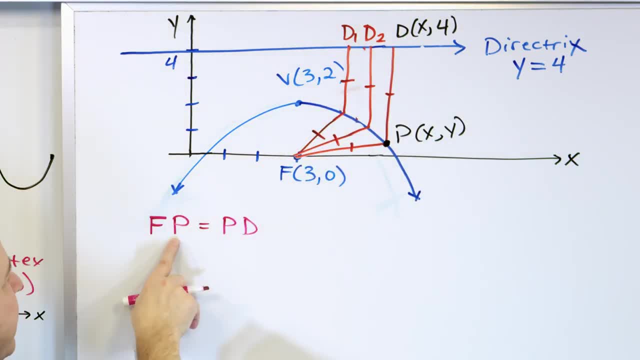 Every point I pick on this parabola, then the distance from the focus to the point on the parabola is the same as from that distance from that same point to the directrix. Fp is equal to Pd. 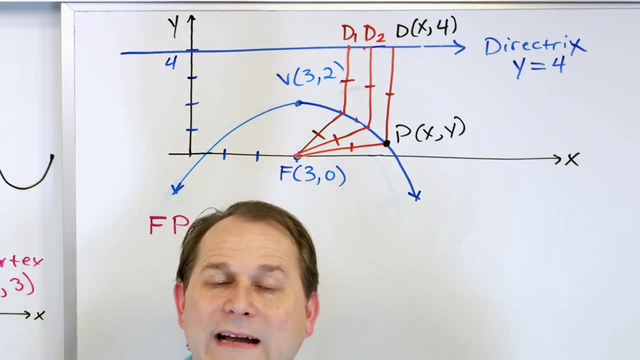 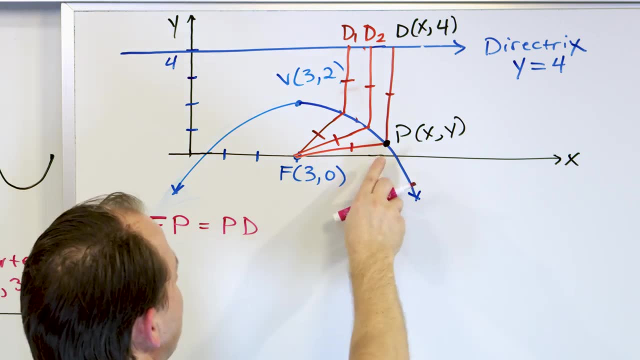 Now, we've learned, fortunately, about the distance formula. We know how to calculate distances between any points in space, right? So what is the distance, Fp? Well, we have to use the distance formula. We know this is x, y, and this is 3, 0. So let's do the distance formula. 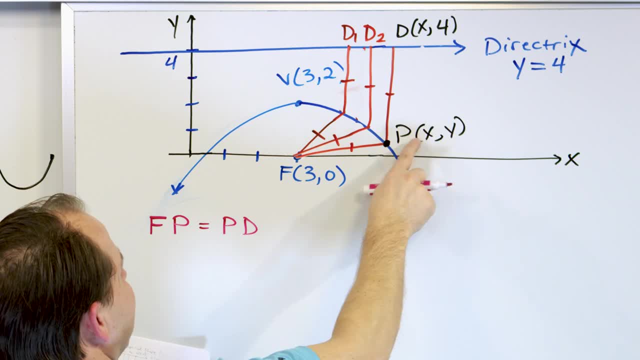 It's going to be the difference in the x values. So we're going to go x minus 3, quantity squared, plus the difference in the y values, y minus 0. Quantity squared, square root of this. 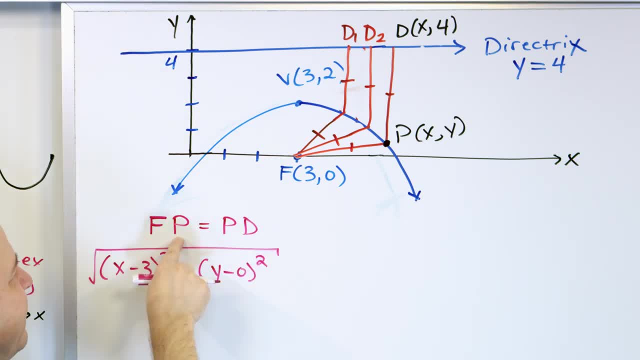 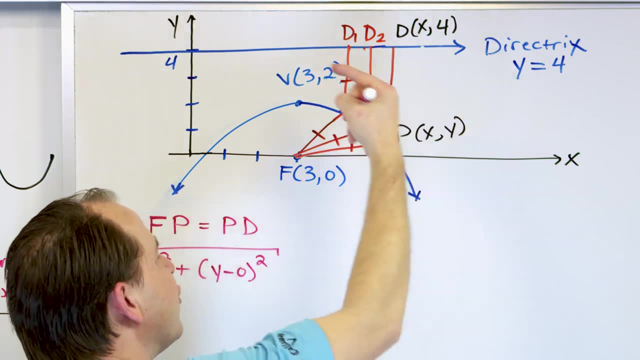 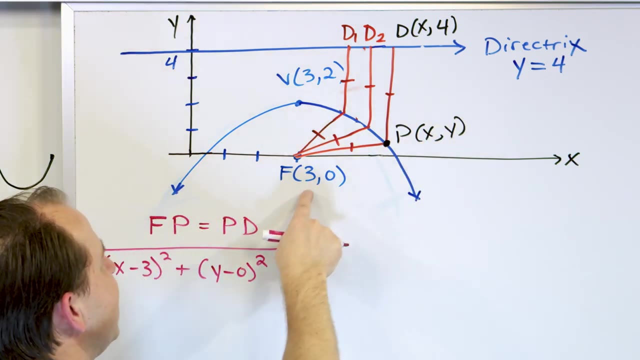 This is nothing more than the distance formula. It's calculating the distance between F, the focus, and this particular point right here. I don't know what the coordinates are. I'm going to create an equation to figure out what these coordinates are. That's what I'm trying to do, but I don't know what they are now, so I just take it as x comma y. Difference in the x values squared, difference in the y values squared, square root of the whole thing. 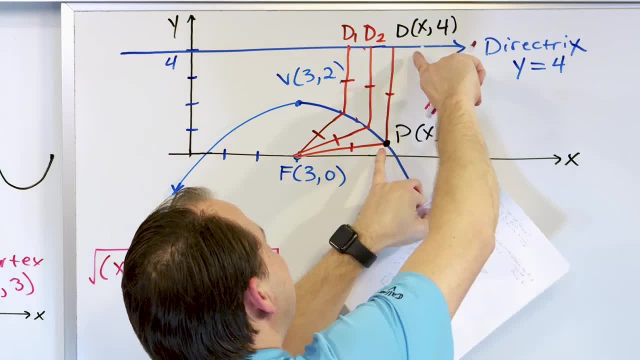 This is the distance here. But I know that this distance has to be the same as this distance. 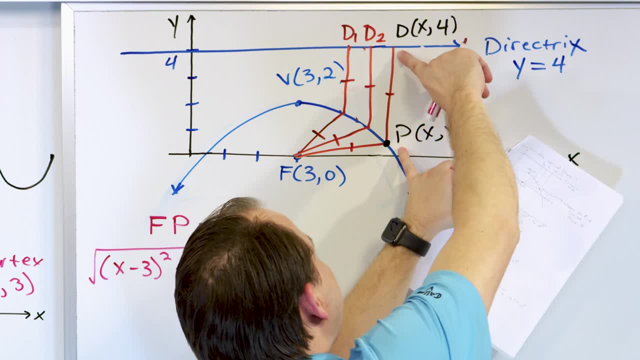 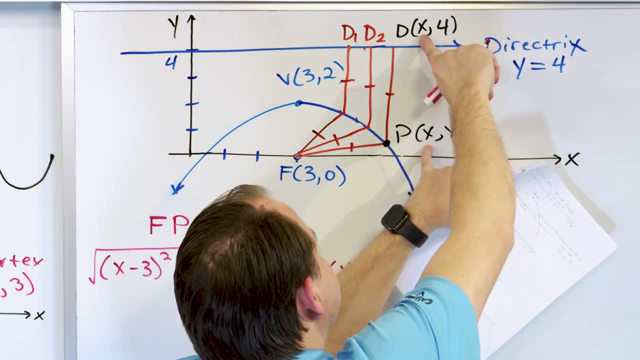 So I have to put an equal sign, and I'm going to now calculate the distance between these two points. Again, the difference of the x coordinates is x minus x squared. Notice the x coordinates are the same. 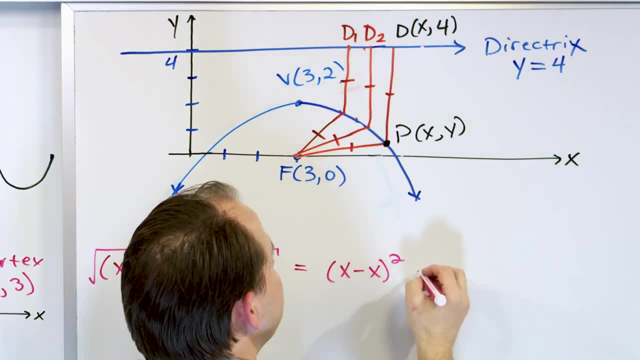 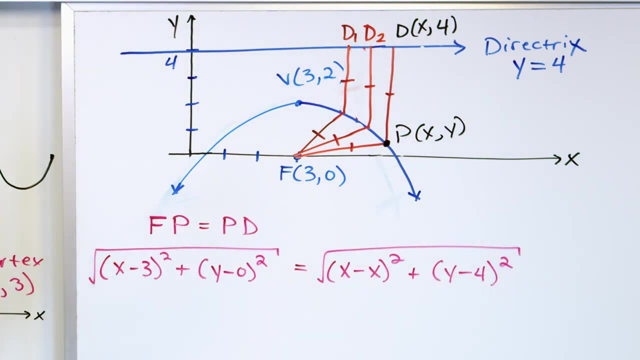 And then the difference in the y coordinates is y minus 4, quantity squared. It is crucial that you understand this equation on the board, because what's going to happen is we're just going to spend the rest of this time simplifying it. 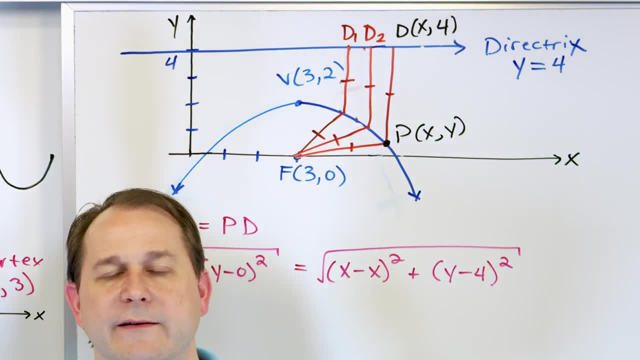 And then it's going to end up showing us that this equation of a parabola is correct. So what we have here is the distance between f and p, just the distance formula. 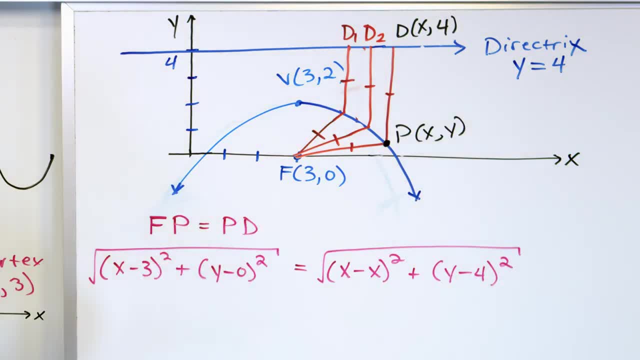 The distance between p and d, this is just the distance formula. Alright, so let's crank through this. 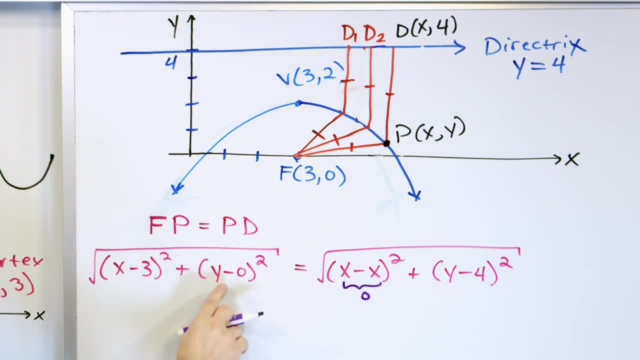 Now, we know that x minus x is going to give us 0 squared. We know that y minus 0 is easy as well. So we're just going to rewrite this. x minus 3 quantity squared plus y squared, because the 0 doesn't matter. We still have a square root. This is just 0 squared. It disappears. So you're just going to have y minus 4. Quantity squared. We're going to have the square root of this whole thing. 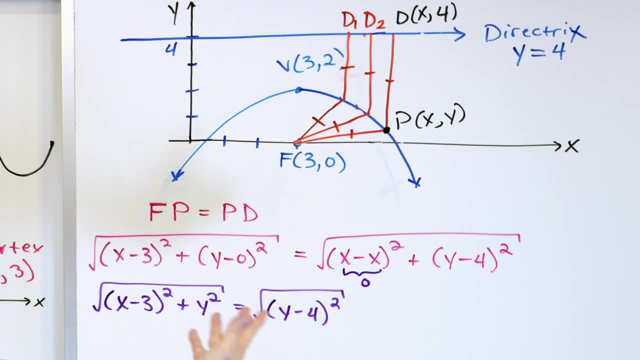 Alright, so all we did was simplify this. Now, how do we go any farther? 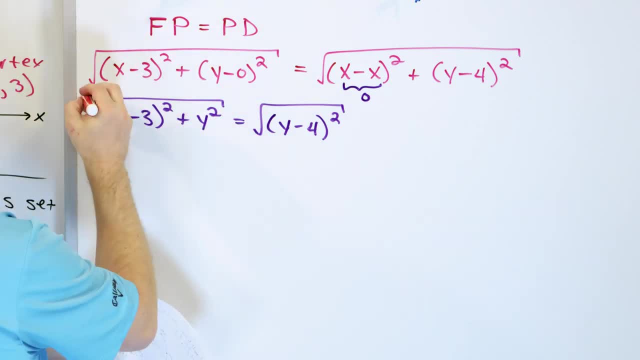 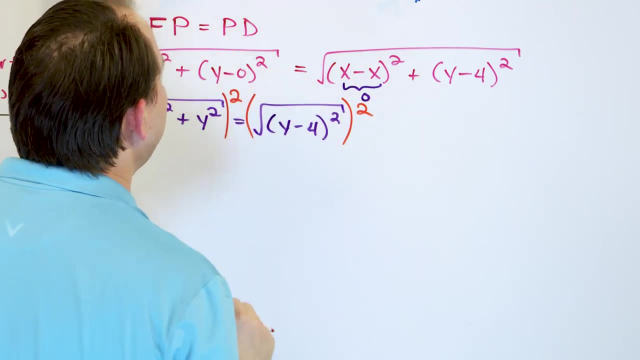 We have a square root on the left and a square root on the right. So we're just going to take and we're going to square the left of this equation. And when we do that, then we also have to square the right-hand side of the equation. This square is going to cancel with the square root. 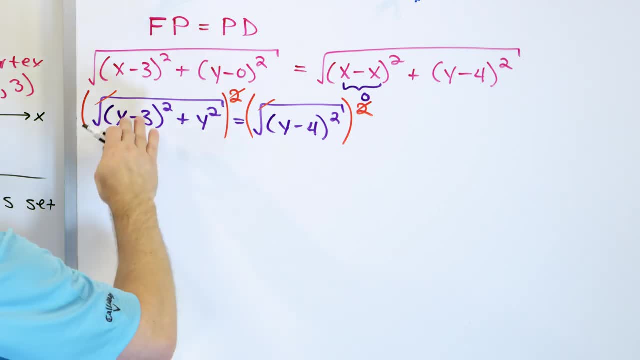 This square is going to cancel with the square root. And so what I'm going to have after I do that is just what's underneath. 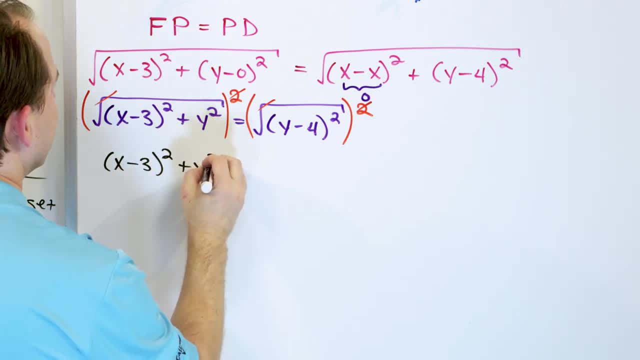 x minus 3 quantity squared plus y squared is y minus 4 quantity squared. And so now you can see I'm not quite there, but I'm getting it closer to what an equation of a parabola might look like. 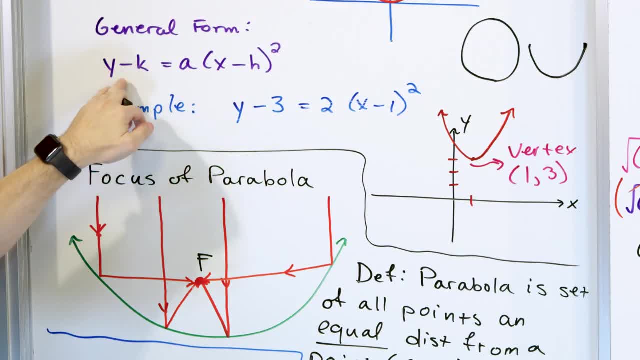 So when you look at the actual answer, you see the y value is on the left and the x values are on the right. So let's take all the y values and move them to the left and all the x values and move them to the right. 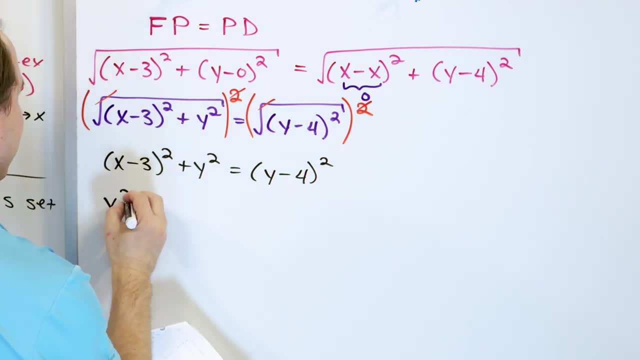 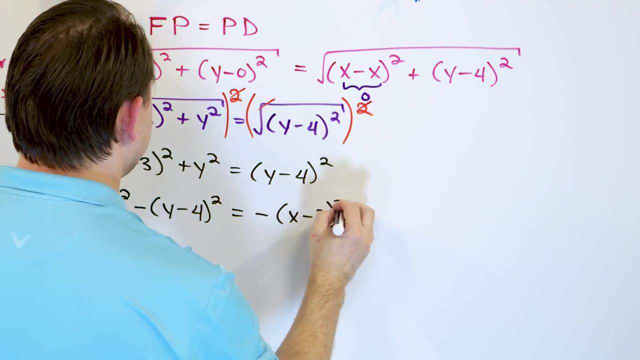 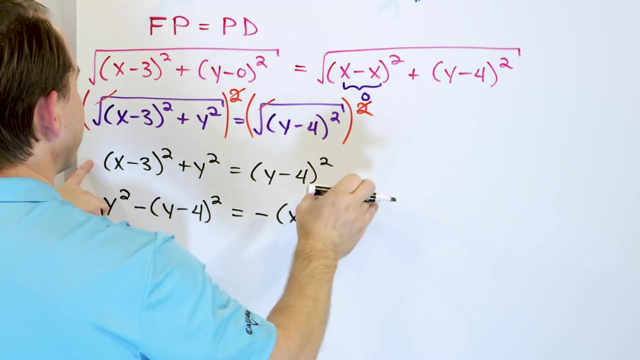 And so what we're going to have is when I do that is I'll have y squared minus y minus 4 quantity squared is equal to negative x minus 3 quantity squared. Make sure you understand I'm holding this the same. I'm subtracting this to get it to this side and I'm subtracting this to get it to the right side. So that's why there's a negative in each location. But I have all of the y's on the left and all of the x's on the right. All right. 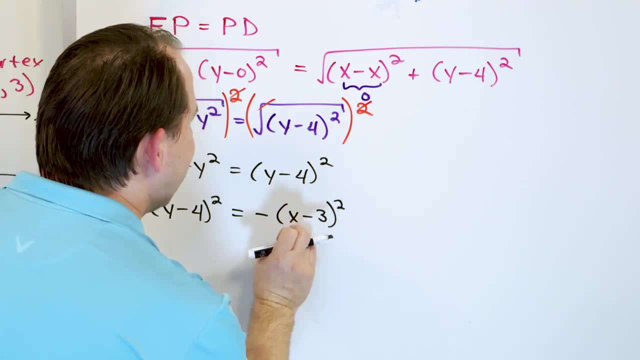 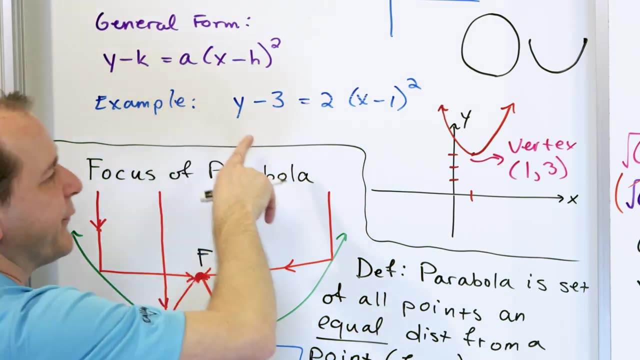 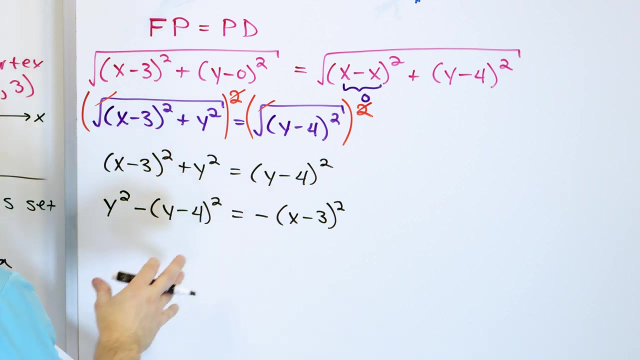 So notice the right-hand side of this equation is x minus 3 quantity squared. That's what a parabola should have. x minus something quantity squared. And there should be a number out in front. In this case, the number right now is negative 1. So actually the right-hand side looks good. The left-hand side doesn't look good. It's got too many squares and other things going on. So what we have to do is expand this. 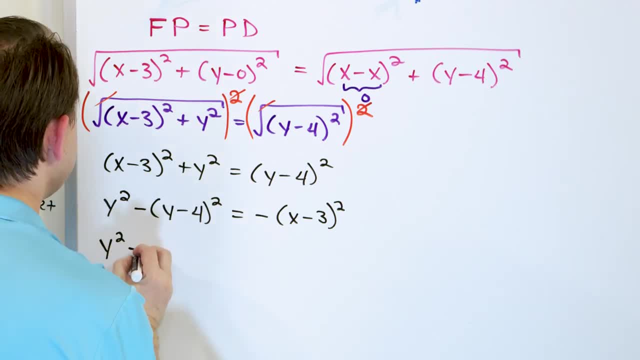 So the way you're going to do that is y squared minus and then what you're going to have is y minus 4 times y minus 4. 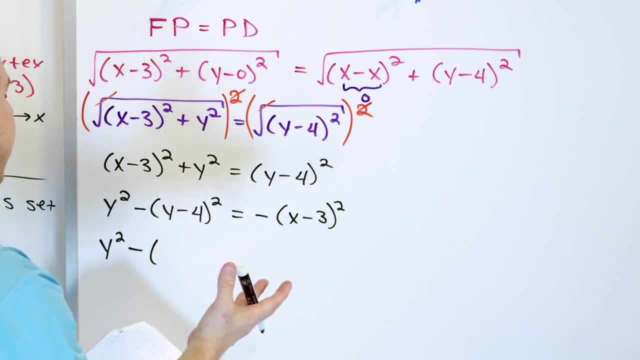 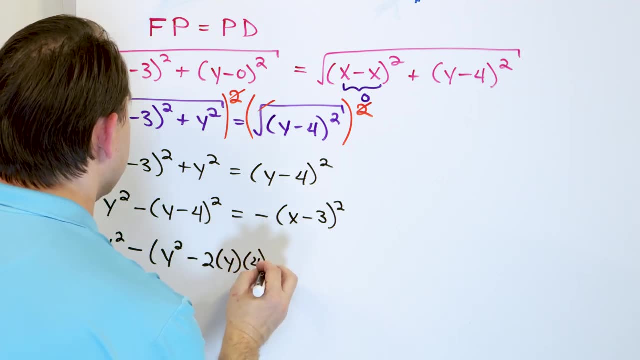 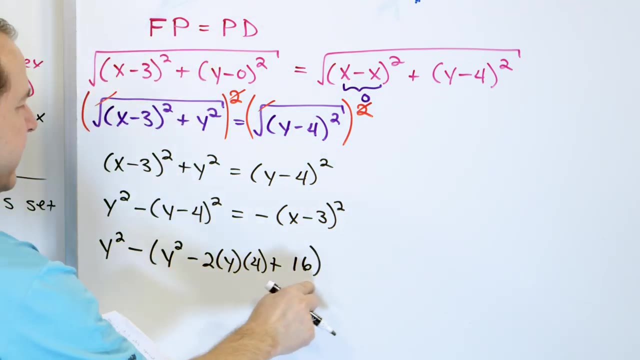 So we're going to use the binomial squaring stuff that we've done in the past. We're going to take the first thing squared. y squared minus 2 times y times 4 plus 4 times 4 is 16. And so we just squared this. 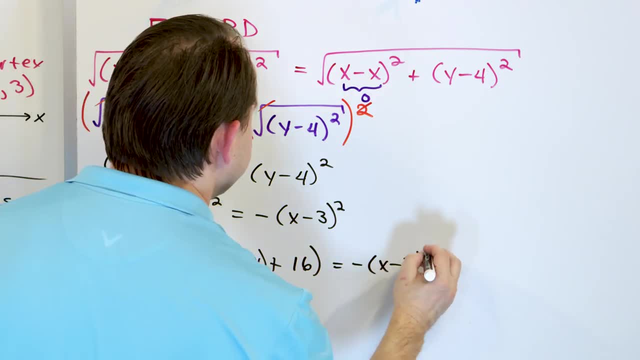 And then on the right-hand side, we'll have negative x minus 3 quantity squared. Okay, let me just catch up, make sure I'm correct. So then we're going to simplify further. 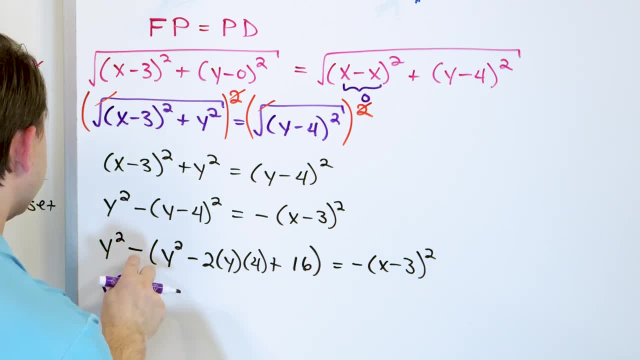 We're going to say, well, what we're going to have is y squared. This negative is going to multiply in making this negative y squared. This negative multiplies in making this y squared. This negative multiplies in making it positive. 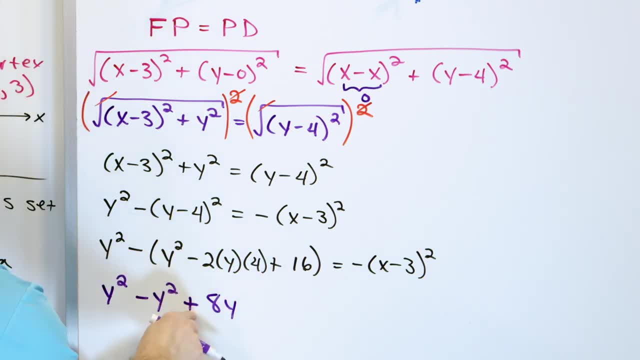 But this is 2 times y times 4, so it's going to be 8y. Negative times negative is positive. Then we have negative times this gives negative 16. 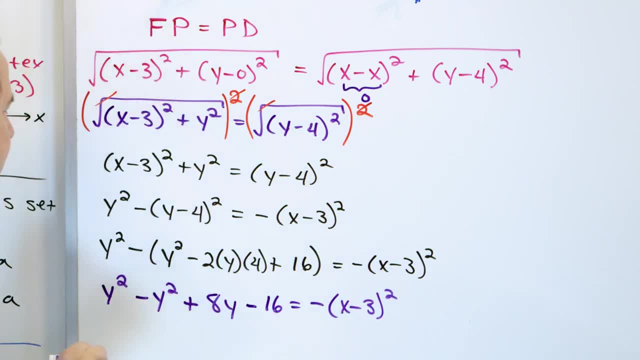 And then this is x minus 3 quantity squared like this. Now notice we have y squared minus y squared. 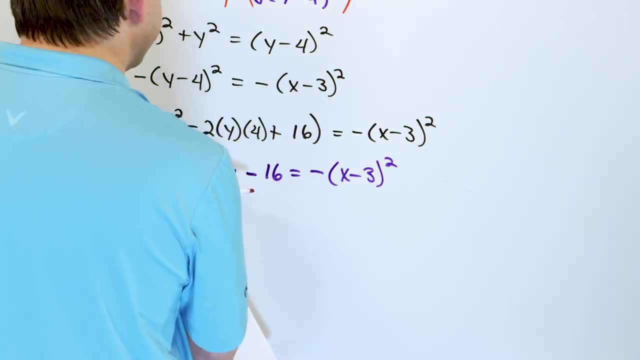 This goes to 0. That disappears. And then on the left, we have 8y minus 16. 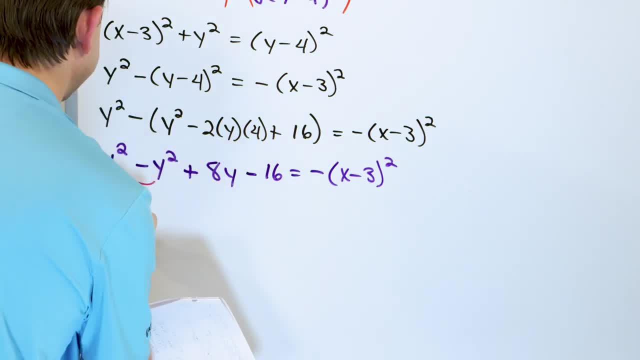 What we want to do is factor out the 8 because we have an 8 and a 16 here. We want to factor out the 8. 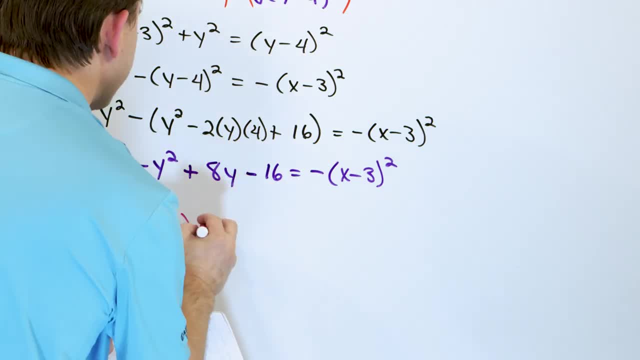 And you have y minus 2 on the left because 8 times 2 is the 16. 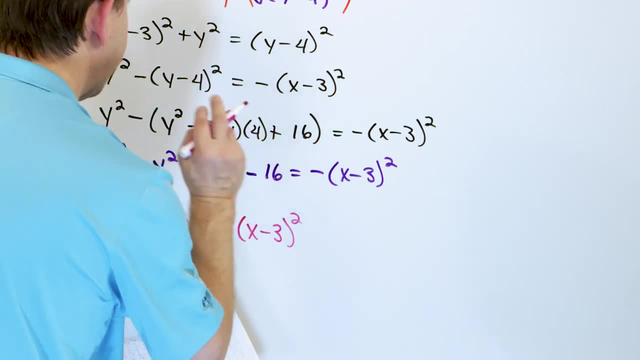 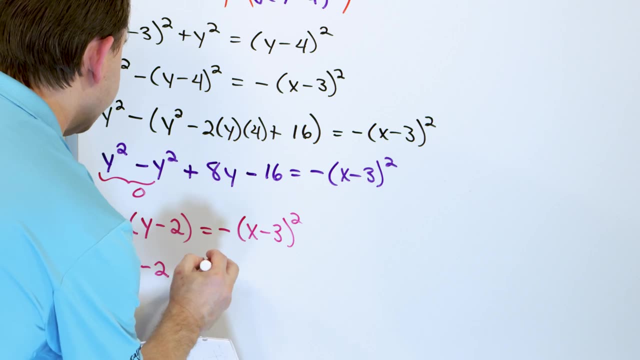 On the right-hand side, you'll have negative x minus 3 quantity squared. And then let's divide by the 8. So we're going to be left with y minus 2 is equal to negative 1 eighth because I'm going to divide both sides by 8 x minus 3 quantity squared. 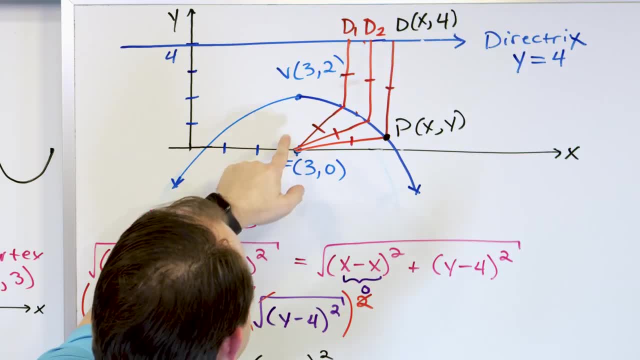 Now look at what we have done. All we did was draw a picture and we said the distance from any point on this path, 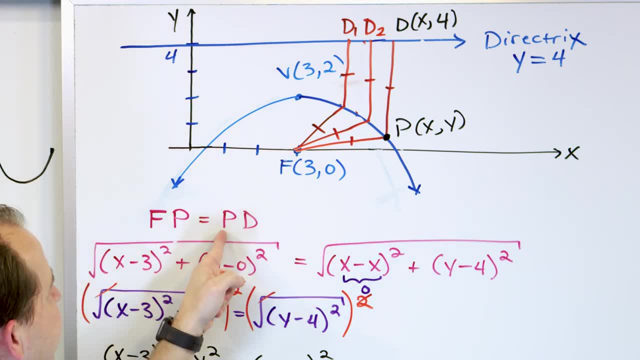 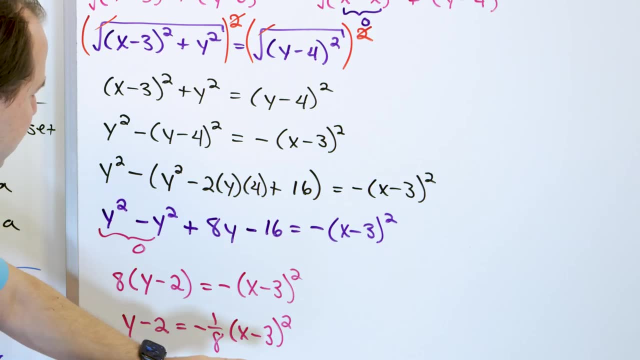 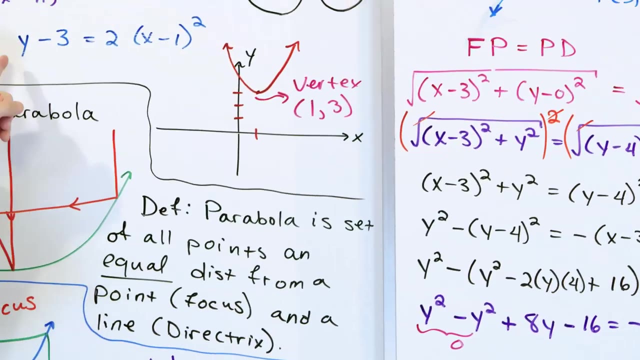 x minus 3 to the focus, is the same thing as the distance from the point to the directrix. We did the distance formulas and then all the rest of it was just simplifying and we end up with this. This looks like the equation of a parabola. y minus 2 is negative 1 eighth x minus 3 quantity squared. The example we gave here is in the same form. y minus something is a constant times x minus something quantity squared. 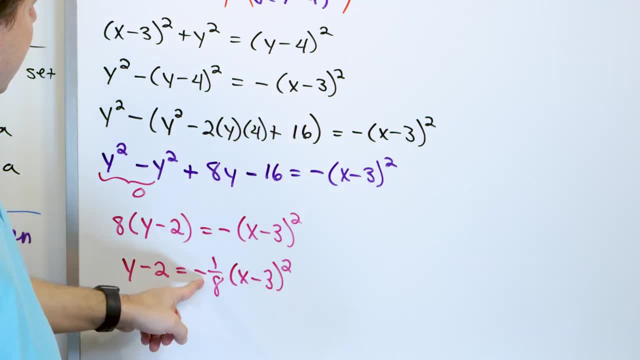 In this case, we have the constant in front that's negative. So that's why it opens upside down. 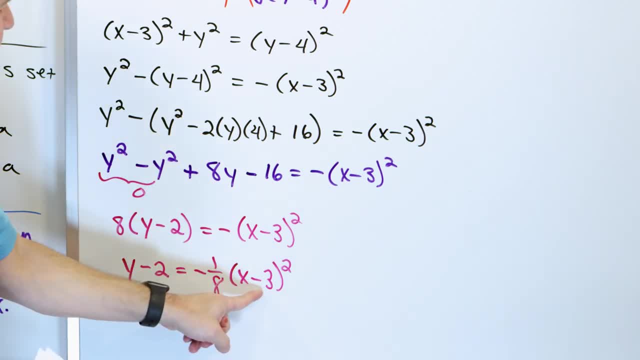 We have a shift that's 3 units to the right. The vertex would be 3 units to the right and 2 units up. So 3 units to the right, 2 units up. 3 units to the right, 2 units up. That's where the vertex is of this thing. It opens upside down. This is the equation of this parabola. 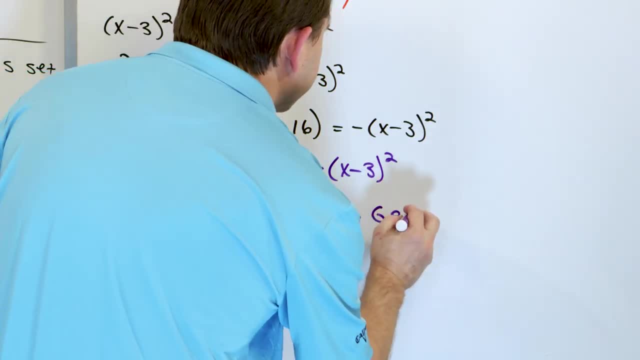 So from this you can generalize. And you can say that in general the form is of y minus k. 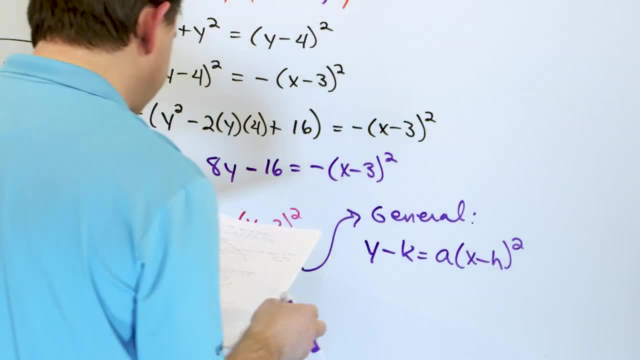 It's a x minus h quantity squared. 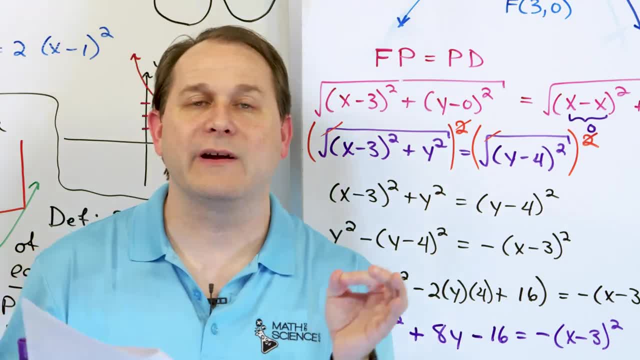 So what we have done is we've figured out from the geometric definition of what a parabola is, the set of all points and equal distance to the focus as it is to the directrix. 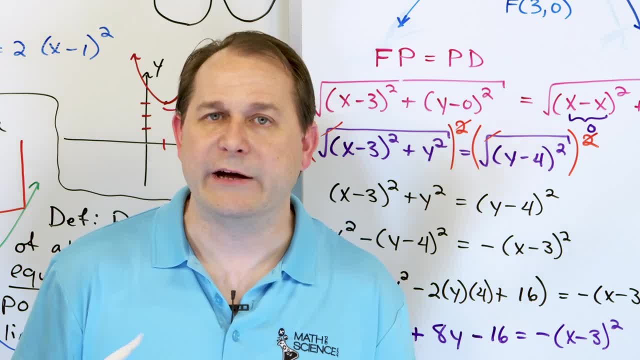 But we've used the distance formula to basically make an equation to find out that all parabolas have this form. 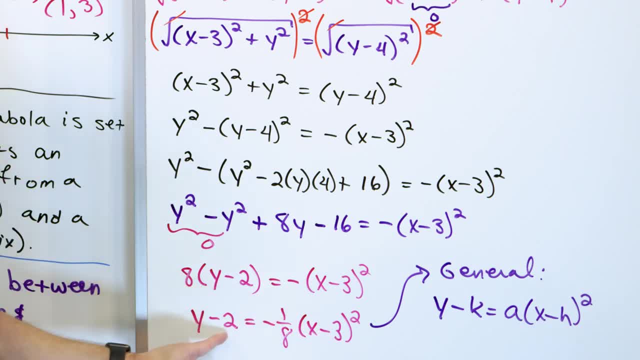 The vertex will be shifted according to these x and y numbers here. 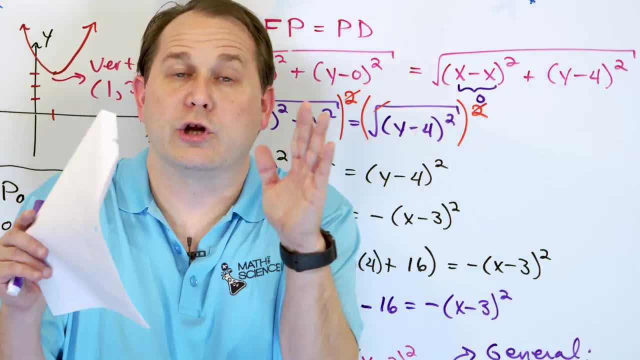 And then the a in the front is going to represent how open or closed it is and also if it opens up or down. 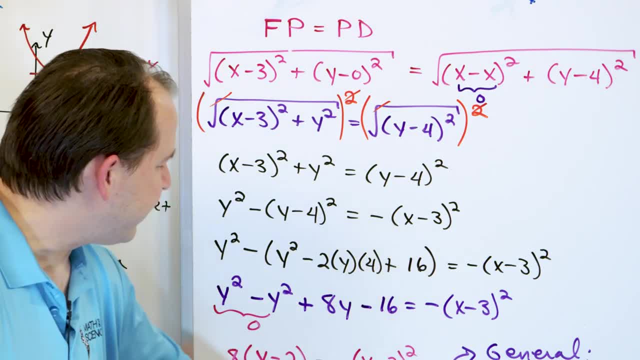 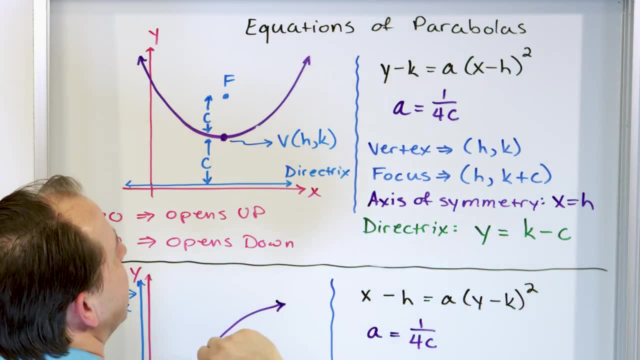 So let's just take a second to take a look at what we have here and compare it to what we have over here. We said the equation of a parabola that opens up like this looks like this. 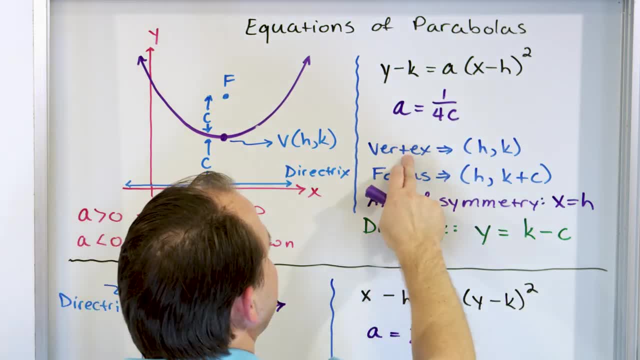 That's exactly what we've written down based on that example. The vertex is at . That's the shift in x, the shift in y. That's why the vertex is . 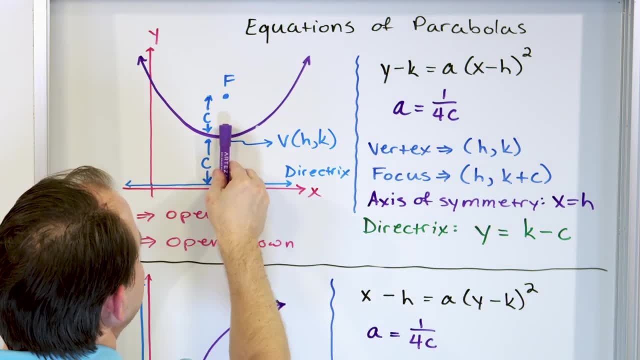 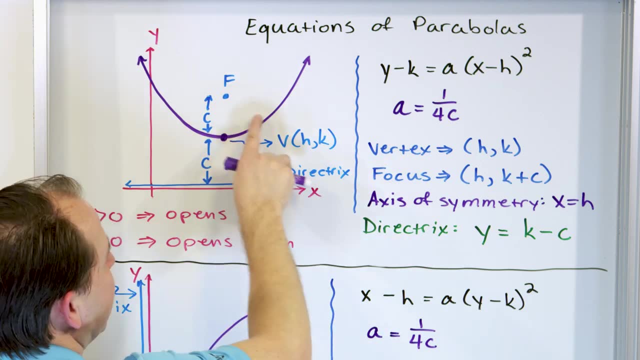 The focus has to be the same distance over in terms of where the vertex is. So the first coordinate has to be h because the vertex is here. So for the focus, it has to be h. 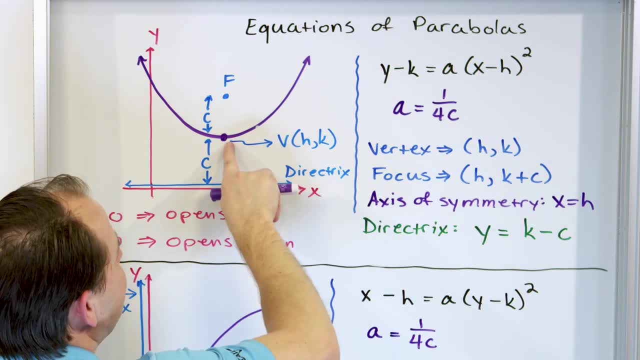 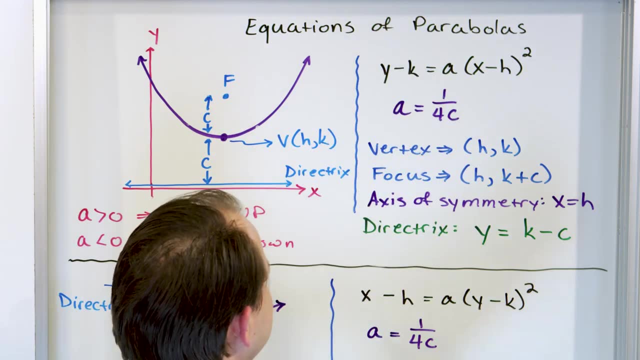 But the y coordinate of the focus has to be whatever k is plus this number c. So it's not so helpful to see it written like this, but that's why it's written like this. 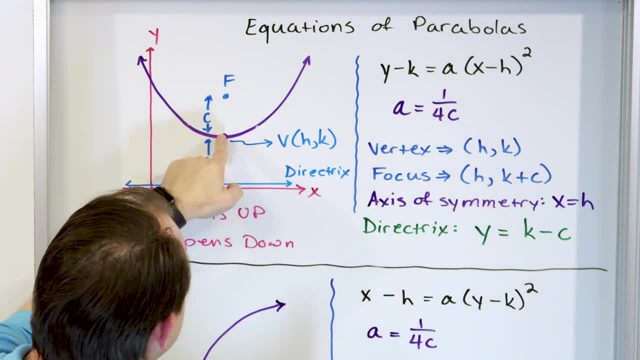 The vertex is , the focus is , because it's this point plus c units up in y. That's all it is. 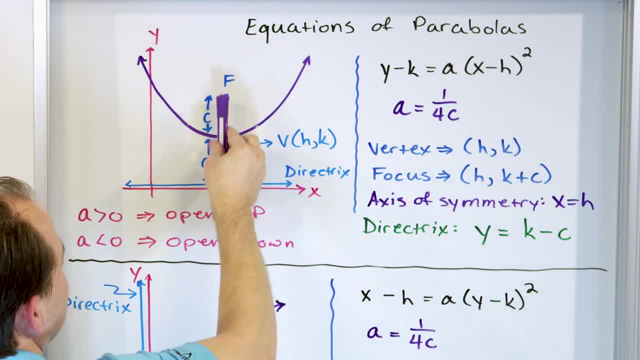 The axis of symmetry is that x is equal to h. It's a vertical line. It goes through the focus and through the vertex. That's why the axis of symmetry is the vertical line x is equal to h, this coordinate right here. 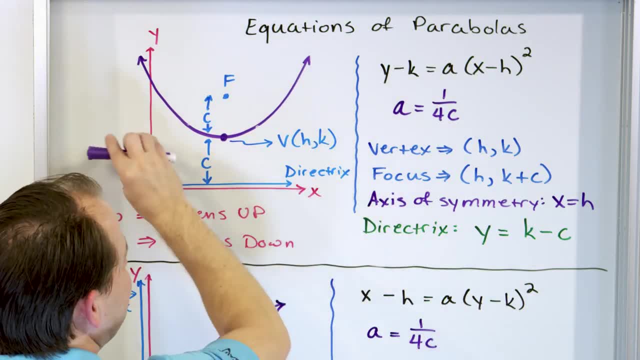 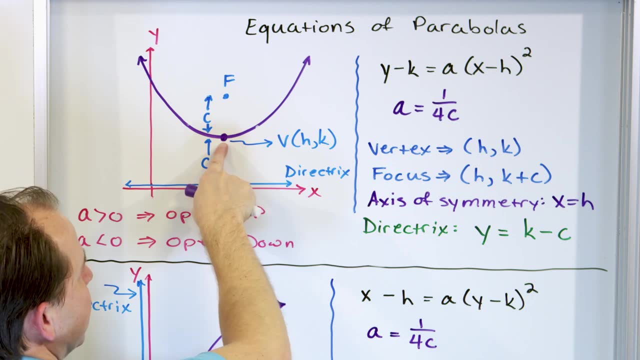 And then the directrix is the line over here. But it's a horizontal line, so it has y equals something. What is it going to be equal to? Well, it's going to be equal to wherever the vertex is. 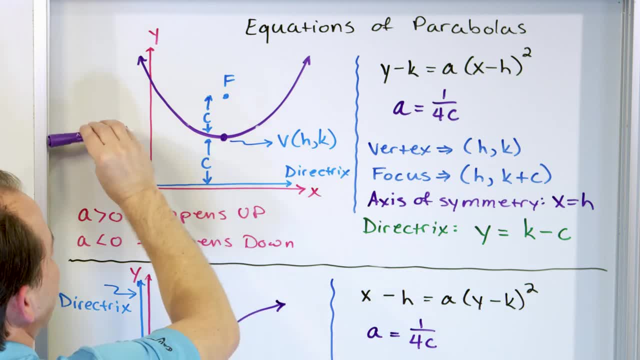 Because the horizontal line y is equal to k would go right through the vertex, but it's not that line. It's k minus c. It's shifted down. 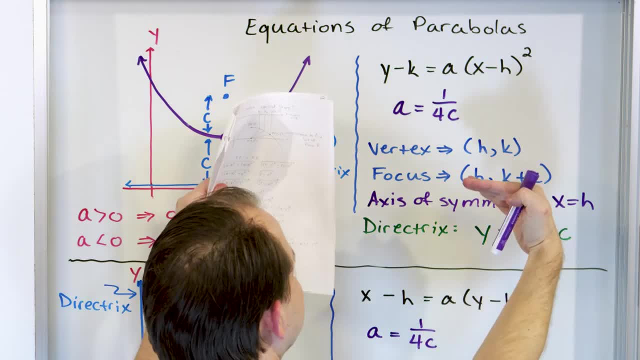 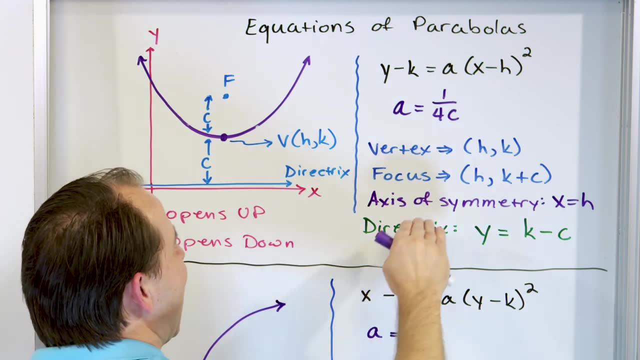 So the directrix is wherever the vertex is, a horizontal line of wherever the vertex is shifted down. The focus is the point wherever the vertex is shifted up. The axis of symmetry goes vertical through both of these points there. And then if a is greater than 0, it opens up. 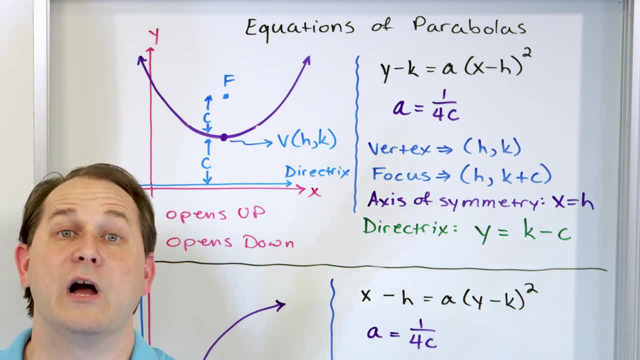 And if a is less than 0, it opens down. It's a monster, right? 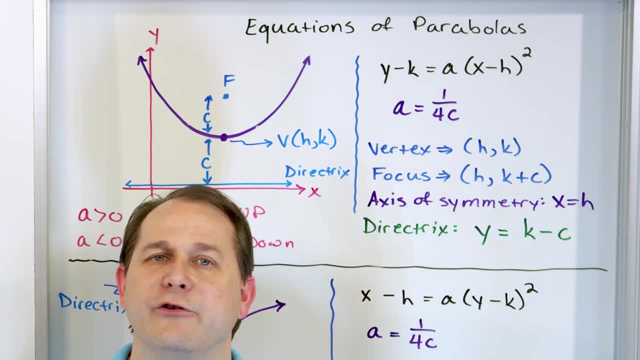 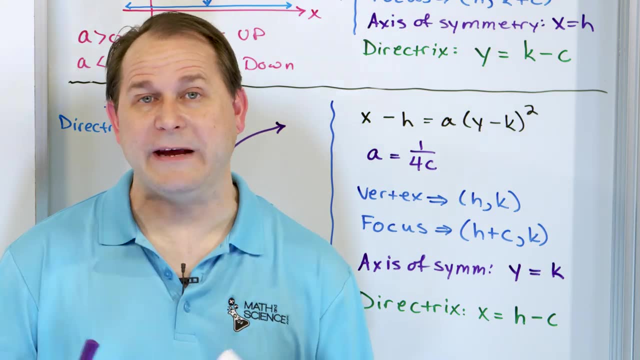 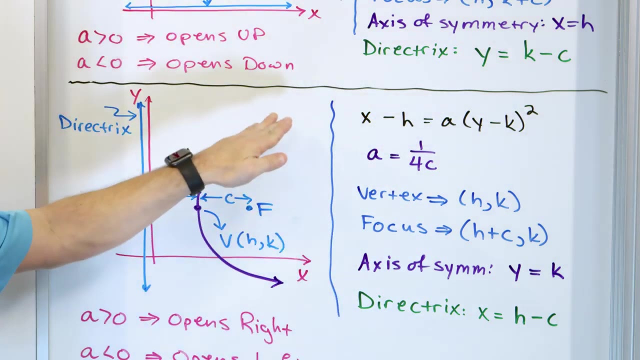 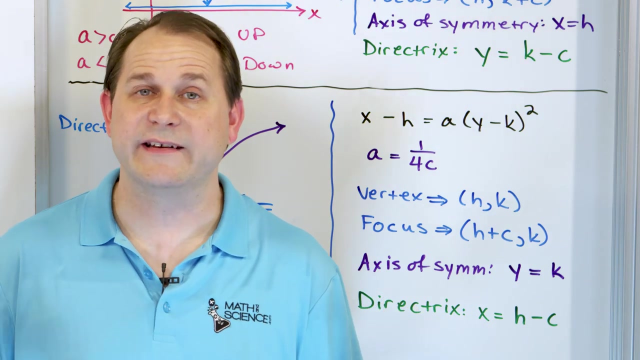 To derive it all and then cram it all into one lesson, but now you know where everything comes from with a practical example. Now, I would love to be able to stop here. And just say, go do all of your problems. However, every class is going to give you problems that has a sideways parabola as well. And that's, honestly, it's just not fun to have to do it all in one lesson, but I need to get that out to you as well. 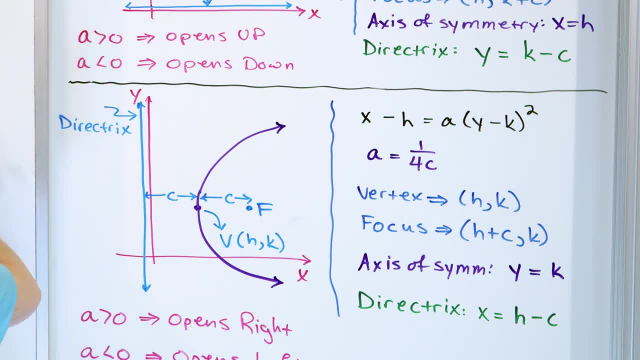 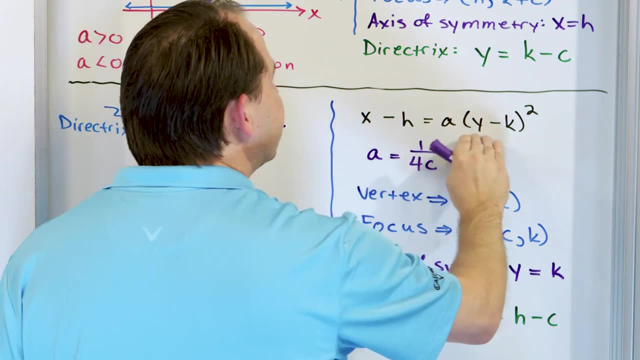 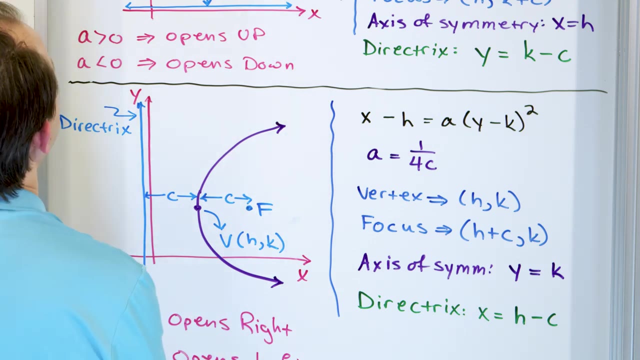 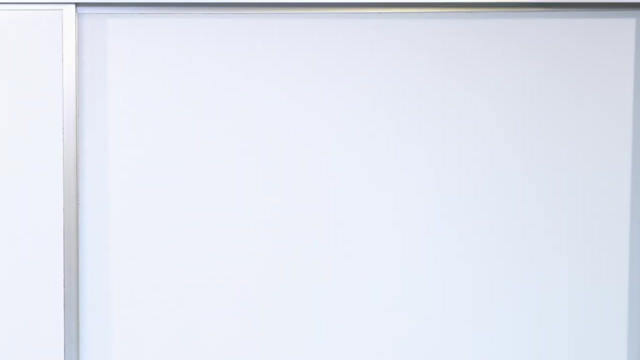 So what we're going to do is we're going to do the same thing that we did before. We're going to derive this equation, which is going to be very easy to do now that you know how we did the first one. And we're going to find out that the equation of a sideways parabola is this one, and we're going to talk about how the vertex and the focus and all that stuff makes sense there as well. So in order to do that, I have to draw, like I did here, I had to draw a picture of a parabola and I had to do the calculations. Now we have to draw another picture of a parabola and do the calculations on that one as well. 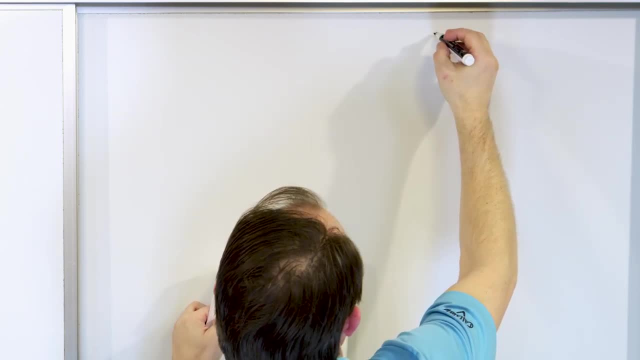 So what we're going to have, let's see if I can draw this thing right. So what we're going to have is an xy coordinate. It's not going to be perfect. I apologize for that. 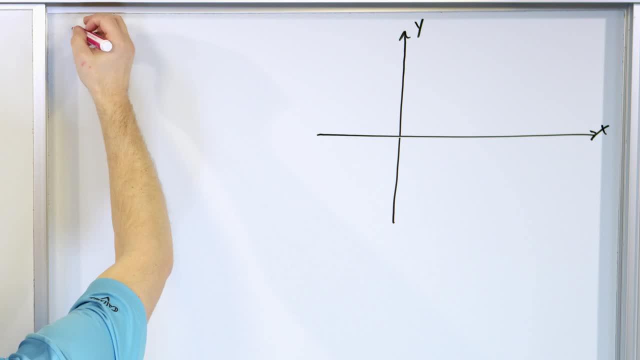 I'm going to advance. So what I want to do is I want to find, and this could be some kind of a test question, 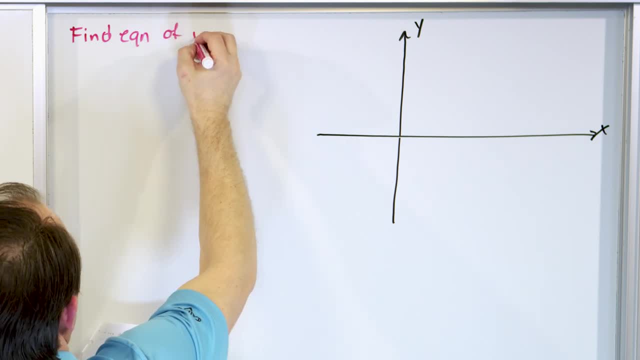 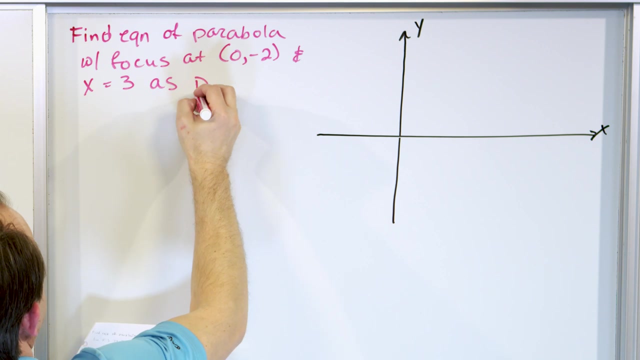 find the equation of parabola with focus at and x is equal to 3 as the directrix. All right. 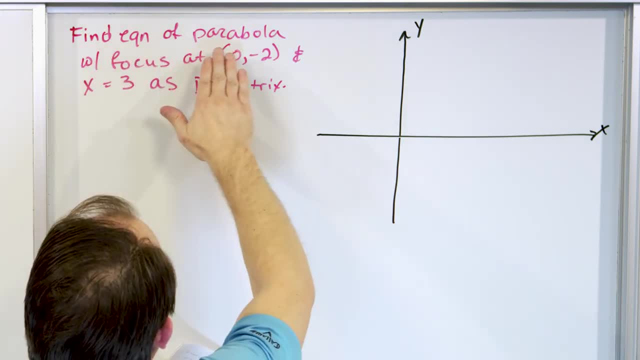 So what we have figured out, or what the problem tells us is, find the equation of the parabola with the focus at . 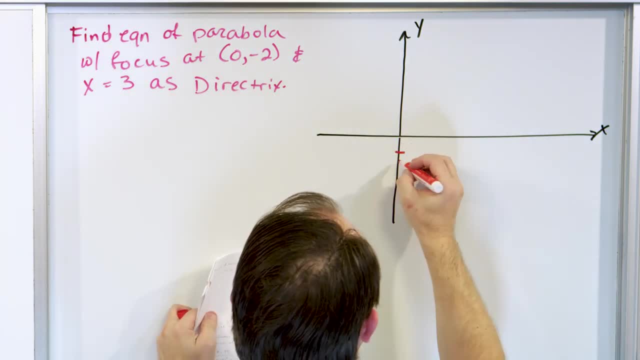 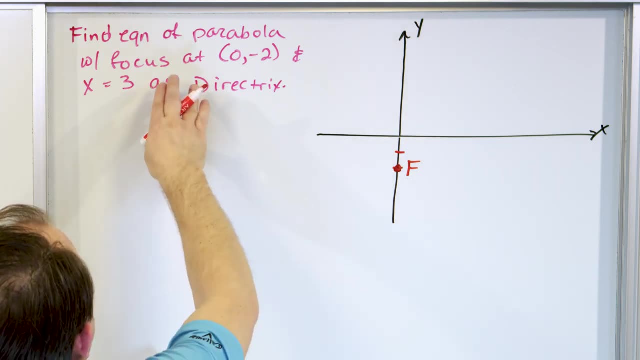 So we can write that down right away. is going to be down here. That's going to be the focus of this thing. And I can put an f there to tell you that that's the focus. At , x is equal to 3 is the directrix. So here's 1, here's 2, here's 3. 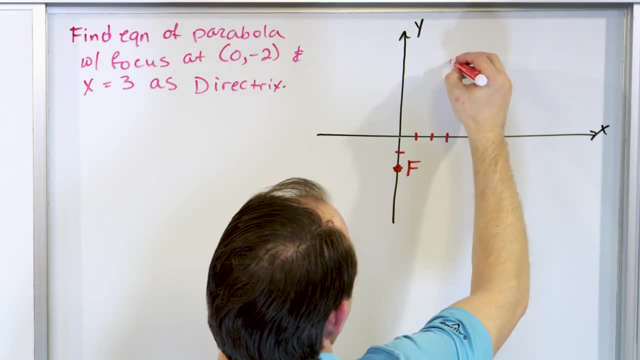 So I'll put a, because it's x is equal to 3, it means it's a vertical line. 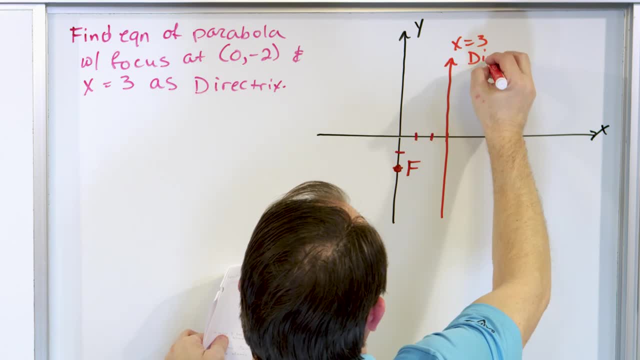 So this is x is equal to 3. This is the directrix. OK. 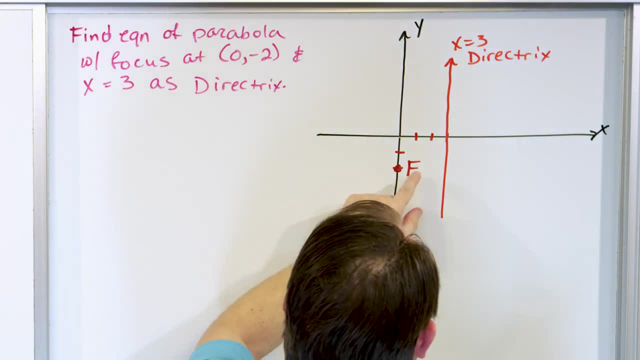 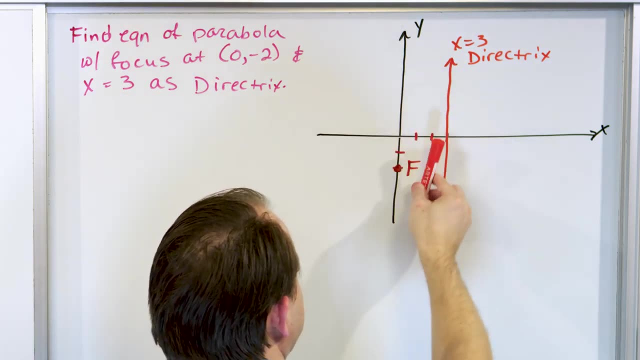 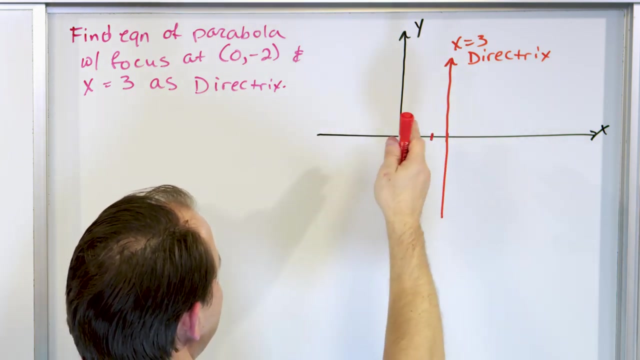 So because this thing has a focus here and a directrix here, you know the parabola has to open to the left, because the focus has to be inside the bowl, so to speak. And it also has to be where the backstop, so to speak, the directrix is aligned on the other side of the rear end of the parabola. So the parabola has to go something like this. 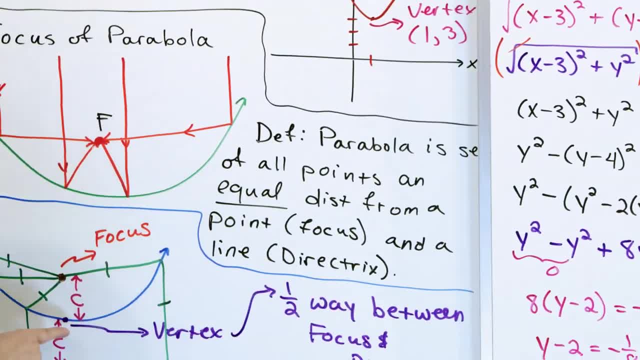 But also we've learned many times over that the vertex is always halfway between the focus and the directrix. 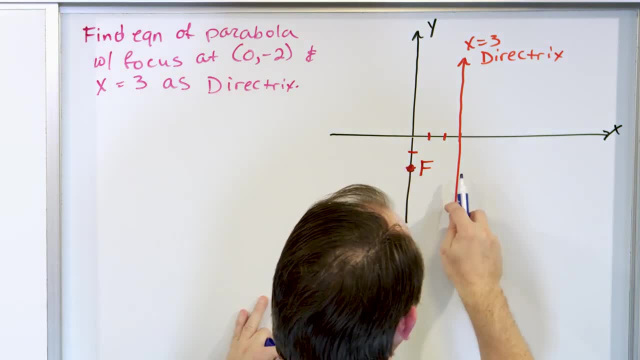 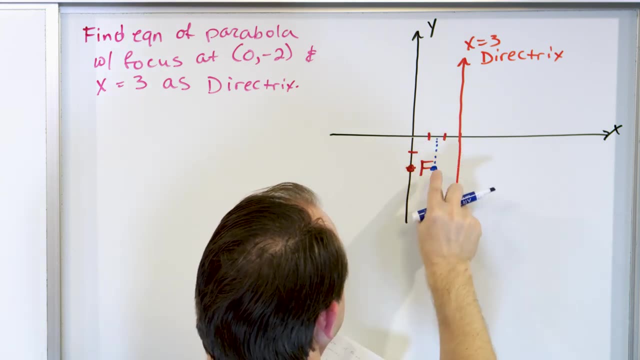 So in this problem, we actually know what the focus is, and we know what the directrix is. And so we know there's three points here. So this down here, this point right there, in between these tick marks down there, has to be the vertex. 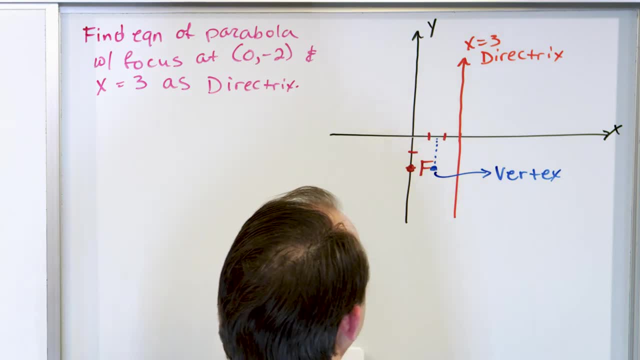 So I'm going to put here, this is the vertex. And what is the coordinates of that vertex? It has to be 1, 2, 3 units, but I have to cut it in half. 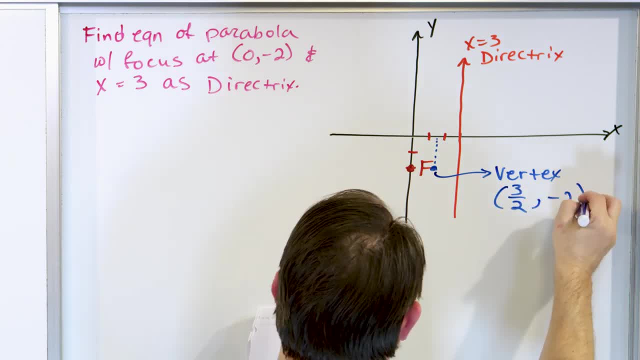 So the vertex is at . The vertex is at because it has to be in between the focus and the directrix. 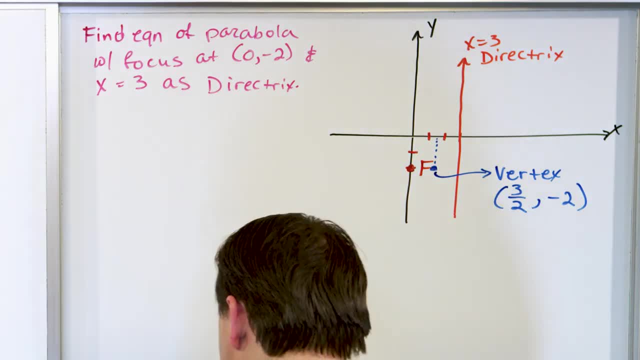 Now what does this parabola look like? I always mess these things up, 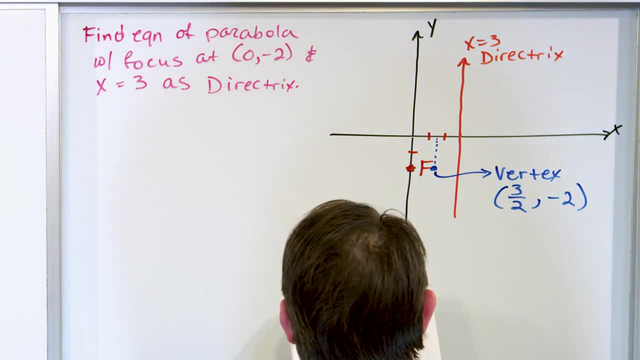 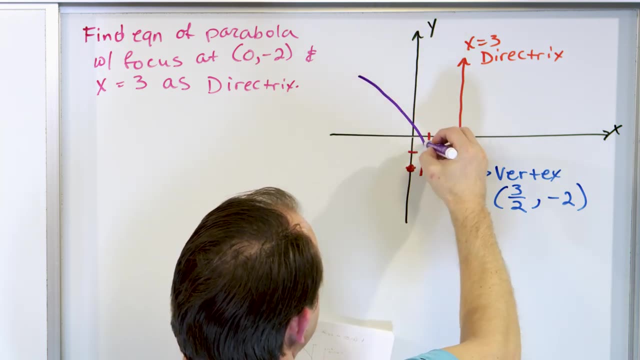 so I'm going to just ask you to accept my apologies already. But it has to go something like this, and it has to go through the vertex. So it's going to do something kind of like this. It's going to go down, it's going to flatten out, it's going to come out like this. Is it perfect? No. 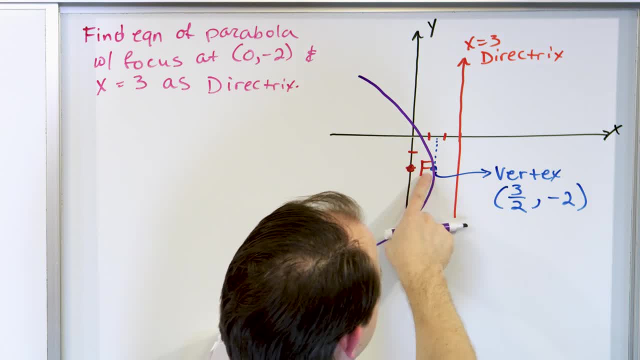 I think I drew it more where the vertex is more like here. You have to use your imagination and pretend that I'm a good artist, so sorry about that. So it's going to be something kind of like this. That's too kinked. 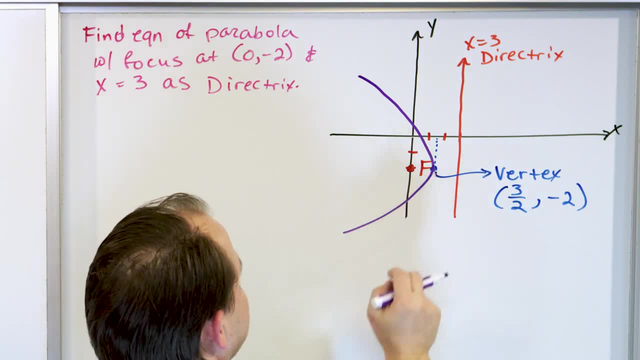 But anyway, you see the vertex is right there at the lowest point. The thing opens up like that. 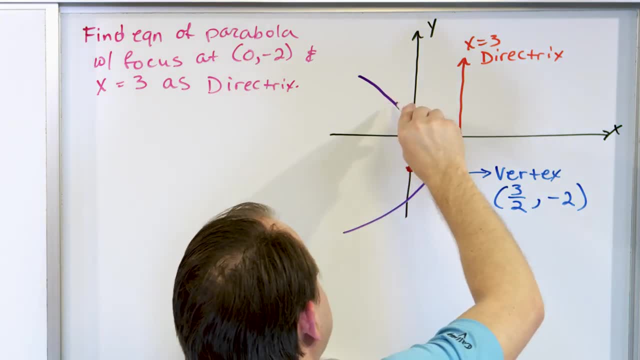 Now the definition says that every point on this purple curve is an equal distance to the focus as it is to the directrix. 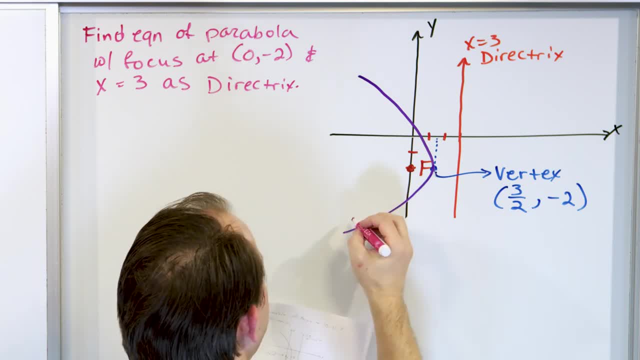 So for instance, down here is a point on the curve. We can call this point , right? 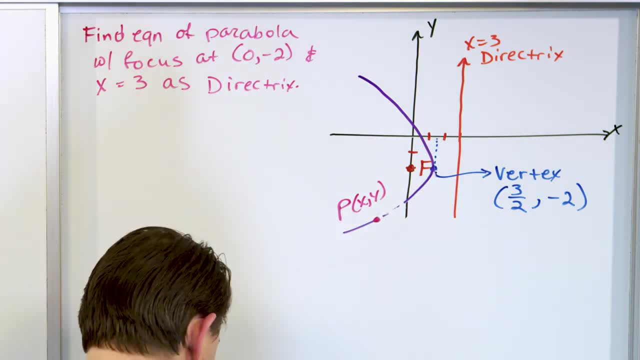 And what this is basically saying is that, look, I messed up my little curve here. Sorry about that. 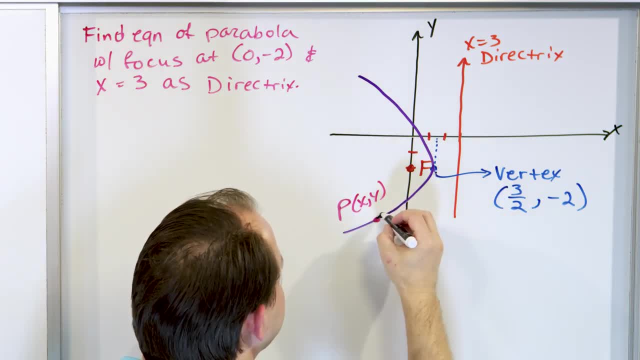 What this is basically saying is that the distance from this point on the parabola to the focus is the same as this distance from the point to the directrix. So I'm going to put a little tick mark line. 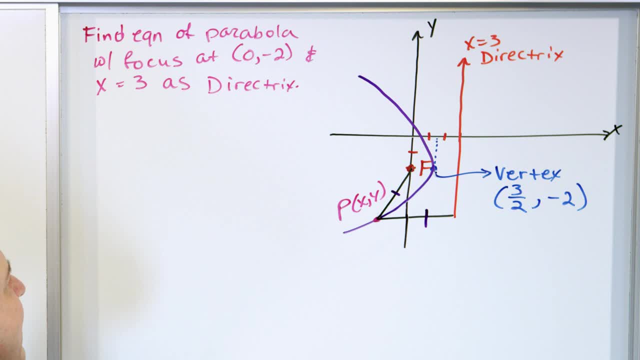 This means that's the same distance as this guy. And that holds for every other point on here. I can draw additional points if you want. 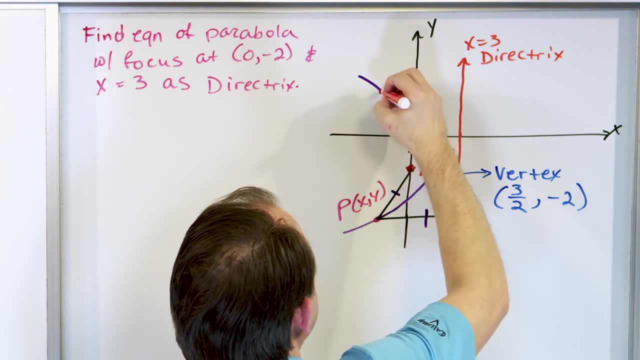 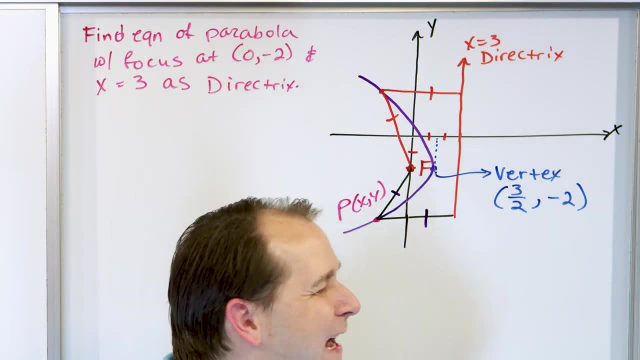 I can pick a point up here and say, well, this point right here is an equal distance to the focus as this point is to the directrix. Those are equal distances. And this purple curve traces out all the points 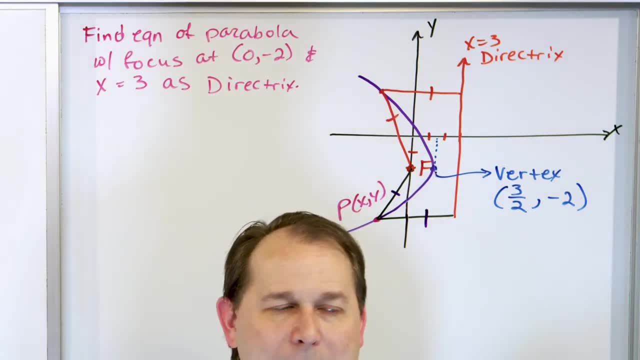 and all possible values of this thing we call the parabola. 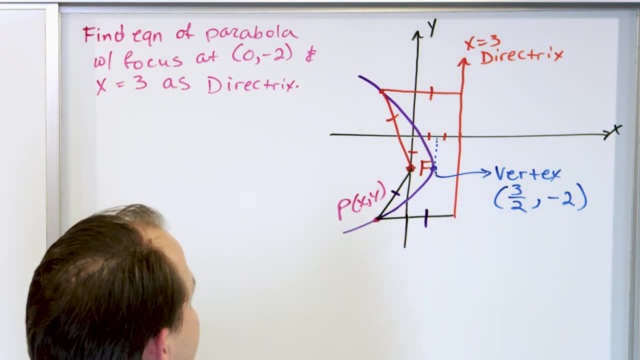 Then every point on here is an equal distance to the focus as it is to the directrix. All right. 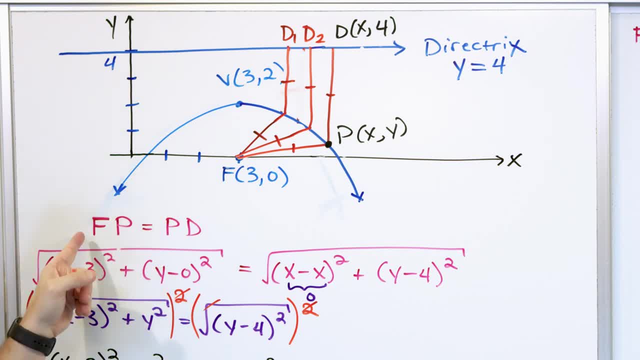 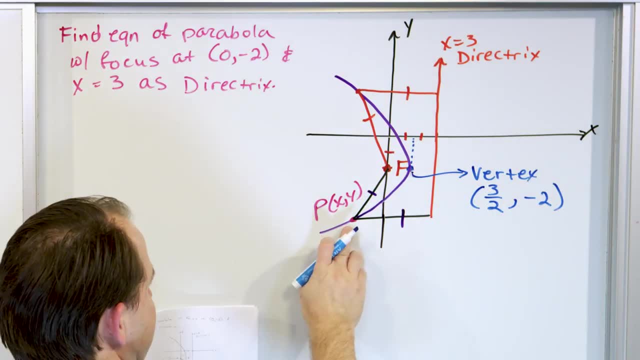 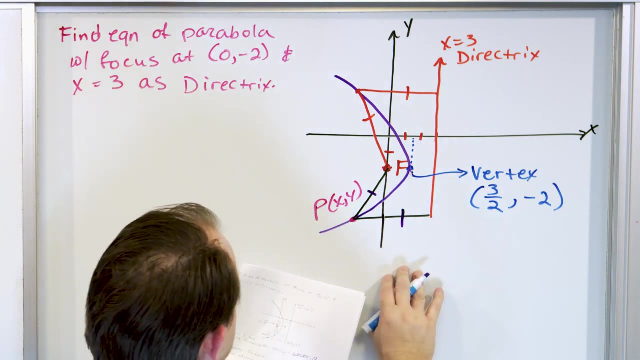 And so we're going to do like we did in the last problem. We basically said, well, the distances have to be equal. So we're going to set the exact same thing up. And we're going to say that if this is p, p of x, p, x, y, and this is f, and this is the point on the directrix in this case, down here, it's going to be, this point's going to be d. It's going to be at 3, y. Why 3, y? Because the directrix is at 1, 2, 3. That's the x-coordinate of this point right here. 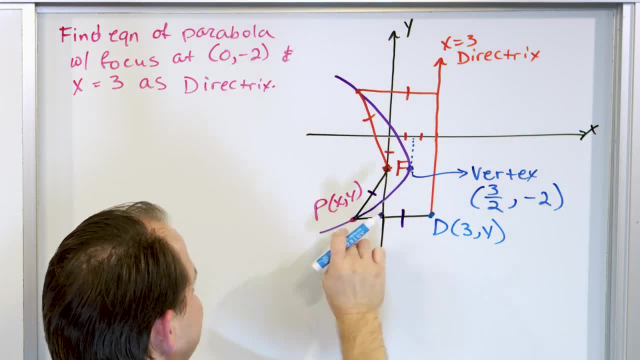 The y-value I don't know because it depends on basically wherever I'm tracing out, whatever point I pick is going to dictate the y-value. 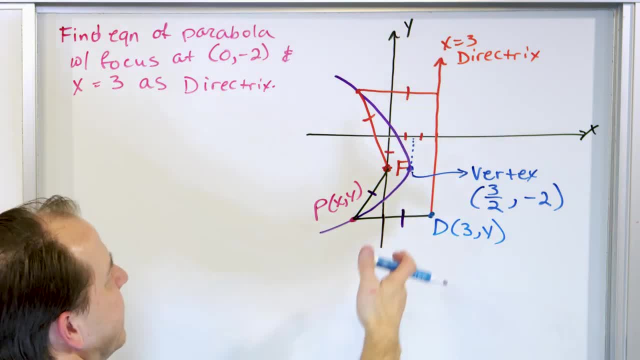 But the x-value is always going to be the same because the directrix is always a vertical line at x is equal to 3. 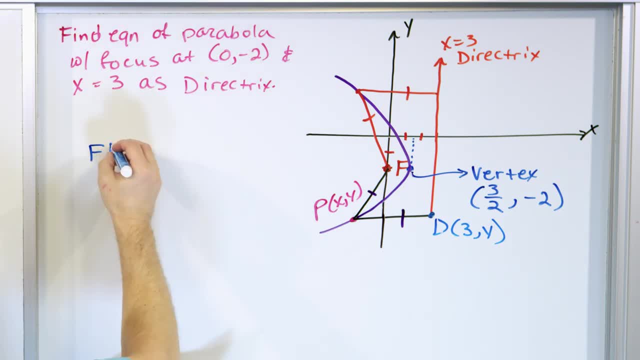 So what we're saying is that the focus to the point p is the same distance as the point p to the directrix, same equation that we used before. 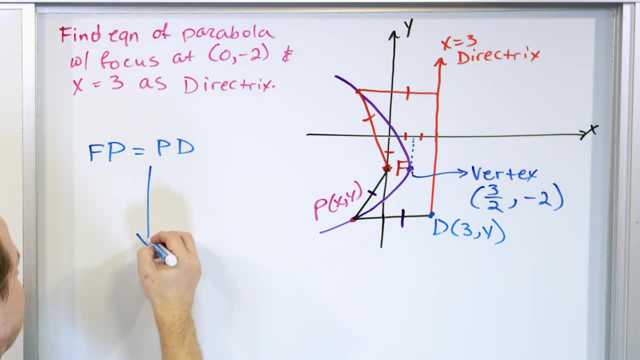 So we have to use the distance formula. So I'm going to have to scooch down a little bit 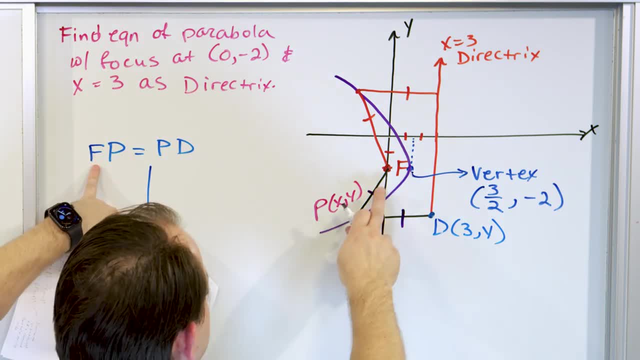 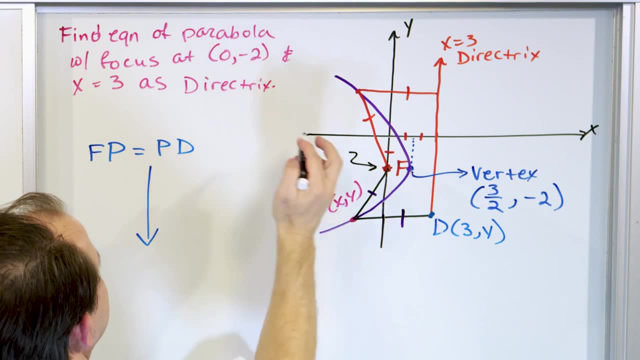 to make sure I have room. What is the distance between the point f and the point p? Well, the point f was given in the problem statement. The focus was at 0, negative 2. 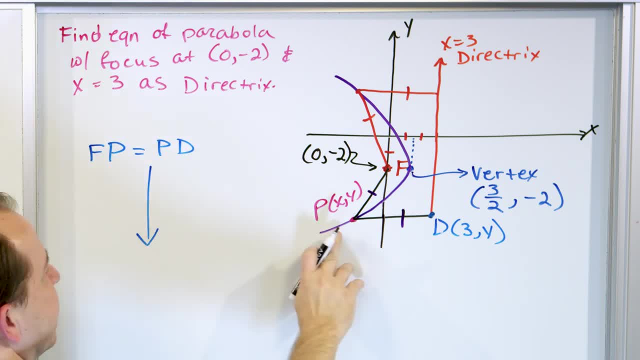 So what we're going to find is the distance between fp. So let's go and take the difference in the x values here. So it's going to be x minus 2. x minus 0 quantity squared. x minus 0 quantity squared. Plus the difference in the y values. y minus a negative 2 quantity squared. We have to take the square root to find the distance between those points. But we're saying that that distance is the same as this distance. 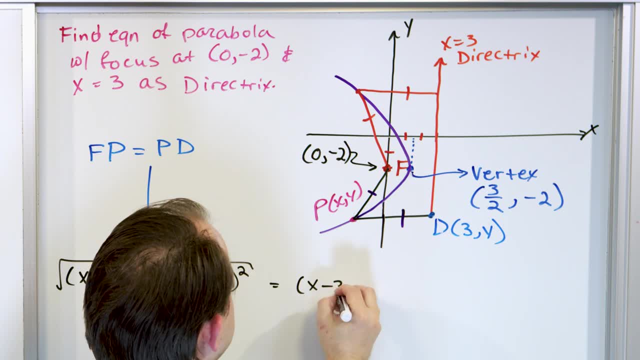 So we're going to take the difference in the x values here. x minus 3 quantity squared. Plus the difference in the y values, which is just y minus y quantity squared. 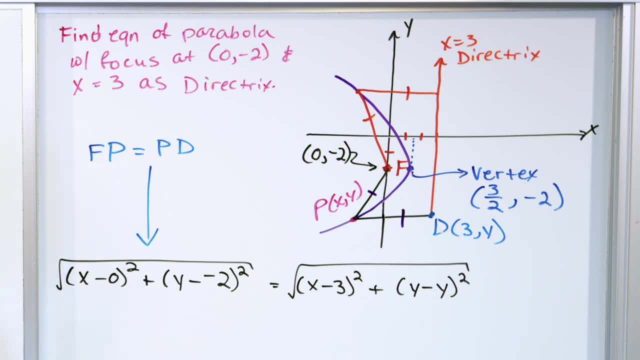 And we're going to have a radical on top of both of those things. Now let's clean it up a little bit. What we're going to have, x minus 0 is just going to be x squared. And then this is going to be y plus 2 squared. We're still going to have a radical. 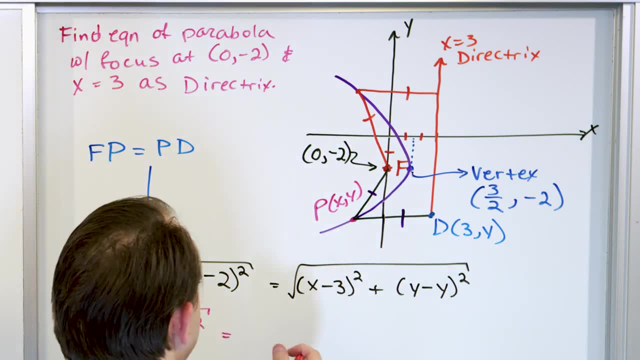 On the right-hand side, let me switch colors. It's getting a little bit hard to see. 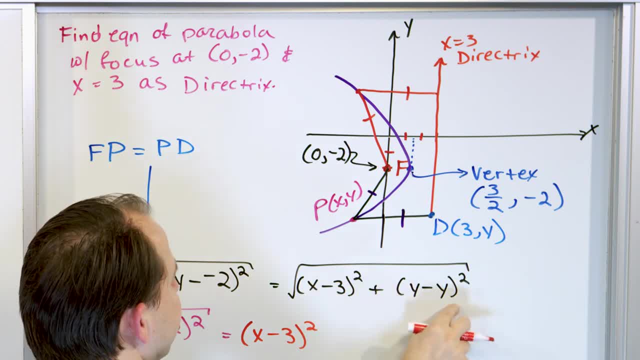 x minus 3 quantity squared. This becomes 0. There's nothing else there. 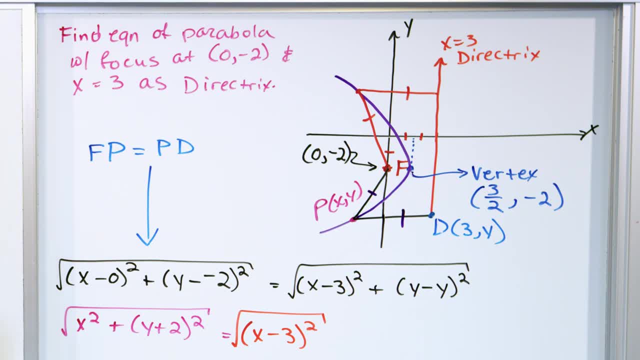 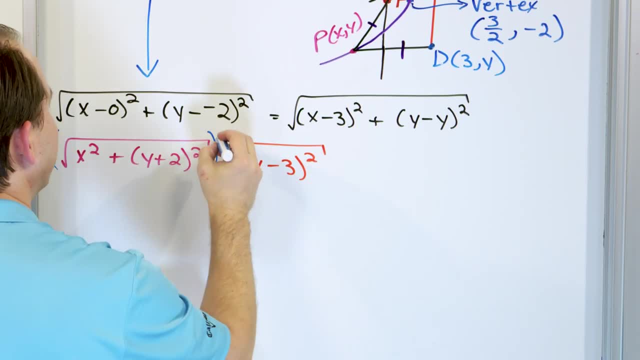 So we still have the square root outside of this guy. Now we have a radical on the left and a radical on the right. So how do we get rid of the radical? Same as before. 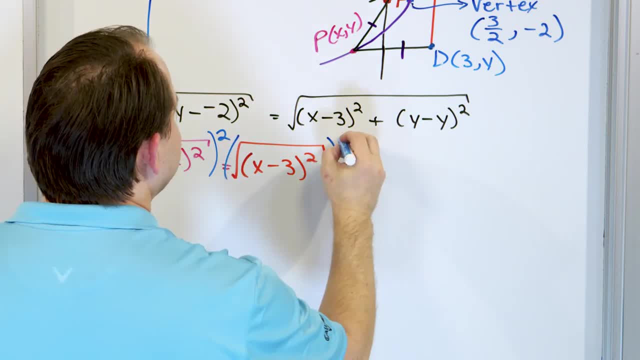 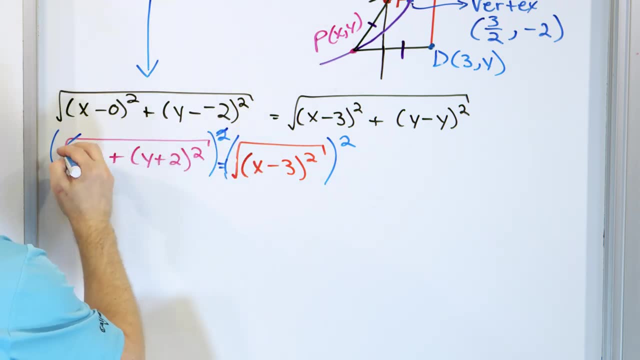 We just square the entire left-hand side of the equation. And then we're going to have to square the entire right-hand side of the equation. So there's still an equal sign between here, like this. And so this square is going to cancel with the radical. And this square is going to cancel with the radical. So really all you have is what's left underneath it. x squared plus y plus 2 squared is equal to x minus 3 squared. All right? So now what we want to do is we want to rearrange terms. 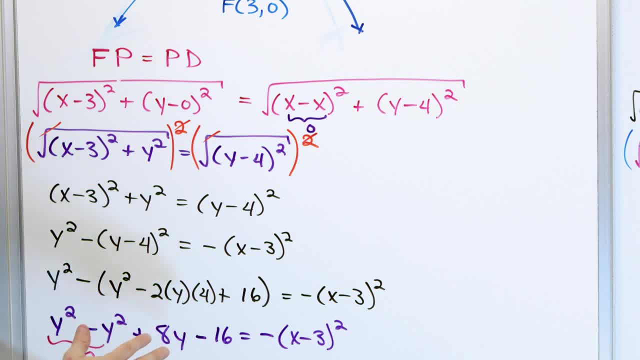 Now in the previous time we did it, it was a vertically oriented parabola. We wanted to put all of the y values on the left and all the x values on the right. 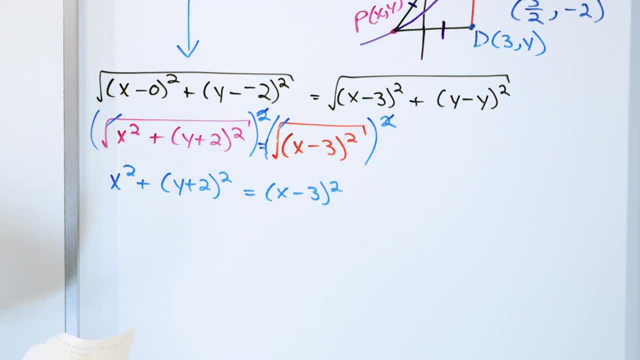 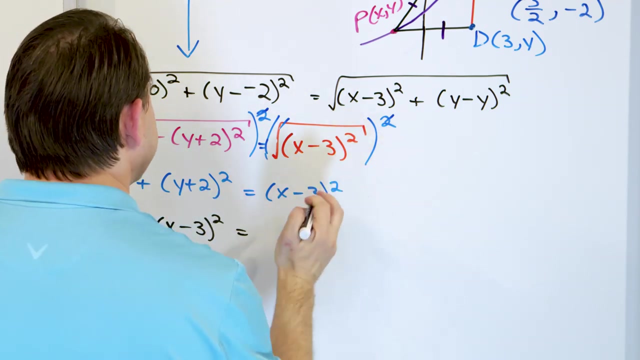 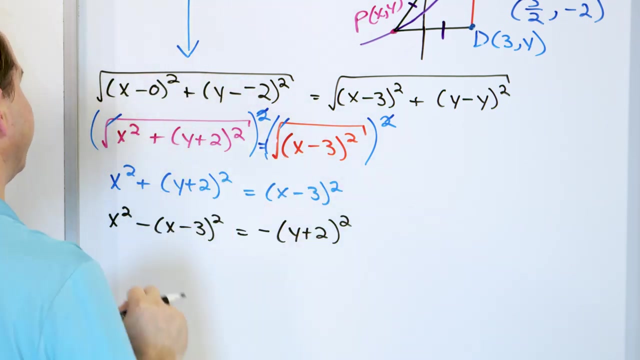 And now we're going to do it exactly in the opposite way. We want to take and move this term over here and this term over here. You'll see why in just a second. So what we're going to have is the x squared minus what's on the right, x minus 3 quantity squared. We'll take this and we'll move it to the right. So it's going to be negative y plus 2 quantity squared, like this. So all we did was we moved this term to the left, this term to the right. 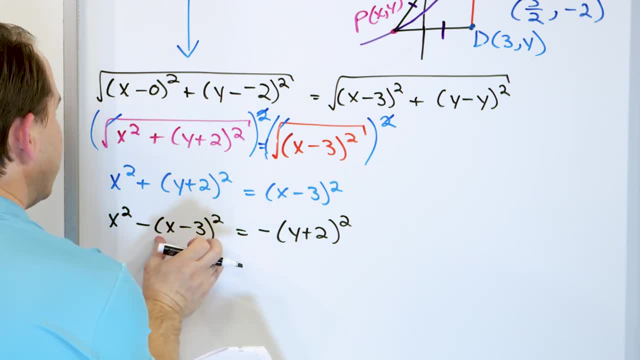 And so now we want to simplify this. So we want to expand this term out as we did before. We'll have a x squared minus 2 times x times 3 plus 3 times 3 is 9. 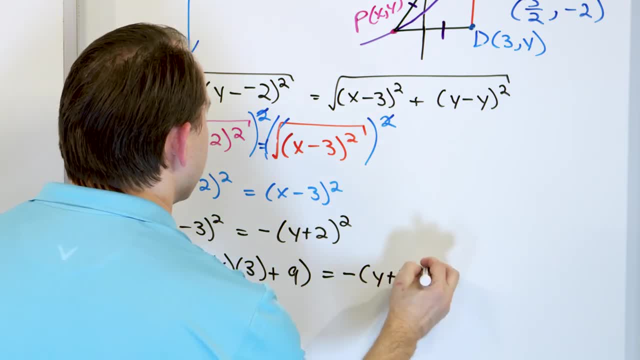 And then we're going to have negative y plus 2 quantity squared. All we did was square this binomial. 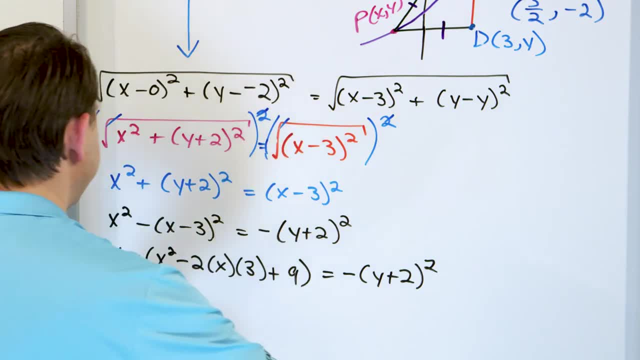 We've done that so many times. You should be able to do that in your sleep by now. Now we have to distribute the negative n. Sorry, this is an x squared. I forgot to write that down. 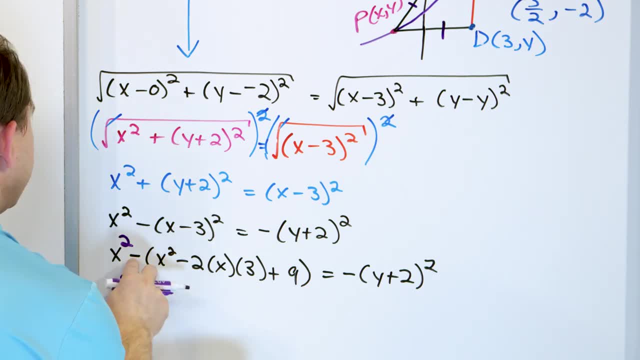 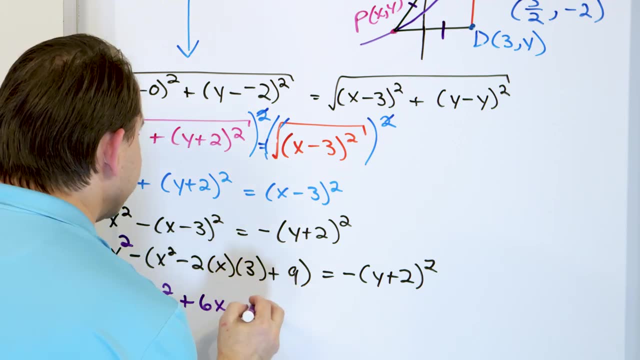 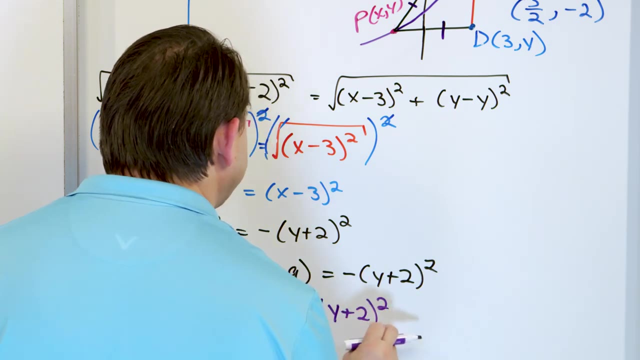 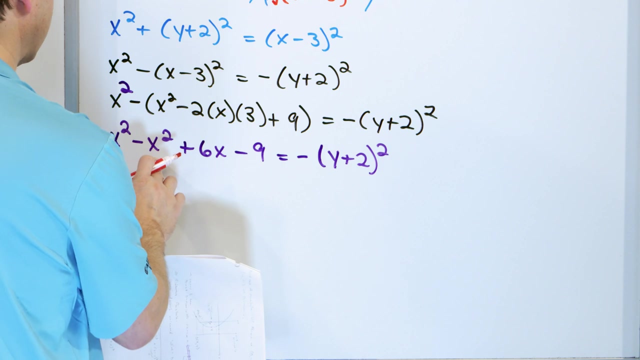 So we'll have an x squared minus x squared, taking that negative n. This will be a positive term. 2 times 3 is 6x. And then the negative times the 9 is negative 9. And on the right we'll have negative y plus 2 quantity squared. We don't want to expand this right-hand side because it's already in the form that we want it to be in. We want it to be in the form that we want it to be in for a parabola. So this gives me 0, like this. And then I look at this 6x minus 9. The 6 in front, I want to factor out a 6. And you'll see why in just a second. Let's factor out a 6. 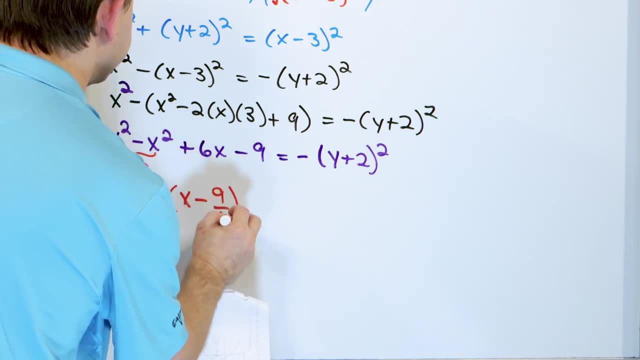 And when I do that, it's going to be x minus 9 over 6 is equal to negative y plus 2 quantity squared. If you don't see this, just make sure and go backwards. 6 times x is 6x. 6 times this fraction, the 6's will cancel. So it'll just give you a negative 9. You're just factoring out the 6. And when you don't have, it doesn't go in evenly. 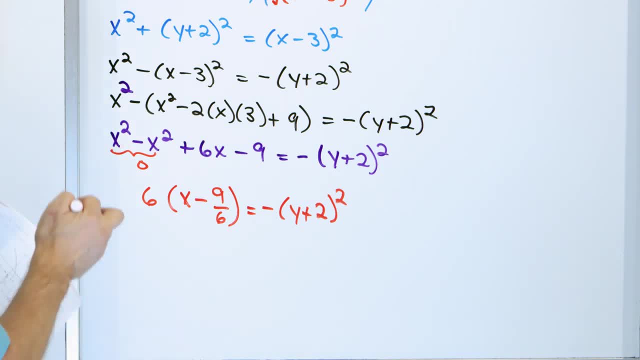 Sometimes you have to write that second thing as a fraction like this. Alright? 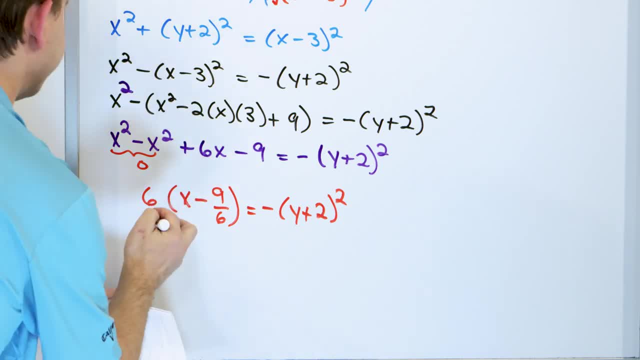 So now we're getting very close. This coefficient in the front, we want to divide by it. 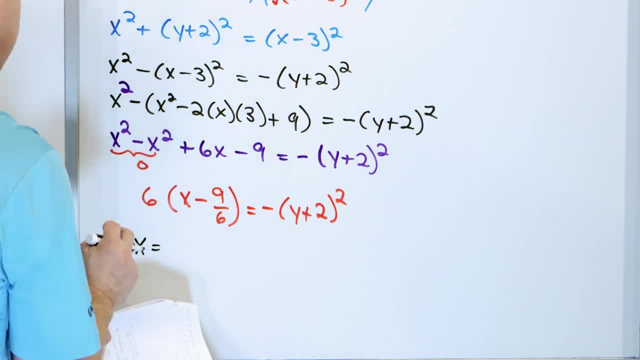 And this 9 over 6 is also going to be able to be written easily as well as... This 9 over 6 is the same as 3 halves. 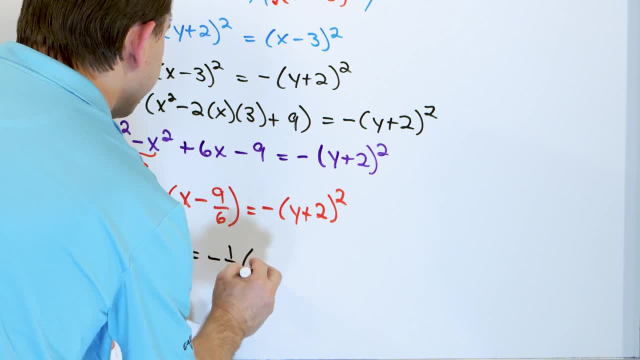 We're going to divide by 6, so it'll be negative 1 sixth. y plus 2 quantity. squared. 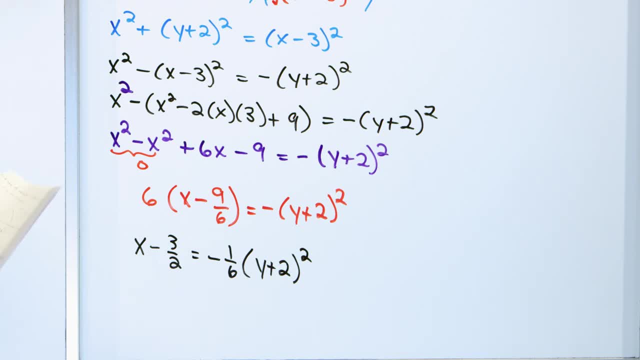 So we have x minus 3 halves is equal to negative 1 sixth y plus 2 quantity squared. So, is this correct? 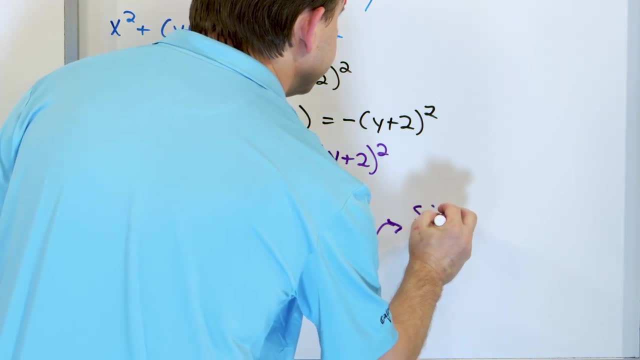 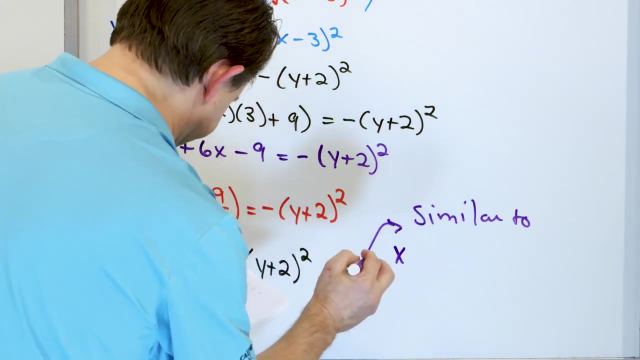 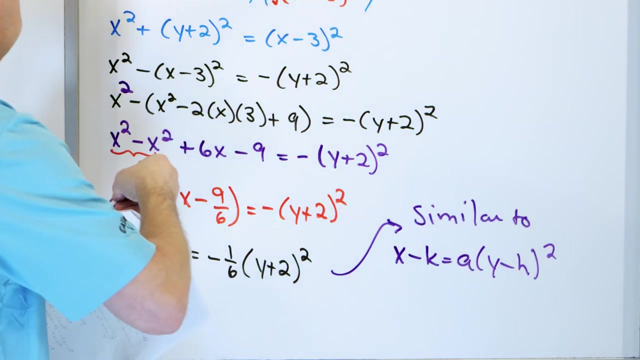 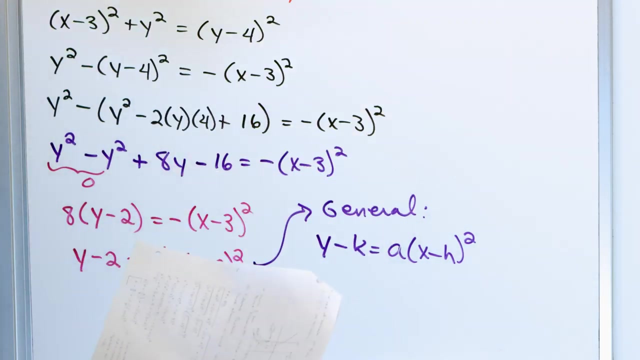 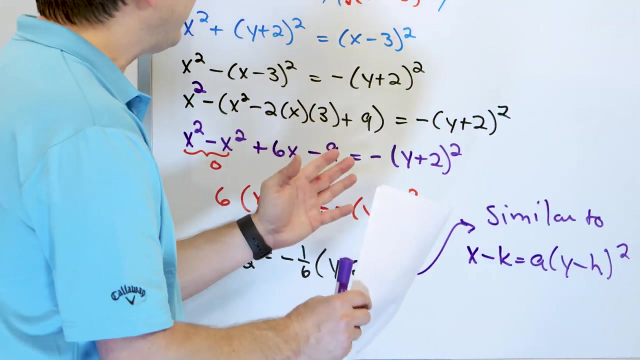 Well, this is similar to the general form of the equation of a sideways parabola, which is x minus k is equal to a y minus h quantity squared. So you can see what's going on here, right? The parabola that is oriented vertically up and down, so to speak, has the y value on the left, but the x term, the x term is on the right, and that is what is squared. For the sideways parabola, everything's flipped around. The y term is what's on the right, that's what's squared, and the x term is on the left. 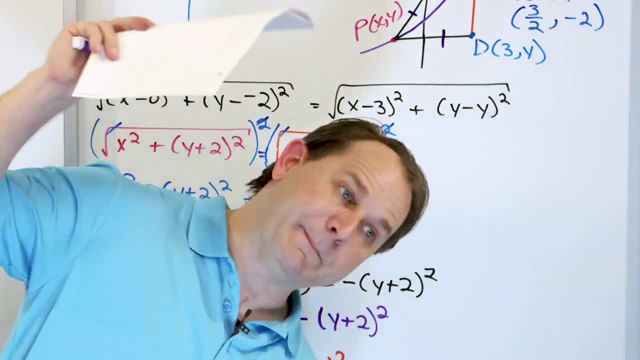 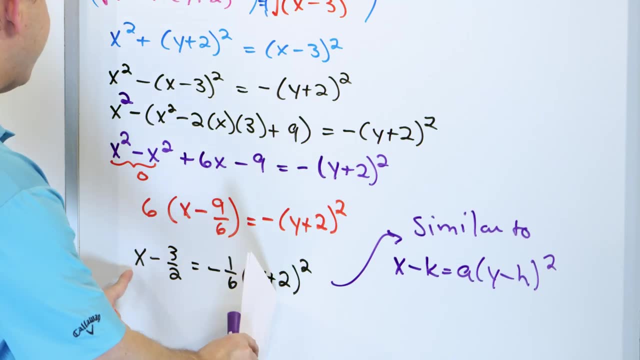 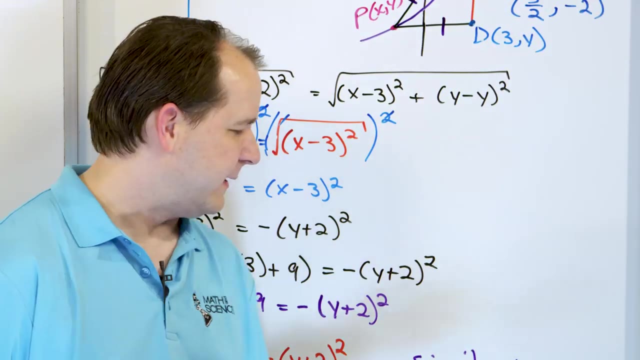 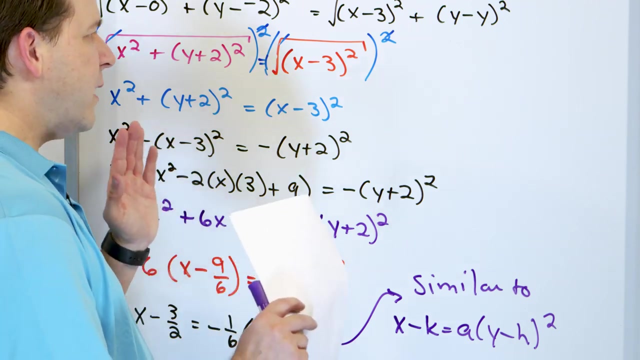 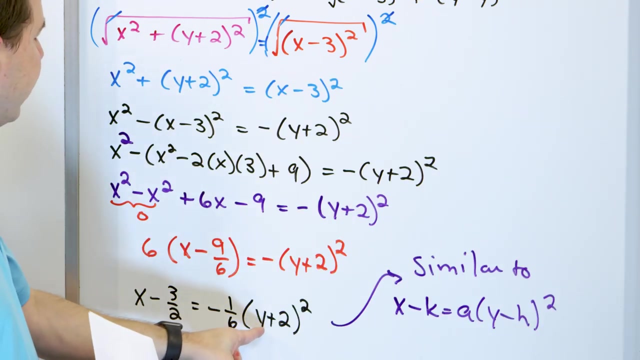 So it's totally written backwards to a typical equation, and that's because you flip the thing sideways. So one way to think of a sideways parabola is just the same thing as a vertical parabola with the x and y variables flipped. You can flip them around. So if this were y and this were x, flip it around, and that's going to make a sideways version of that parabola. But it still has a coefficient in front. In this case, it's negative. So because it's negative, a positive value would open to the right. A negative value opens to the left, which is what our drawing had. The vertex of the parabola is that y is equal to negative 2 and x is equal to positive 3 halves. 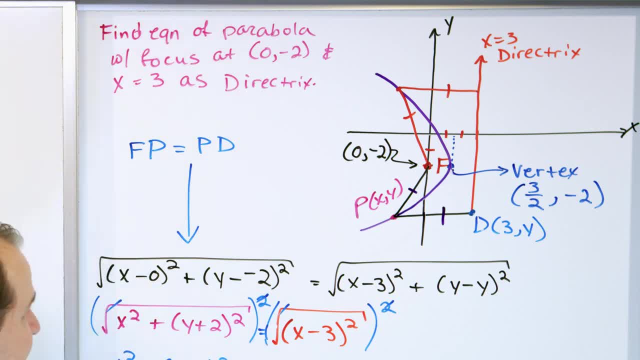 So x is equal to positive 3 halves, y is equal to negative 2. That's exactly what we have here. The y goes with this, the shift in x goes with this. 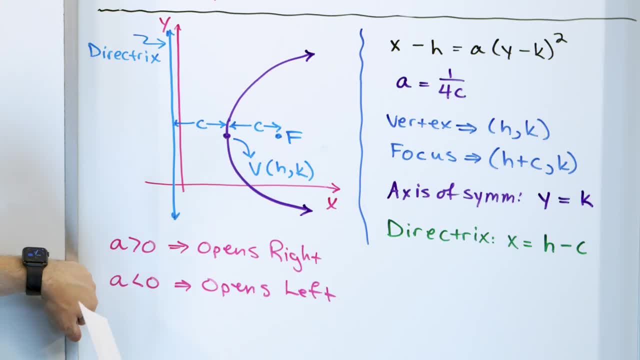 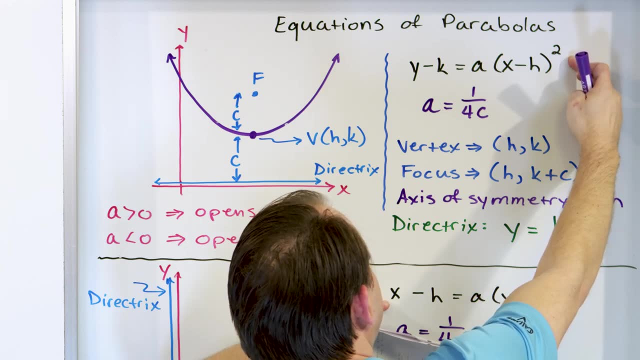 And now that we have done that, we can now look at the sideways version of the parabola. The equation of the parabola looks exactly like the equation of the other vertically oriented parabola. 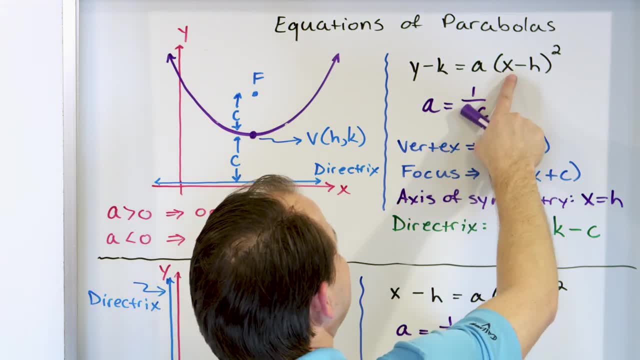 It's just that we take the y value and we replace with x, we take the x value and we replace with y. 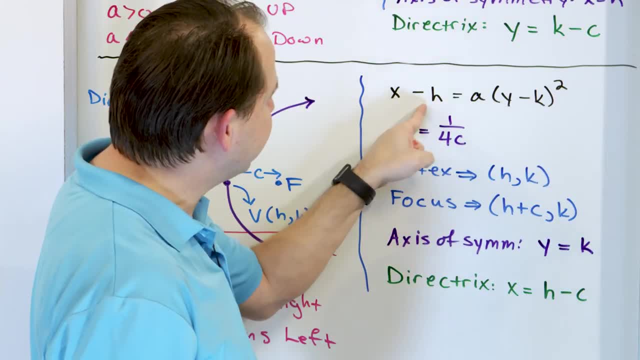 The vertex is still at . The x shift goes with the x coordinate of the vertex, the y shift goes with the y coordinate of the vertex. So this is the vertex. 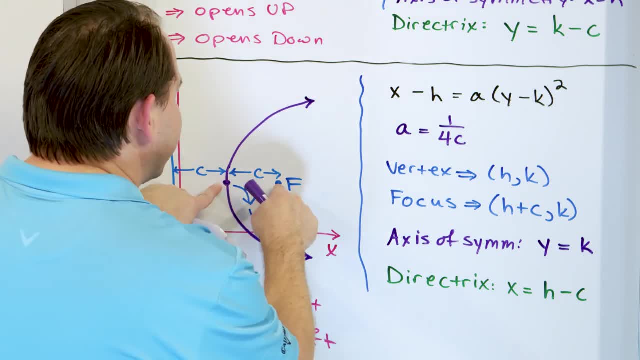 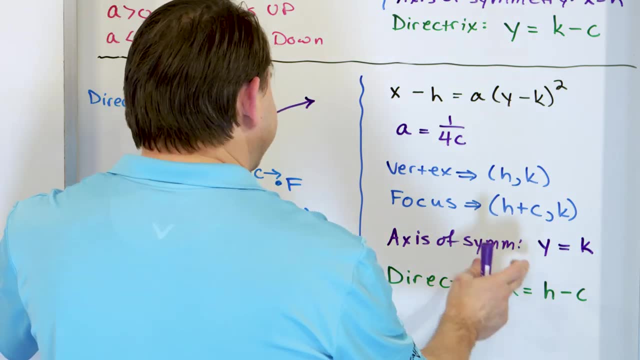 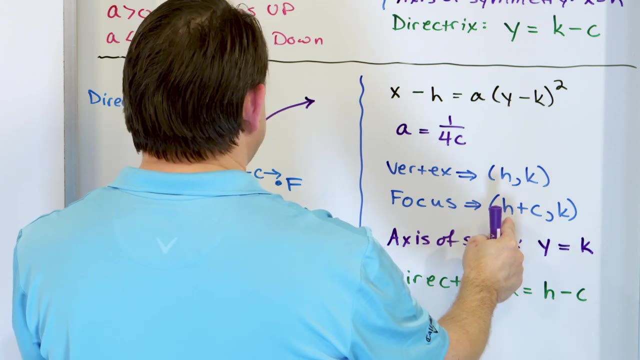 The vertex right here, the focus has to be this point but plus a little more in the x direction. So we have to add c in the x direction, k stays the same. The directrix is c units in the other direction. So it has to be a vertical line that is h instead of plus c, it's going to be minus c because it's going to be a line that's going to be over here. 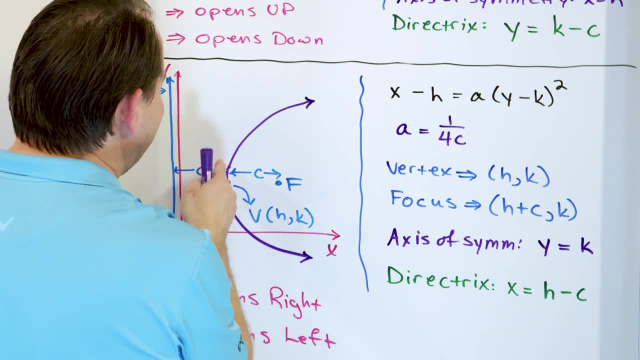 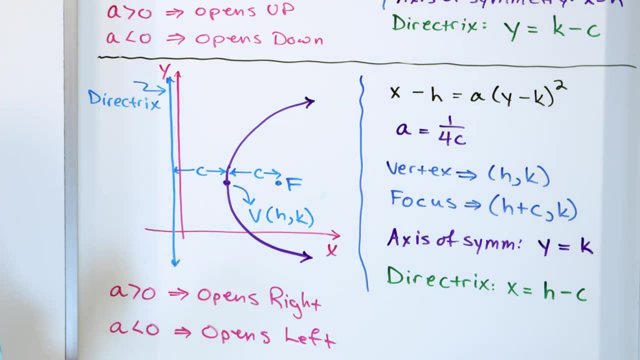 In other words, a vertical line that goes right through this point would be x is equal to h, right through here. But we don't want that line. We want it to be c units this way. So we call it h minus c. 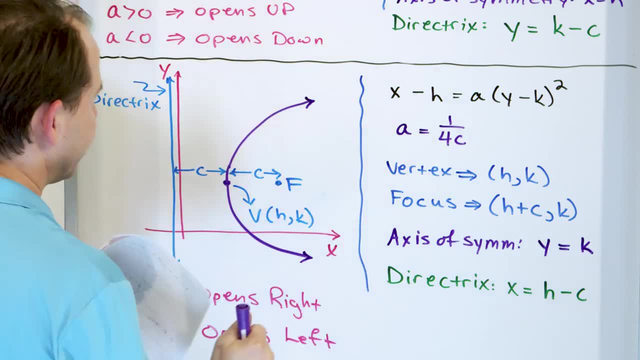 The axis of symmetry for horizontal parabolas like this is a horizontal line. 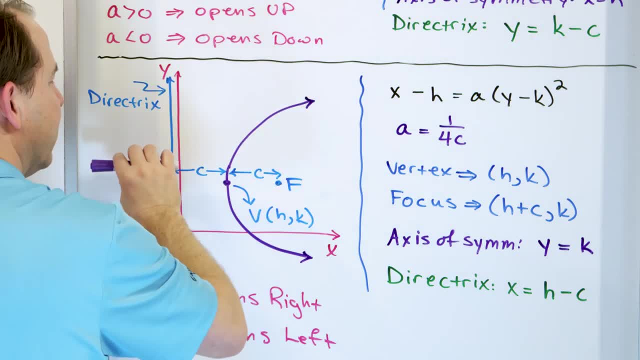 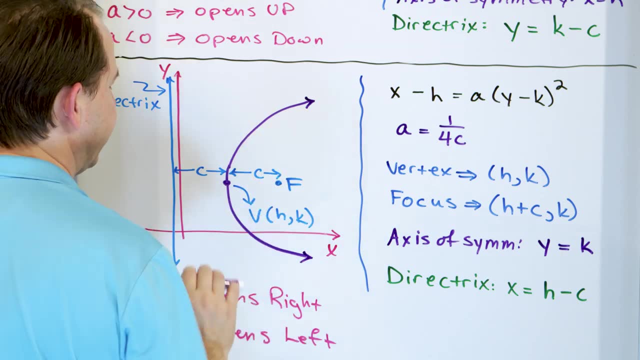 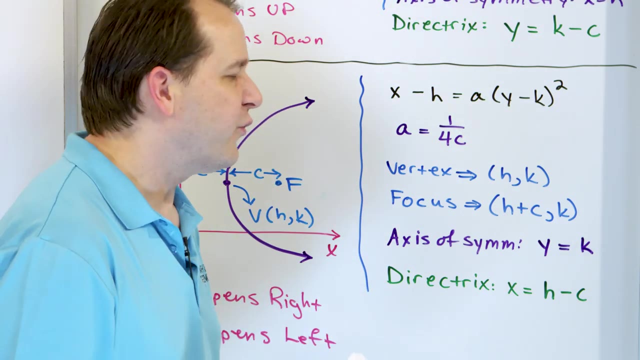 Because it can't be a vertical line, that goes with vertically oriented parabolas. Horizontal parabolas have to have a horizontal line and it goes through the point k. y is equal to k because it goes right through the vertex. And then of course when a is bigger than 0, it opens toward the positive x values. When a is less than 0, it opens toward the negative x values. 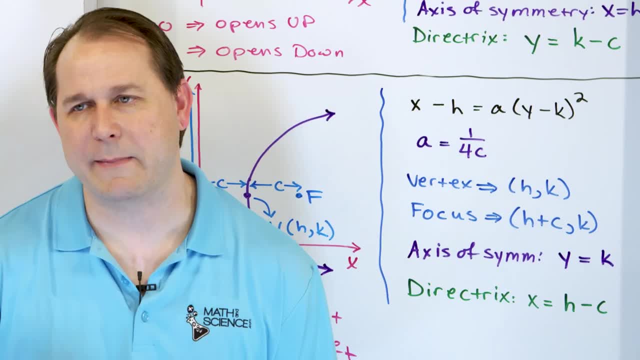 When a is larger than 0, it opens toward the other direction, opposite of that. We have done a tremendous amount in this lesson. 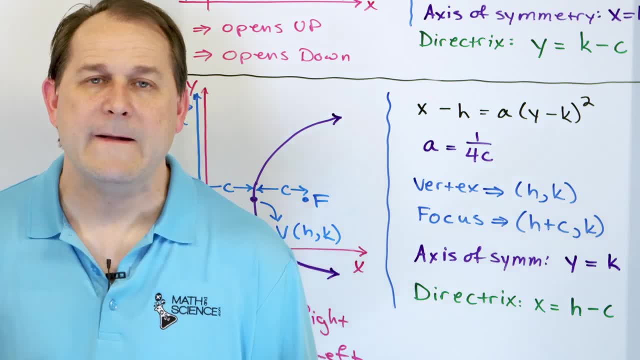 And to be honest with you, I don't like filming lessons this long. But I had to in this case. 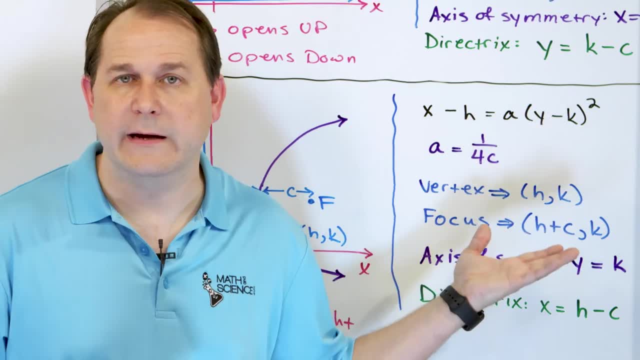 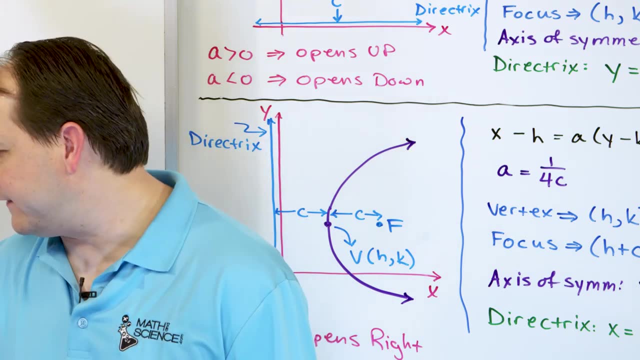 Because if I just give you the equations, you won't understand what to do with them. And if I just derive the shape of the parabola, you won't know how to solve any problems. And if I just review stuff like we did in the beginning, then you'll just review what we've learned and you won't go any farther. 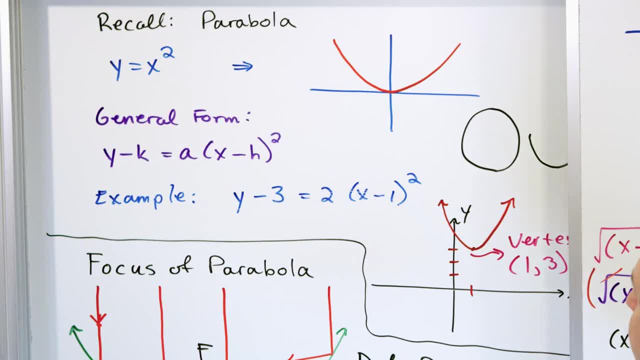 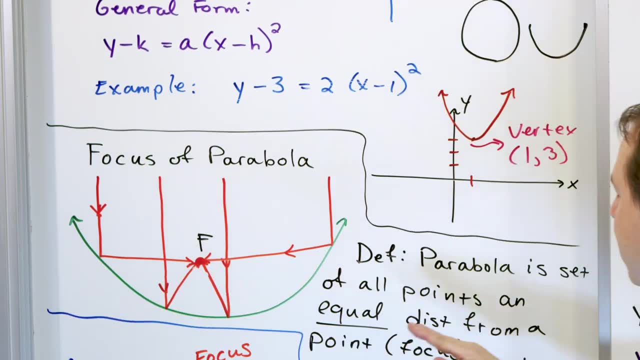 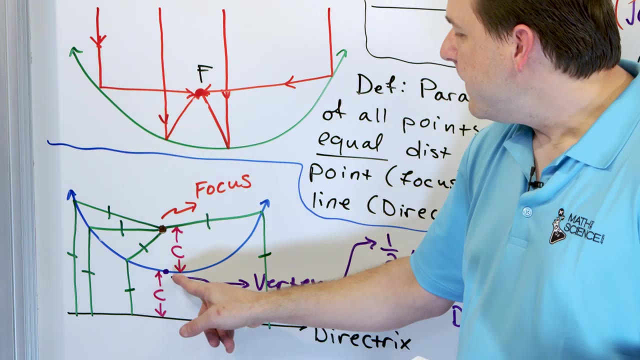 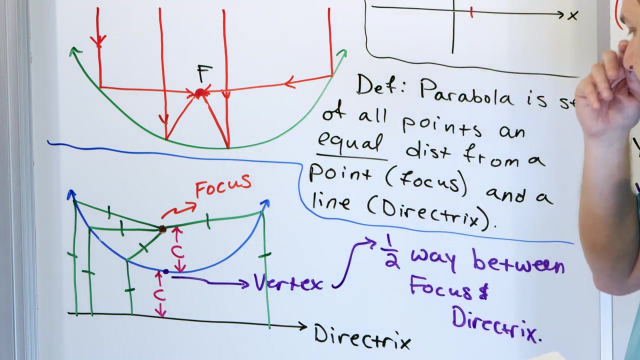 So in this lesson, we have gone from where we have started. We've learned that parabolas have this equation. We knew that. But then we talked about the focus of a parabola. We talked about the definition, being that these points on the parabola are in equal distance to the focus as they are to this line called the directrix. Which by the way, the bottom part of the parabola is always in the middle of the focus and the directrix. Always. That's very useful for you to know. 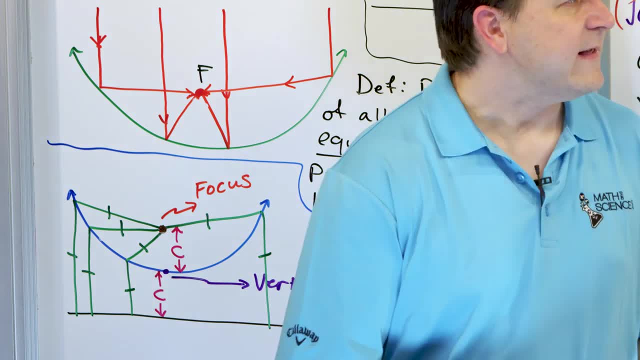 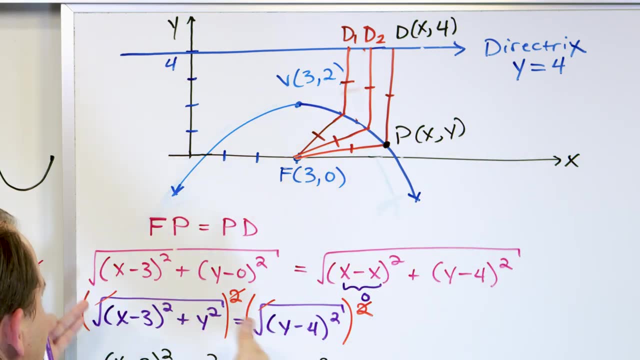 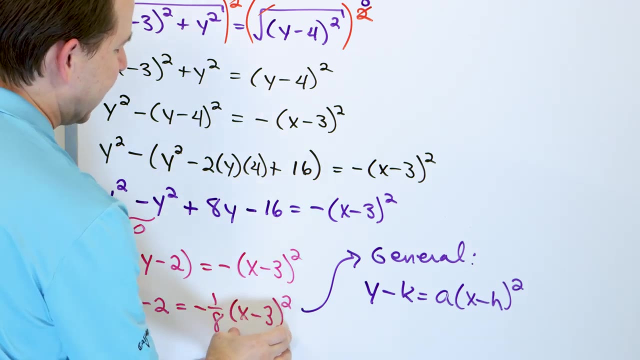 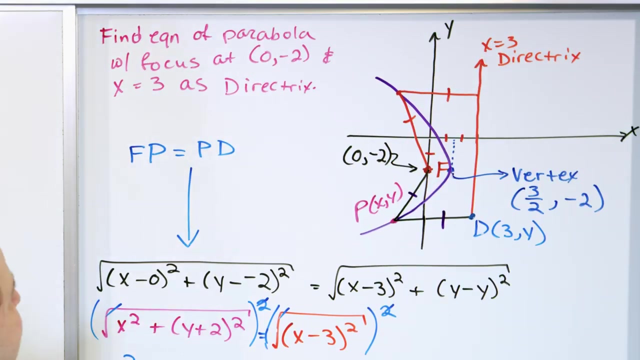 That's the definition. See, it's halfway right there. Then we apply that definition and we say, well if this distance has to be the same as this distance, we'll calculate the distances. We'll set them equal. This is just algebra and you get it down to the equation of the parabola that we have used. y minus some shift on the left, x minus some shift on the right squared. This determines if it opens up or down. Then we do the exact same thing horizontally. We say, let's draw a horizontal parabola. Here's the vertex right in the middle between the focus and the directrix. 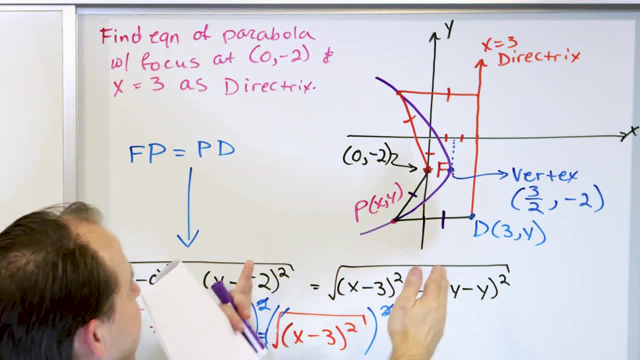 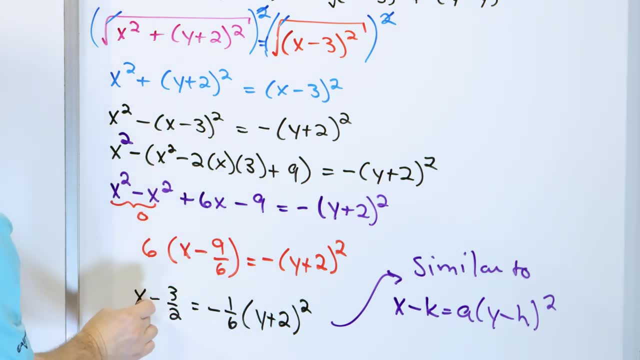 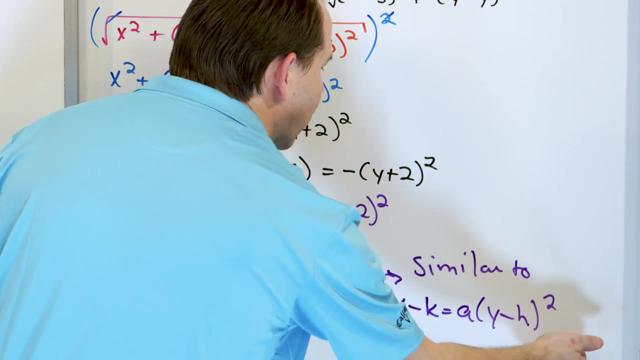 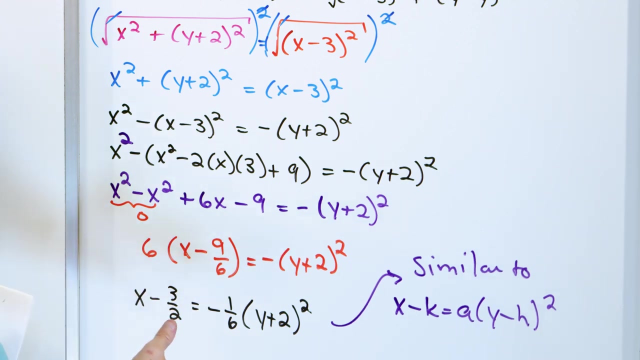 This distance has to be the same as this distance. We'll set this distance equal to the other distance. We'll do all the algebra to get it all down, but what we find is that the rolls of x and y are flipped. It was y on the left and x squared on the right. Now it's x on the left with y squared on the right. So this would be the general form of a horizontal parabola. The shift in y for the vertex goes here. The shift in x for the vertex goes here. Those rules still apply. 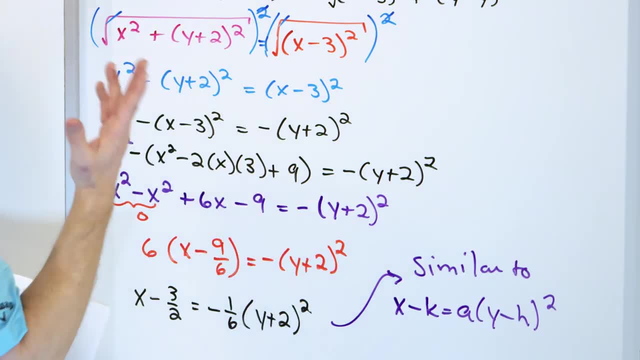 The number in front determines if it opens to the right or to the left, just as you would expect towards positive x or towards negative x. 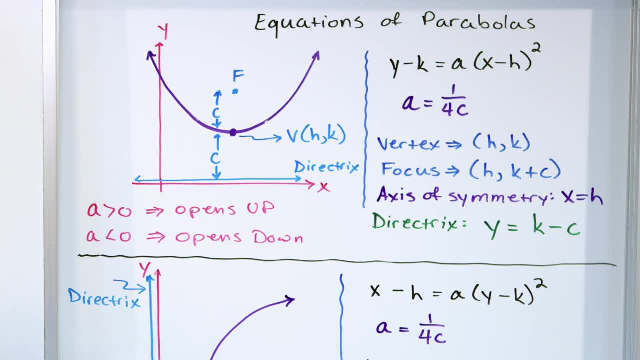 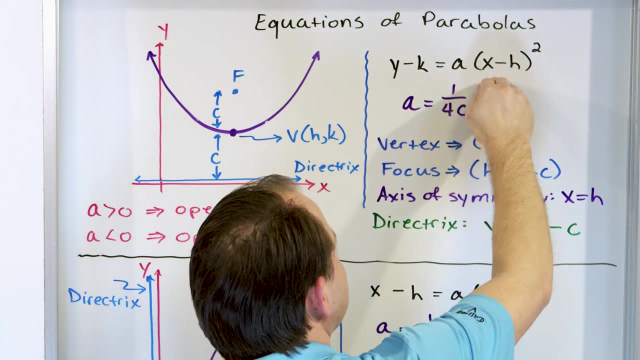 And then finally we have this, which we're going to use for all of our problems. Every parabola has a vertex, a focus, and a directrix. The equation of the parabola is here. The vertex, focus, axis of symmetry, and directrix, we've all talked about them.